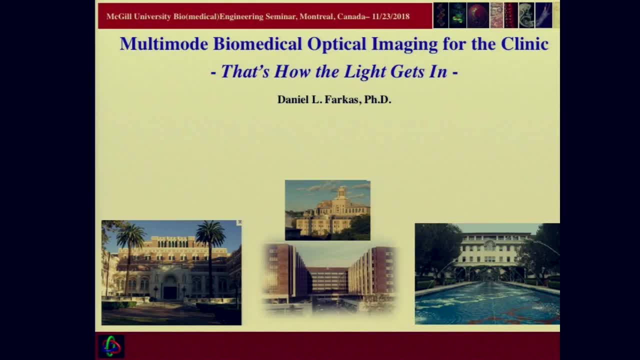 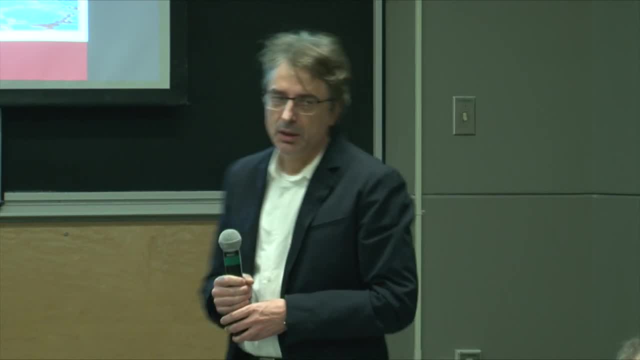 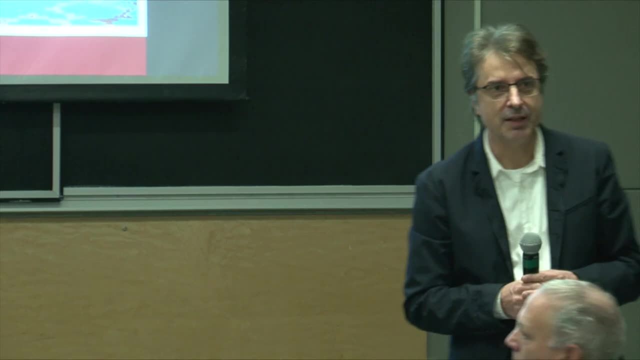 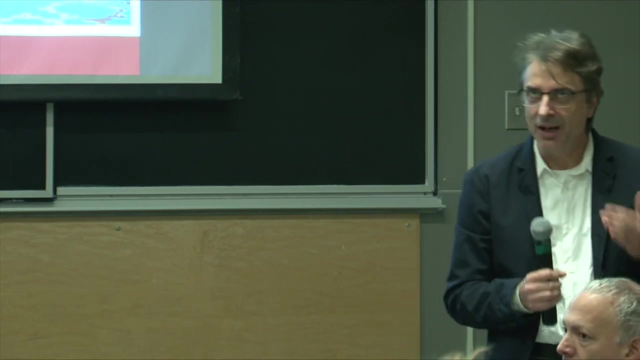 Hello everybody. It is a pleasure to introduce Dr Daniel Farkas. He is coming from Los Angeles and he did his PhD in Israel with a Fulbright scholarship and then he moved to the United States. He spent some time at the University of Connecticut, then some time at the University of Washington, then Carnegie Mellon University, where he was director of a center for light microscopy. 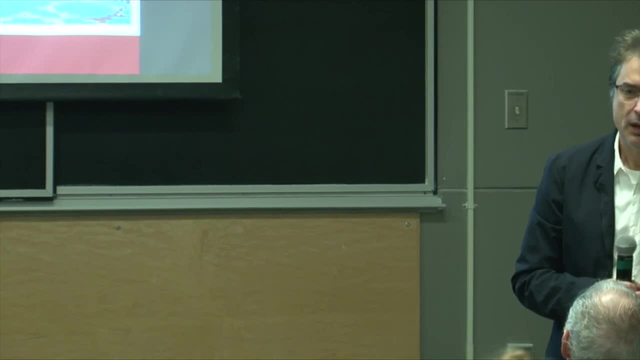 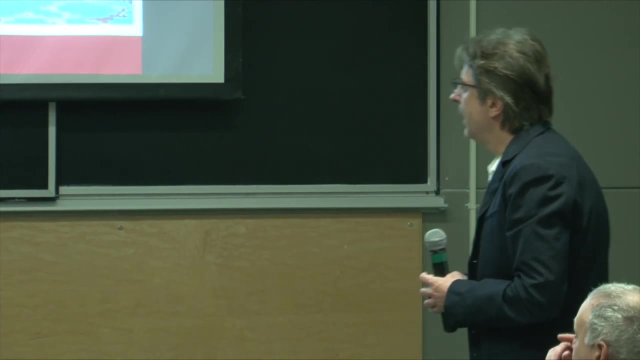 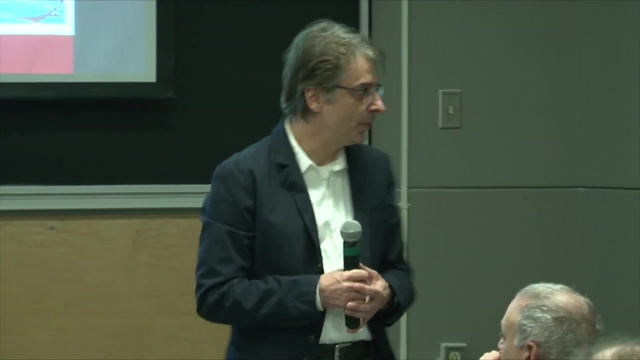 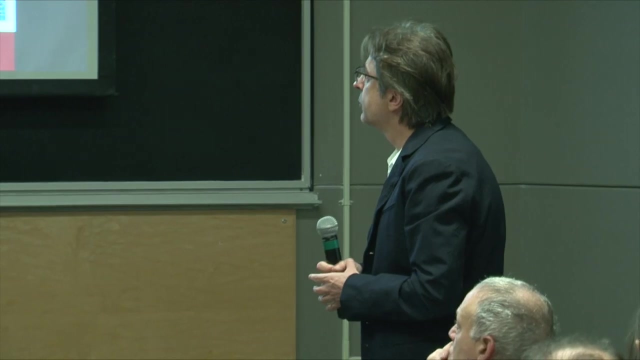 In Pittsburgh, an NSF center. Then he moved to Los Angeles at Cedars-Sinai Medical Center And in the past several years he's been busy with startup companies. He has great experience with starting them and taking them to the next level, So it's a very interesting topic. I don't know if he was going to talk to us about that a little bit. 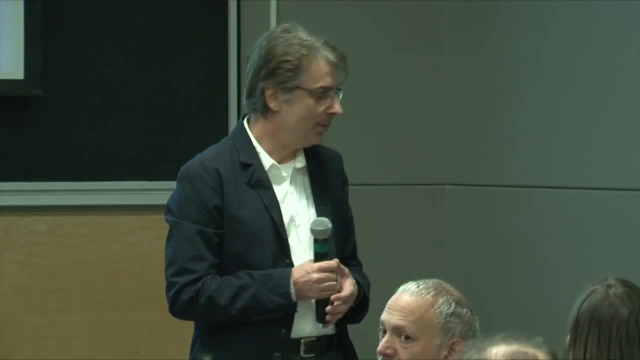 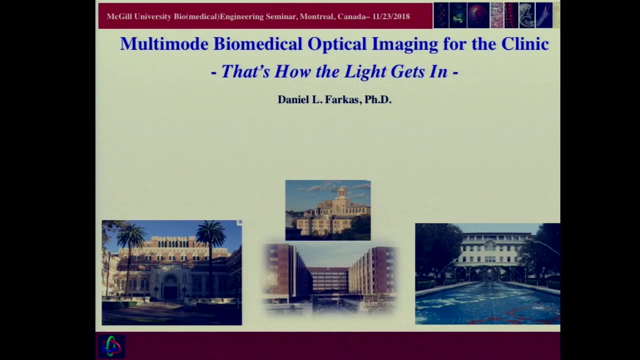 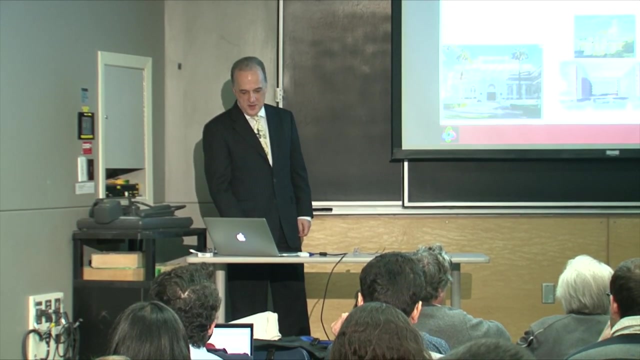 I have great interest in your experience with industry and with startup companies, But today's talk mainly is going to be about multi-modal biomedical optical imaging for the clinic And Daniel, Good afternoon. It's a pleasure and a privilege to be here and I'm grateful for the kind invitation to Professor Waksman-Hodju and Professor Nicolaou. 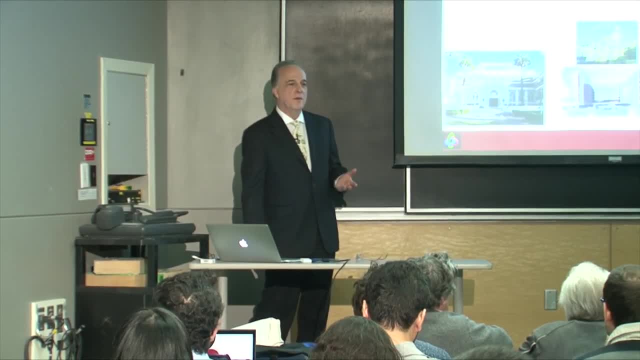 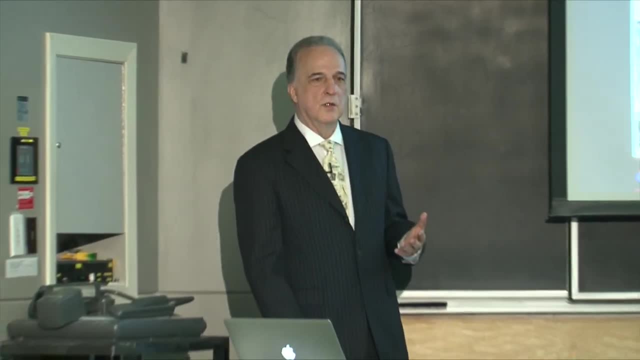 I hope to give you an overview of what we have been doing. I'm very happy to be here and I'm very happy to be working on, And the details are less important than the methodological conclusions and the attempt to get into the clinic and make a difference in people's lives. 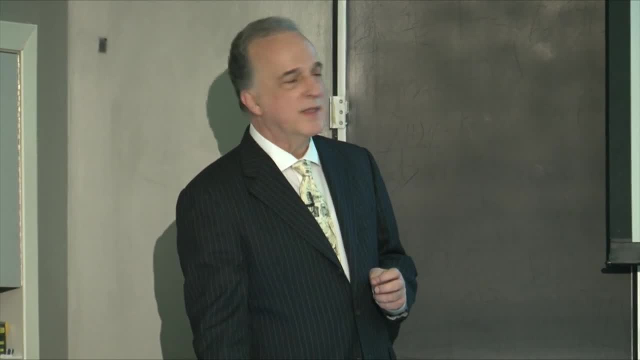 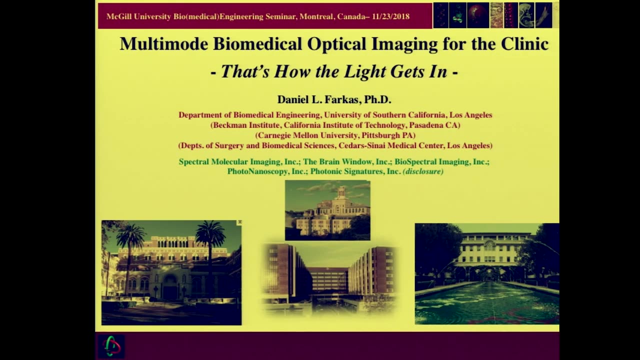 So those are my affiliations. The ones in parenthesis are recent past ones and the green ones obviously are not just companies but also by way of disclosure, And these are pictures of the various places. I shall explain the title and I don't think I have to explain the subtitle. 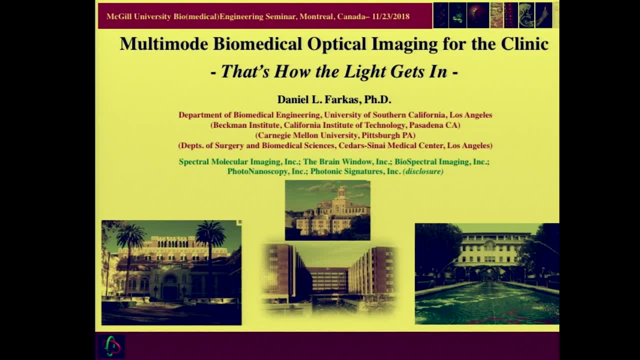 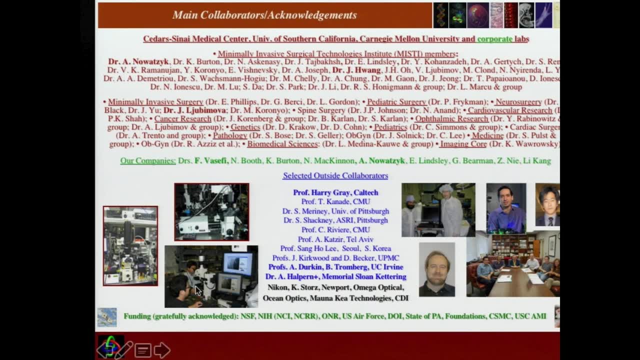 It's just an homage to one of your most famous alumni, Leonard Cohen, But I do want to talk about how the light gets in. So I usually get in time trouble towards the end of my talk. So I always put the acknowledgments up front, and the people particularly emboldened characters are the ones whose work I'm going to highlight. 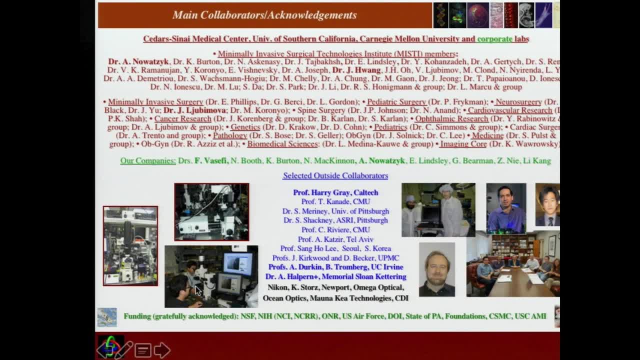 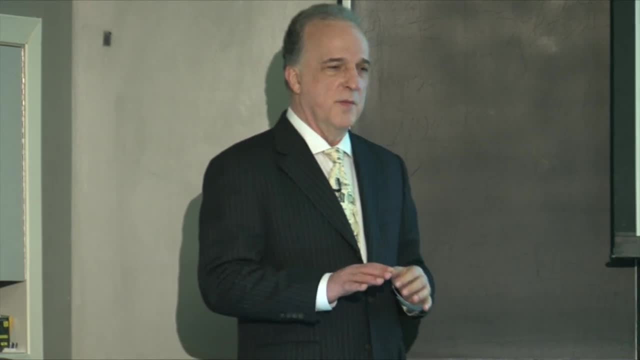 And especially Dr Vasefi here, Dr Novacek And Dr Huang, And we have a lot of collaborators, So my slides are kind of busy and think of them as baroque or think of them as being the top of a stack of slides. 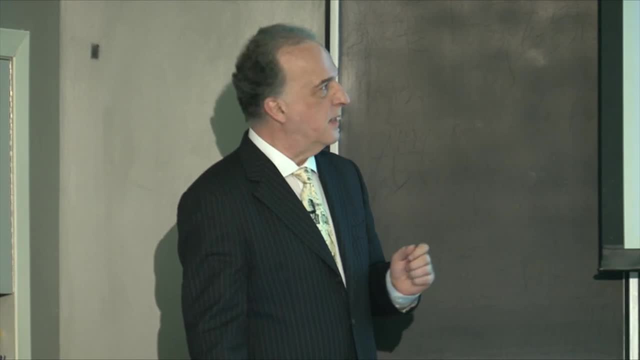 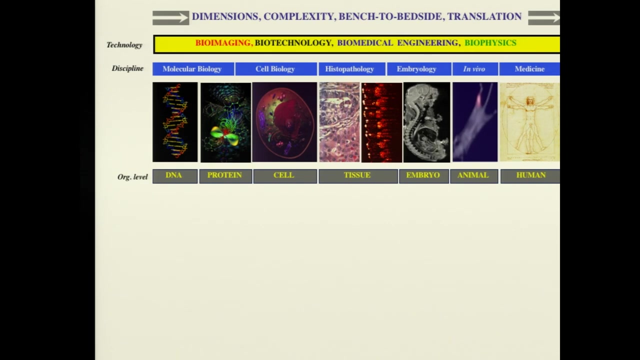 But hopefully they will convey a relatively simple idea each of them. This one is to illustrate what we think about as translational work. So the idea is that as you go from laboratory based findings towards the clinic, you try to extract the most interesting conclusions, lessons and applications and put them to use in the clinic. 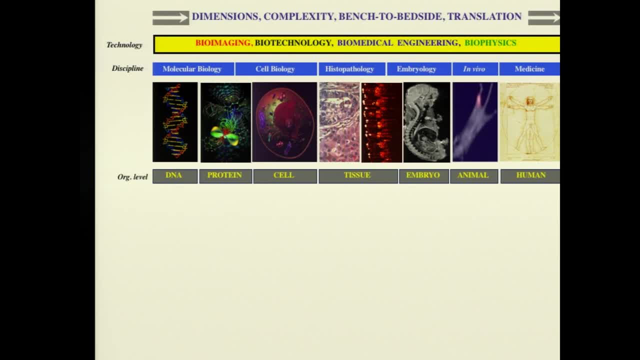 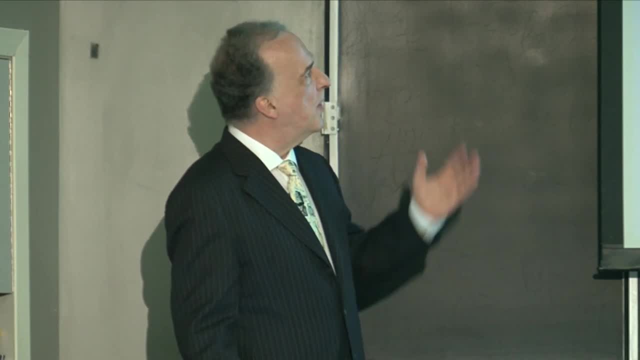 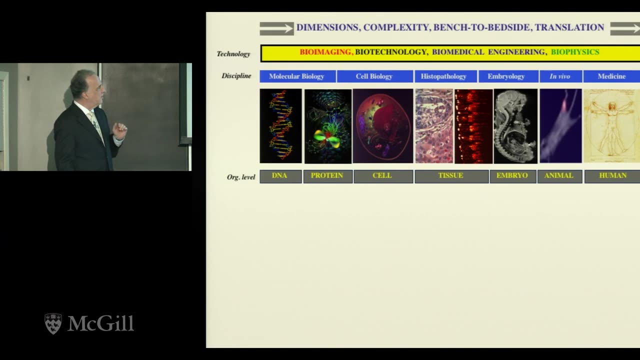 And we all know that this is desirable, and we also know that it's not working quite as well and certainly not quite as efficiently as it should. So, therefore, it raises the question: why is that So? as you go here from left to right, you see the disciplines involved, you see the organizational levels, all the way from molecules to living humans. 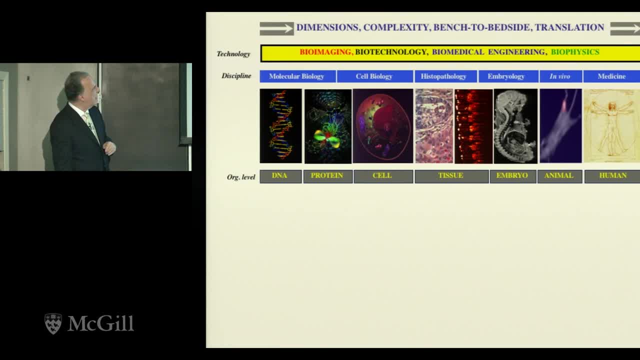 And On the bottom, the organizational levels, And then there's also obviously an informatics component to this, And so you see genomics, proteomics, all very much on the rise. But last I looked, the most important omics is still economics. 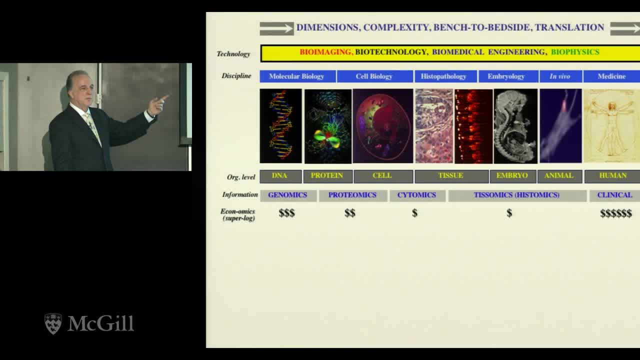 And the dollar signs on the bottom are severely super logarithmic representation of what the money is. And so the couple of dollar signs at the end there in the clinic, those are trillions of dollars we are talking about And the in-between space is really not that much. 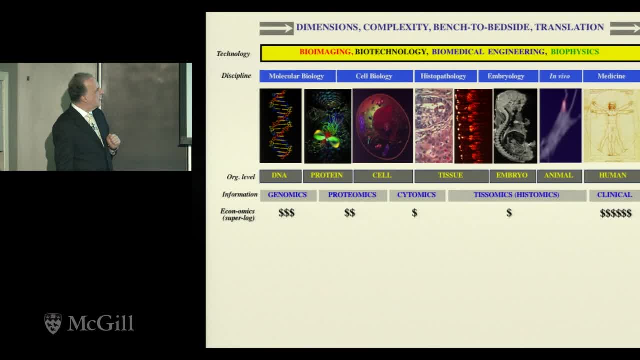 This is really not that particularly well covered, And this becomes even more obvious if you look at what the research is mostly, what the clinical need is mostly and also what the diagnosis is. So, on the current practice, at best you extract a piece of tissue from the patient and you bring it to the middle to diagnose it by, let's say, histopathology, very much like you could do 100 years ago. 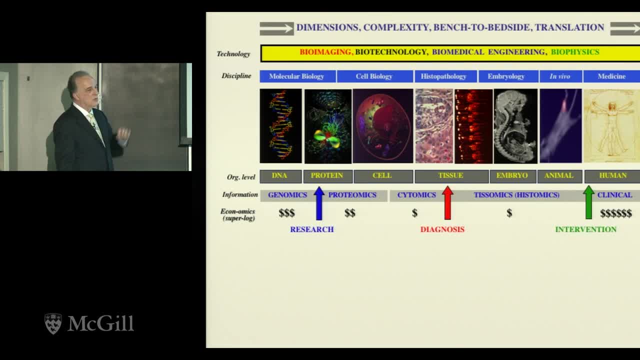 And if that doesn't give a clear answer, then maybe you look for molecular markers and so forth. That is probably not the most efficient way to do it. So ideally you would like to overlap these arrows, but not overlap them on the research side, but overlap them on the clinical side. 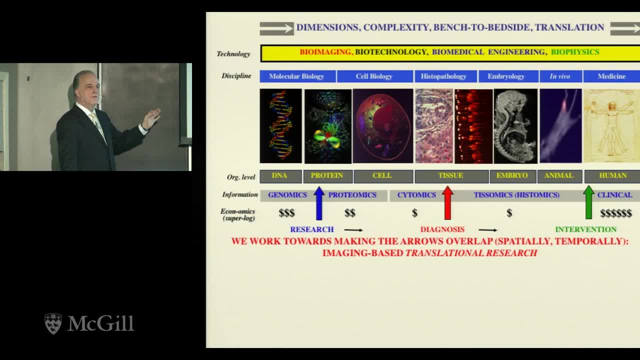 Like that, And so we are mostly working on overlapping these arrows on the clinical side, in the sense that you could do molecular and cellular level work in the living body of a patient, And if you think that that's a nice thing to do, Yeah. 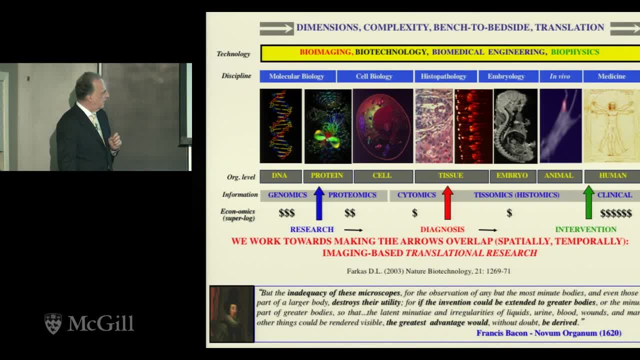 Novel idea. Here's Francis Bacon, no less that you know, 400 years ago or so, not having seen a microscope, he just says: basically microscopes are great, but what would be really great is to have microscopic resolution in the body. 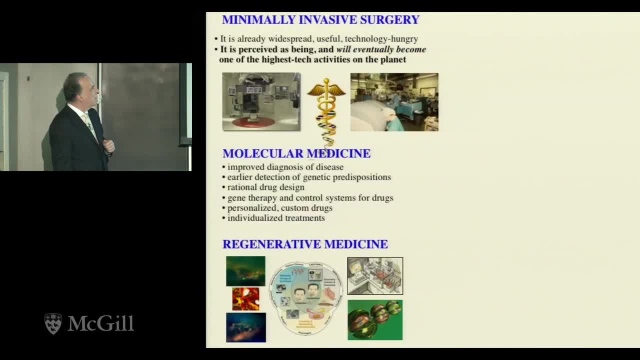 Then you can really say something. So let's look at what I think is going to be kind of the foreseeable future of modern medicine for the, let's say, the next 50 years: Minimally invasive surgery, molecular medicine and regenerative medicine. 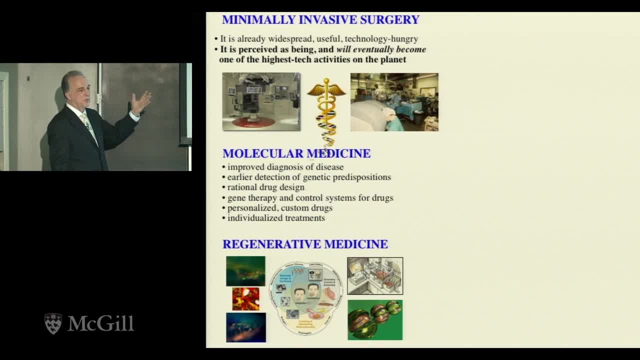 Minimally invasive surgery and endoscopy, basically, is taking over from regular surgery, And you would assume that it's one of the most sophisticated undertakings on the planet, but I'm here to tell you that it's not. But it could be. 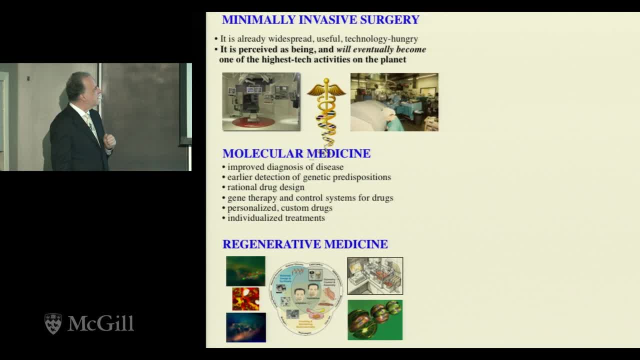 Molecular medicine is also very exciting: Improved diagnosis, rational drug design, gene therapies and personalized custom drugs Of course it's very worthwhile to have. And regenerative medicine possibly even more exciting, because not only can you in principle fix things, you can actually make them better than they ever were if you do things right. 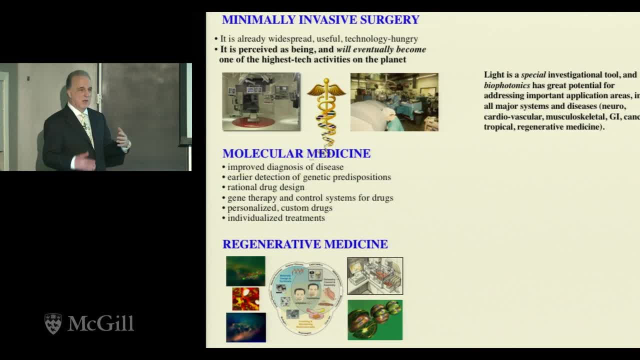 So now, the main point I would like to make, through multiple illustrations at various levels of biological organization, is that light is a very powerful investigational tool and in certain ways, it's still underutilized, especially as advanced optical imaging is still very underutilized. 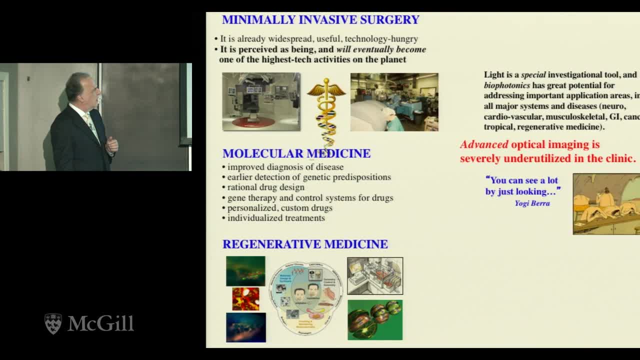 And why that is. You can look at it this way that, as Yogi Berra said, you can see a lot by just looking. So a lot of modern medicine still uses this very, very subjective, human, limited ways of looking, whether it's histopathology or, in the dermatology field, looking at very serious potential things like melanoma. 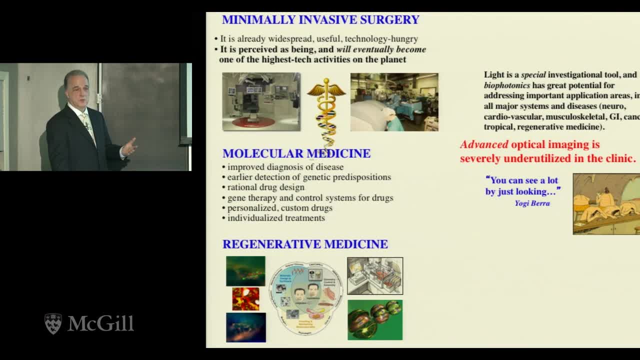 We still look at them and treat them the same way as we could have done in the Roman Empire. basically, Look at it, see it being ugly and cut it out. That shouldn't be like that, And let's see what we can do about it. 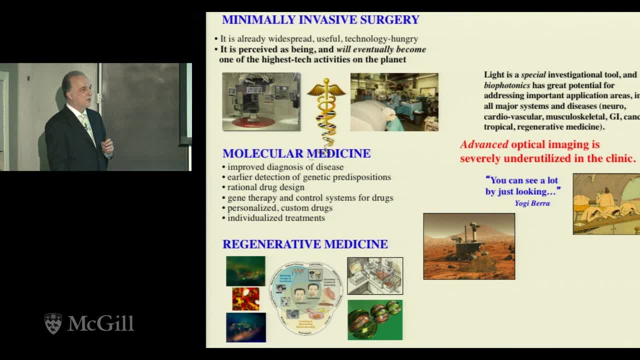 Some of you might recognize this picture. It's the Mars rover, And the reason I'm showing it is that today we can image dust on Mars significantly better in terms of pixel resolution, spatial resolution, discrimination ability and so forth- better than we can image inside the human being in serious trouble in one of our best hospitals. 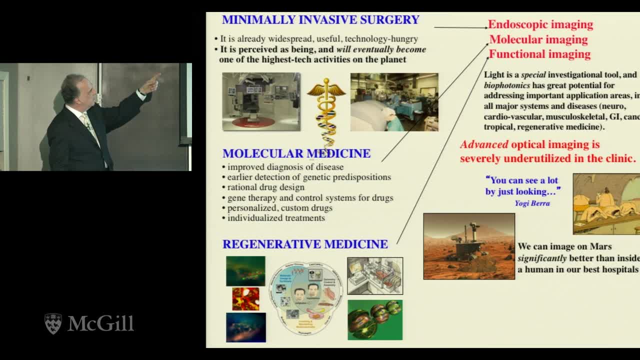 So if you take these three fields and map them onto the type of imaging that is needed- endoscopic models- you can see that. So if you take these three fields and map them onto the type of imaging that is needed- endoscopic, molecular and functional- there's no reason why they cannot be one and the same. 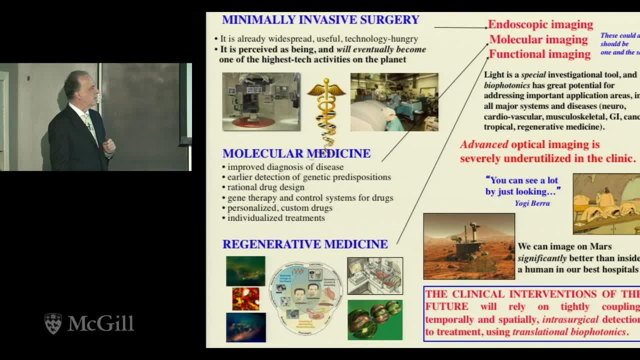 And that would allow you to engage in modern clinical intervention in which you're coupling temporally and spatially much more tightly- diagnosis, advanced diagnosis based on advanced optical imaging and intervention, And so I would like to illustrate a few of these things in applications that we have tackled through the years. 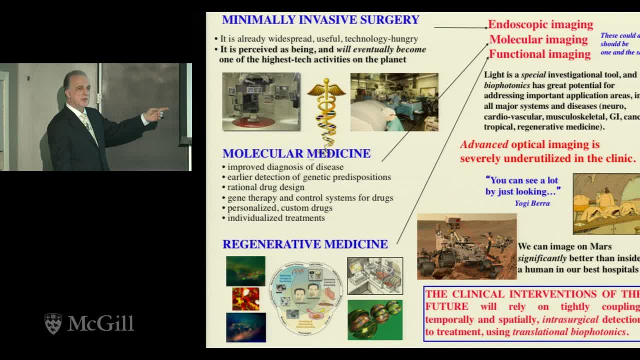 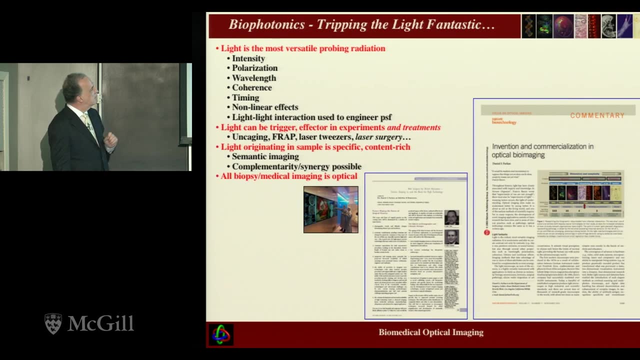 By the way, that was the old Mars rover. The new Mars rover has something like 26 cameras and lasers that pulverize rock, and so on. So, as technologists, this should give us pause that we are falling behind Quickly about biophotonics. 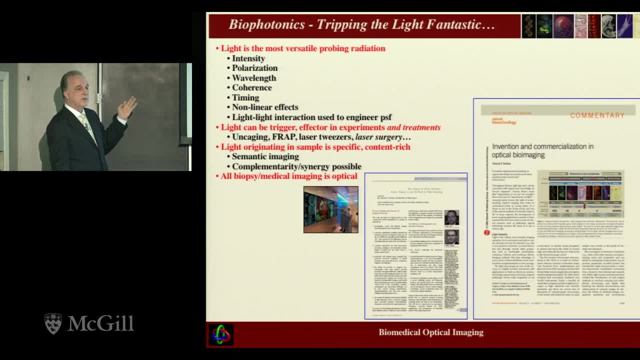 So light is a very versatile probing radiation. It has multiple ways in which it can create contrast. There's no reason that you cannot combine those different ways- And it can also be a trigger and defector in clinical experiments. It's originating in the sample as a very kind of semantic level signal. 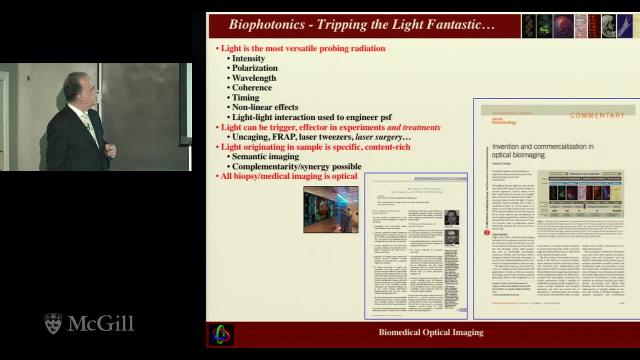 And ultimately all biopsy and medical imaging is partially optical, because when you're looking at your MRIs and PET scans and so forth, somebody still has to look with the eye and determine what that all means, And so somebody we have to worry about the three R's resolution, relevance and realism. 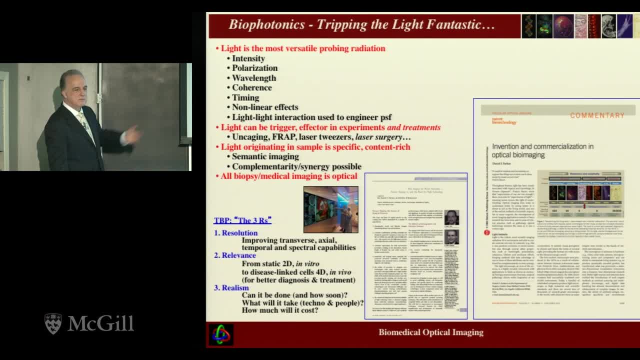 And realism. of course, can something new be done while we are still alive. So we can't do it all around. So Dr Galloway is telling us that you need a pile of sophisticated high technology to map the molecular inhabitants of the cells. 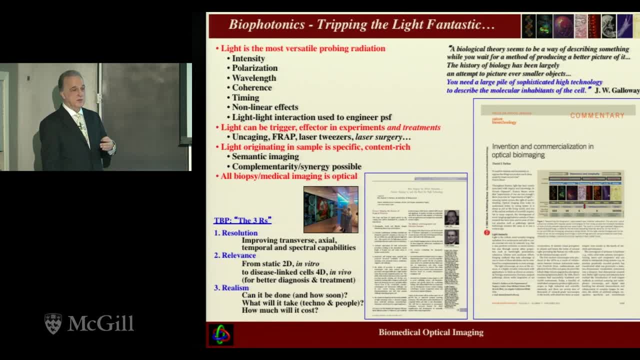 So, remember, we would like to map these molecular inhabitants in the body. So you need much more than you need just for the cells, and preferably not in the configuration of a pile, in something a little bit more strategic, And I'm going to talk about the strategy part of this. 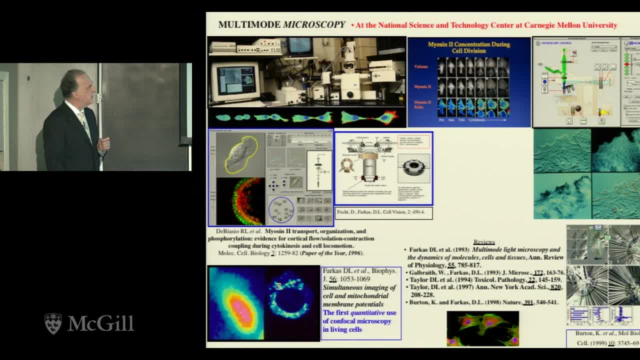 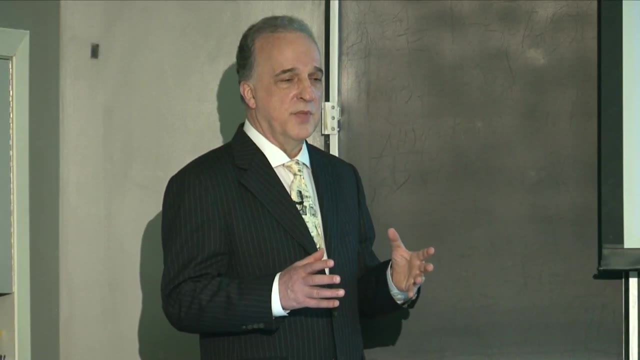 So let's start with the center that Sebastian mentioned. So I had the singular good fortune of leading this national science and technology that encompassed nine departments at Carnegie Mellon in the 90s, And what we developed was an approach to microscopy in which you roboticized the microscope and allowed it to look at the cells that were still kept cozy and thinking that they are still in the body and engaging in cellular type activities, such as wound healing and cellular division and so forth. 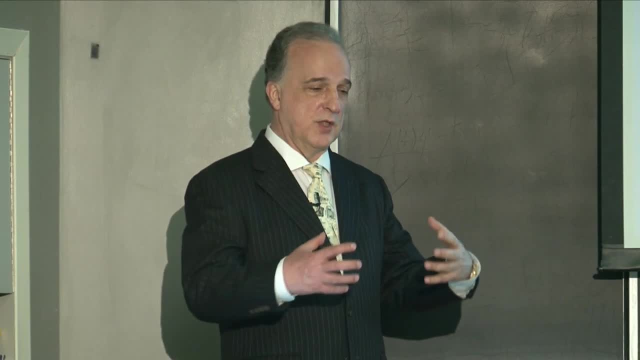 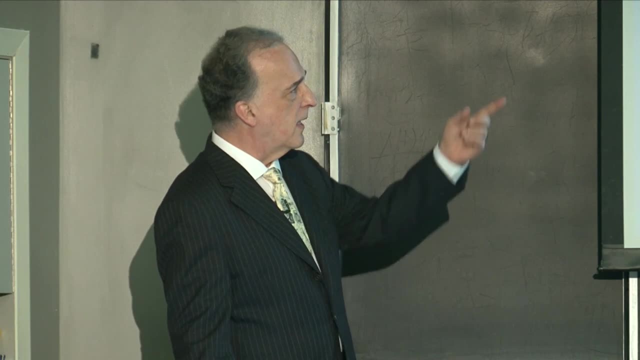 But look at them in four, five, six different ways so that you capture as much as possible of the essence of what is happening, And we published quite extensively on this. We were able to look at things like nano-Newton level forces involved in cell division. 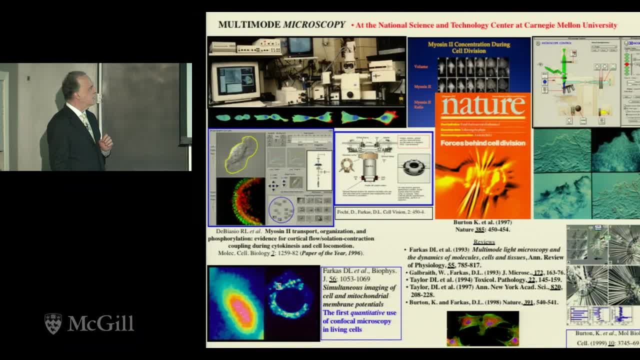 This is beautiful work by Kevin Burton, who is still with us after all these years, And we used the confocal first to do dynamic and quantitative things, And so all in all it was very rewarding for molecular, cellular and developmental biology. But it became clear that we would like to first accelerate the process. 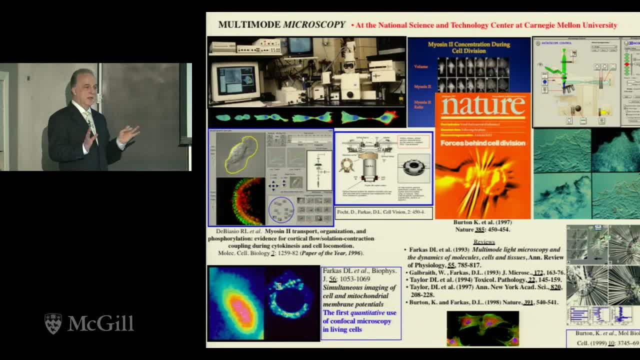 But it became clear that we would like to first accelerate the process. But it became clear that we would like to first accelerate the process, Then extend the tools that we are using in all possible directions. that made sense And I'm going to talk a little bit about that in the next couple of slides. 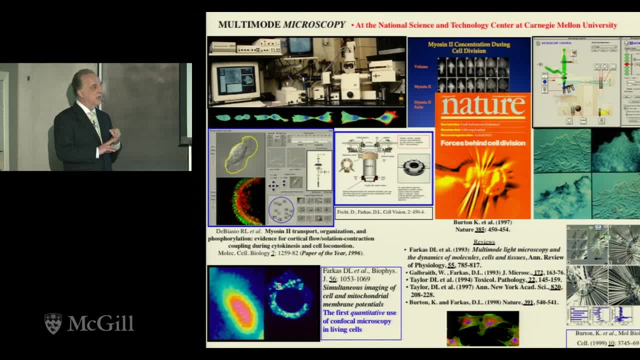 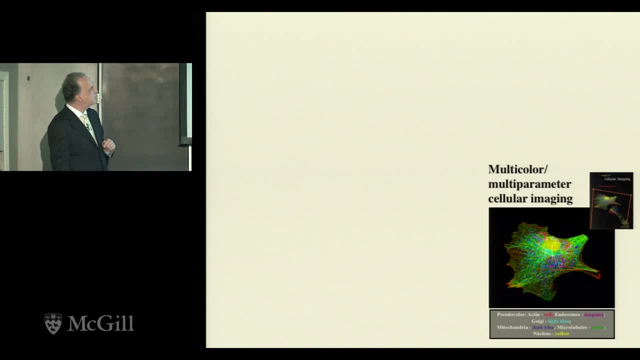 And then take all of that was learned and try to apply it to actually bettering the human condition by bringing it to the clinic. One thing you can do is you can start looking at the cellular components and see what they contribute to various cellular activities. for that you need to separate them by. 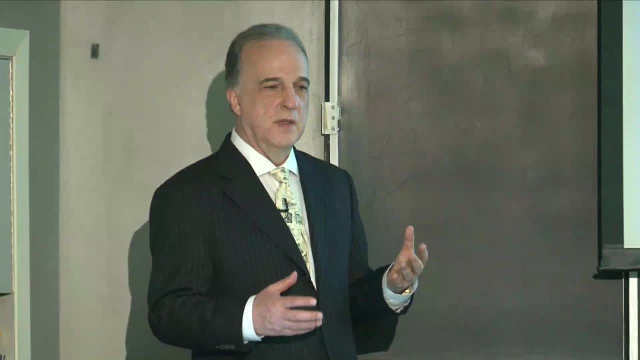 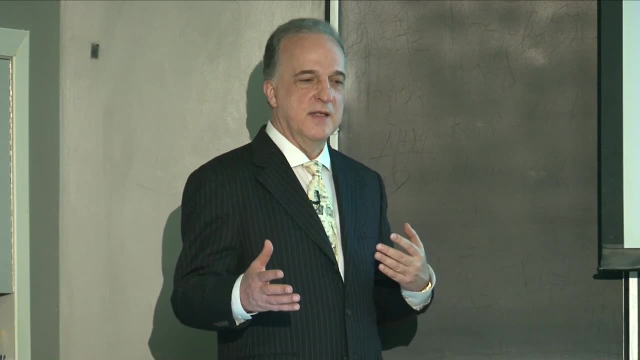 let's call it color. but by wavelengths And at some point regular microscopy, lassen pipes will become more efficient. regular microscopy allows you to look, maybe, at three, four sinks, but by the time you want to get greedy and look at six, seven, eight sinks, you need something different. 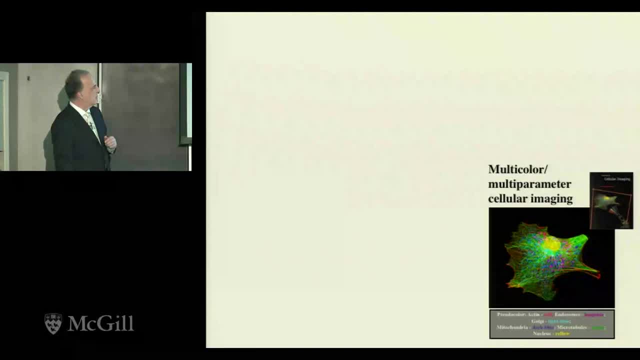 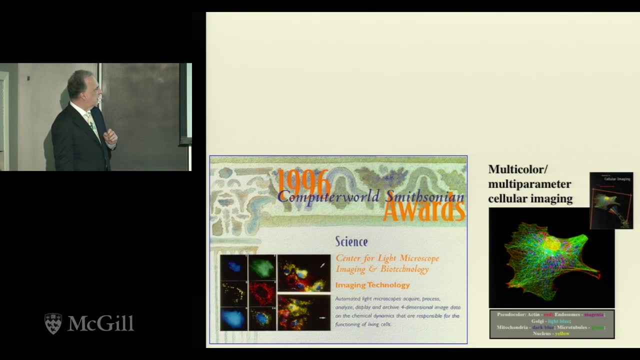 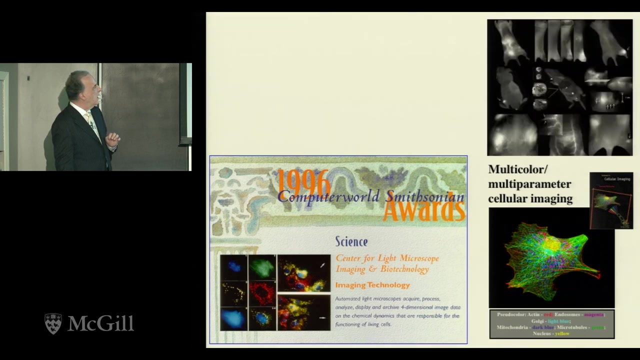 which we took it to be hyperspectral imaging. This was actually very well regarded by both reviewers of papers and by the Smithsonian people. At this point we were able to look at five different cellular components in cells that were engaging in wound healing. Another direction is obviously to go into preclinical. 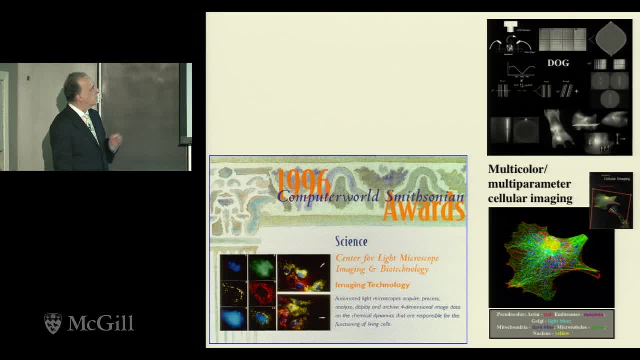 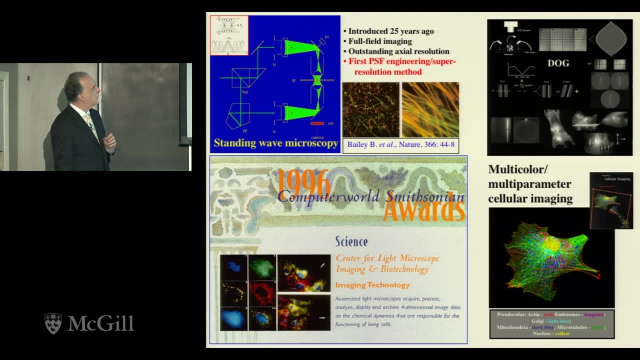 models and eventually clinical. and we developed a 3D method that we called- because they're already CAT scans and PET scans- we called it DOC scans- Digital Optical Goniometry. And finally, we tried to improve on microscopy. The microscope is an icon of the sciences, but its resolution is limited. 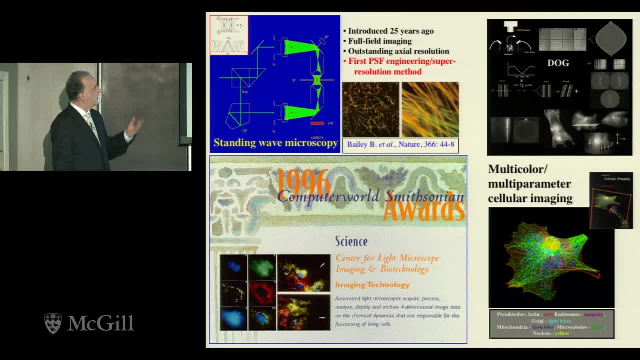 by very well-understood, well-defined physics. So therefore, this was early on. there were no super-resolution methods at the time, and it was becoming clear that you need to manipulate the point spread function in order to get the additional resolution that you would ideally. 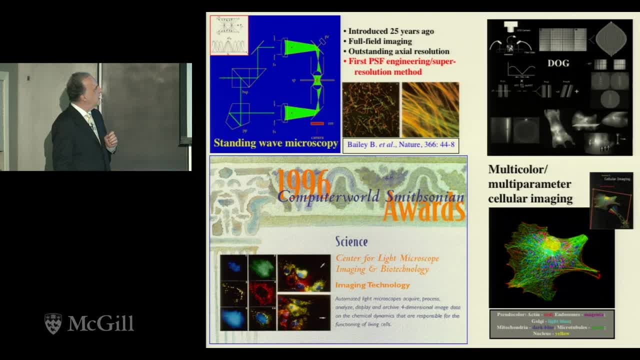 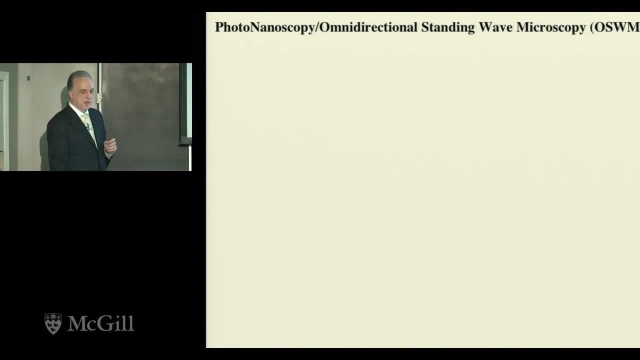 want out of your microscope. So we introduced the first of these methods. It was published twenty-five years ago and it allowed us to enhance the axial resolution of microscopy by almost two orders of magnitude. So there has been, in our lab, recent follow-up on 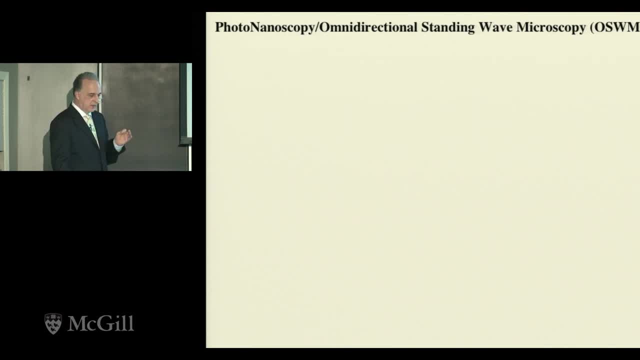 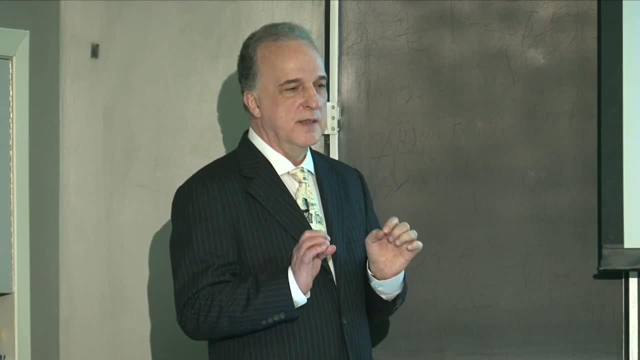 this, so I am going to describe that very quickly. So the way that you can get around the physics that governs the resolution in microscopy is to basically put the light only in certain places, and this can be done in multiple different ways. as I said, engineering. 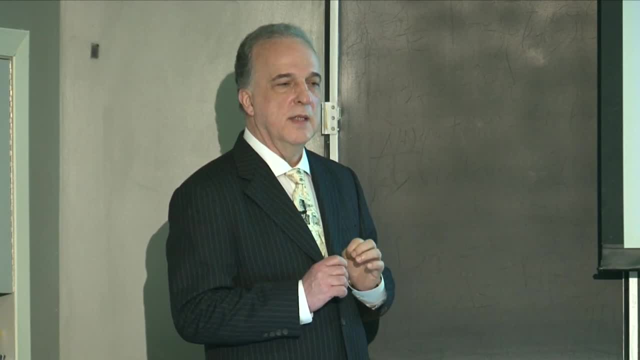 the point spread function, and the one way that we did is that you take the light that is illuminating the sample and split it between two lines, and the point spread function, as I said, is a point spread function, and the one way that we did is that you take the 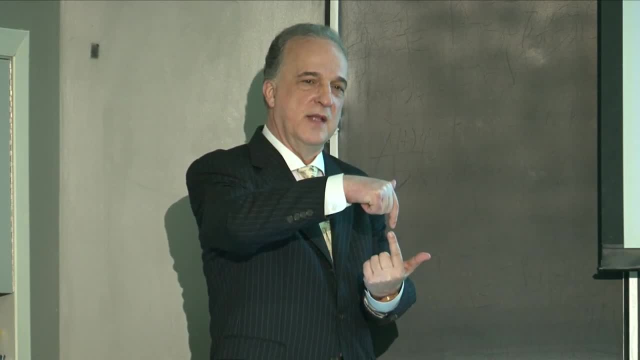 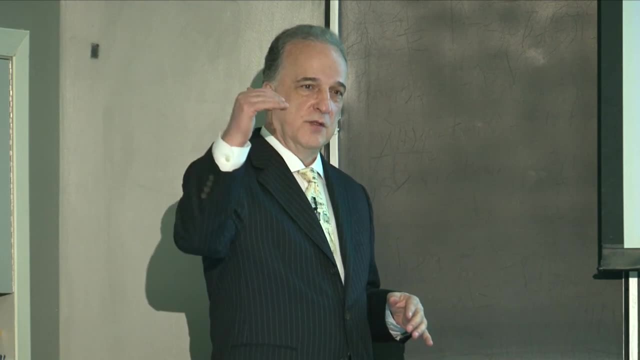 it- it's a laser light- and make it interfere with itself at the specimen, which creates fringes, vertical fringes of interference, and you can move those fringes by just changing the phase of the interferometer. So with that you can move the fringes. if you think about, 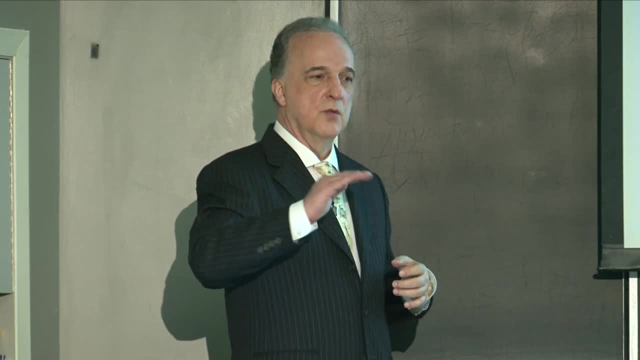 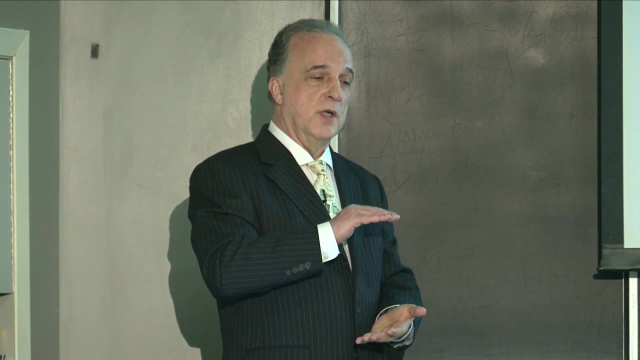 the focal position of the microscope as the coarse rulings on the ruler. you can introduce the fine rulings just by changing the phase of that interferometric set of fringes. So it turns out that you can go from typically one micron resolution in the axial domain. 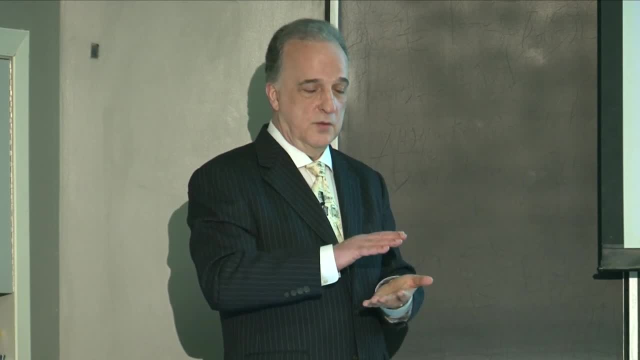 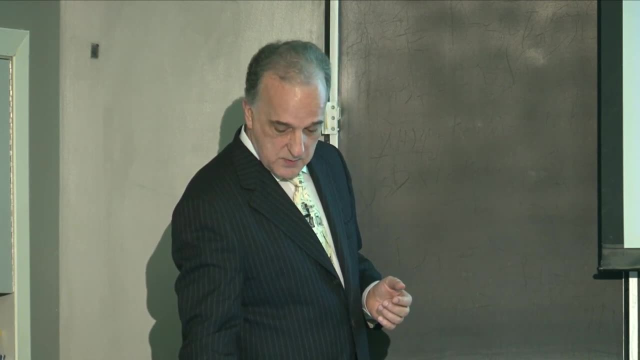 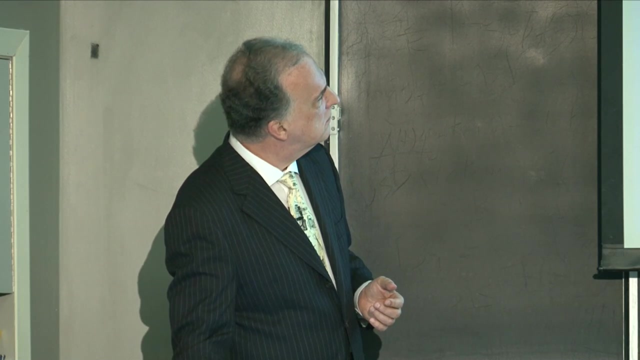 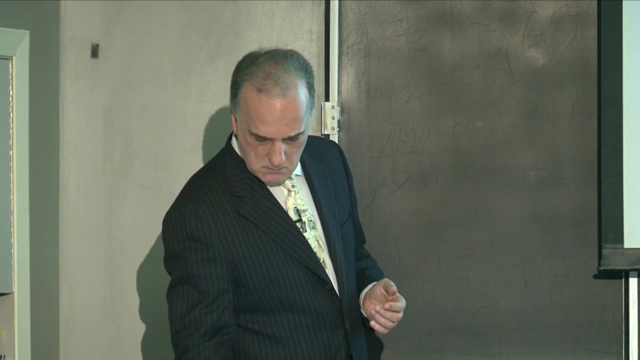 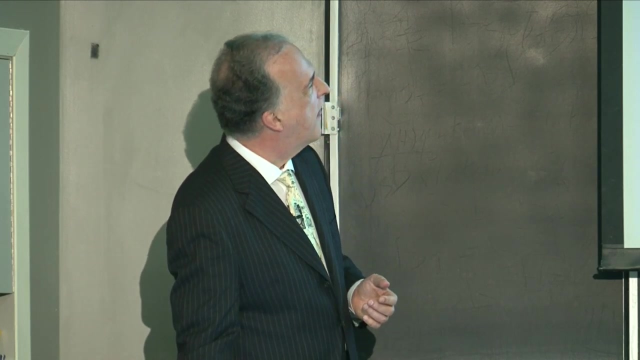 which you get in normal microscopy, or half a micron in confocal and two photon. you can go all the way down to a couple of nanometers in resolution by just moving those fringes, And we did that. I'm not sure why this. That's what it does, Okay, So we developed this method that we 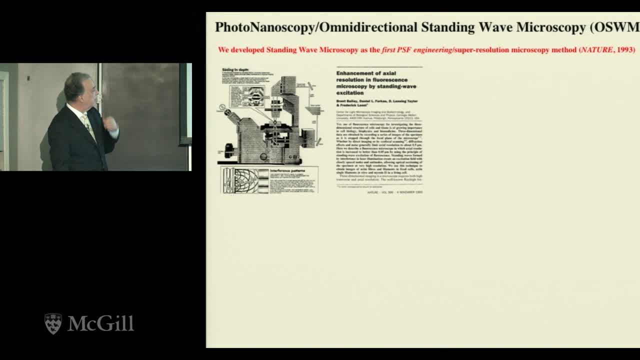 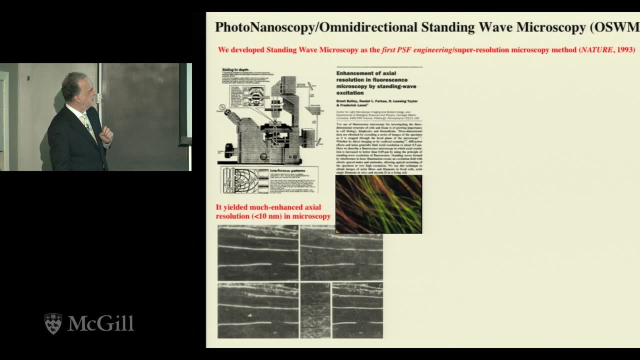 call standing wave microscopy because the fringe pattern is a standing wave pattern and we were able to get, for instance, the two sets of delicate fibers in the cell. actin fibers are separated by 35 nanometers here and they are very easy to see separately. 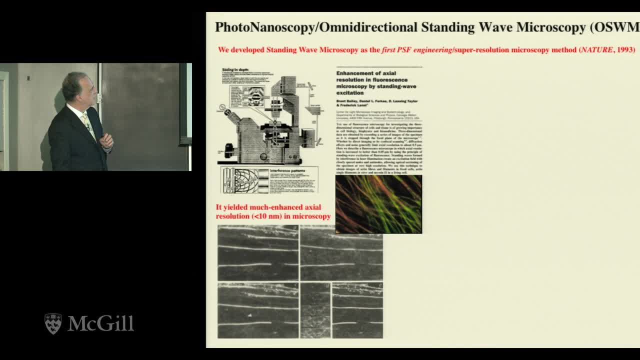 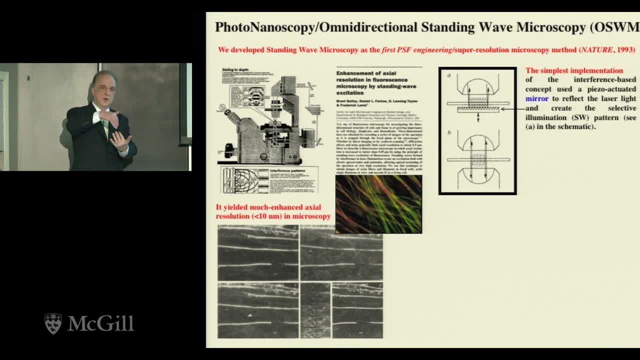 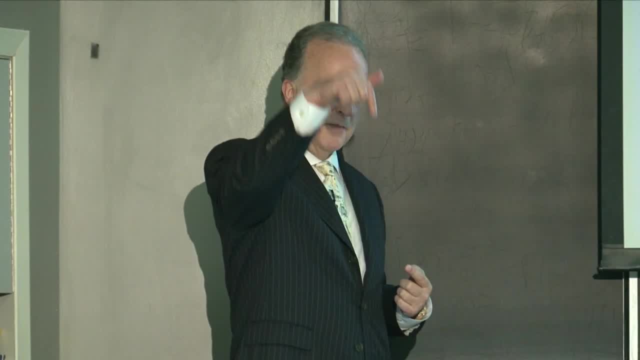 this is not even to take the laser beam and set and separate it and interfere with the cell, but rather take a single laser beam go, have it go through the specimen, put a mirror on top of the specimen, have it hit the mirror and come back on itself, which? 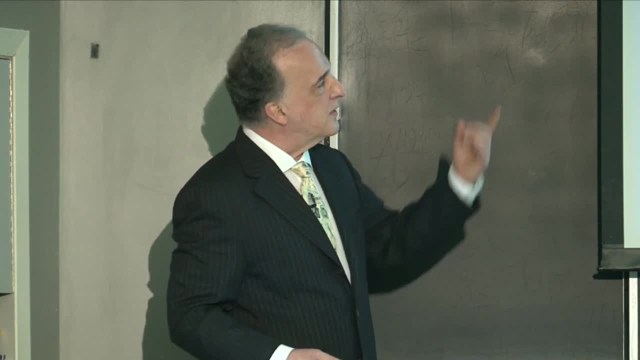 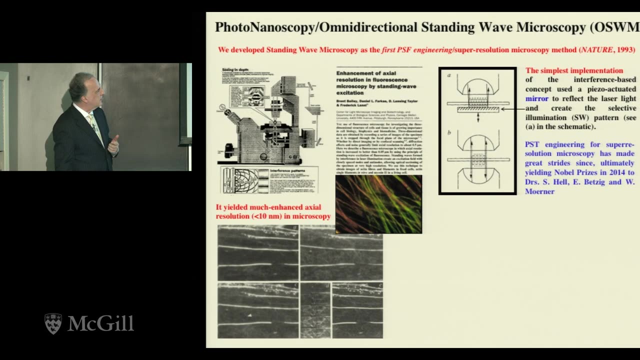 introduces this interference fringes in standing wave, And so that was the cheapest, simplest implementation of standing wave. But subsequently it gave Dr Andreas Nowacheck in our labs an idea that maybe this can be moved into all three dimensions, And we were trying to do it at the time. 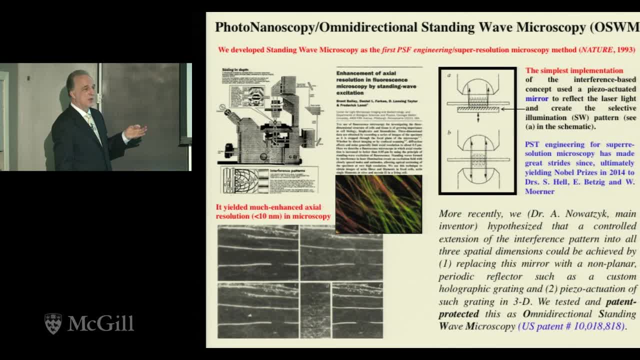 but it turns out that the computational power was really not available even from a Cray supercomputer at the time. By the way, in the meantime, of course, the field of super-resolution microscopy has evolved tremendously and extraordinarily smart and beautiful things have been done, culminating. 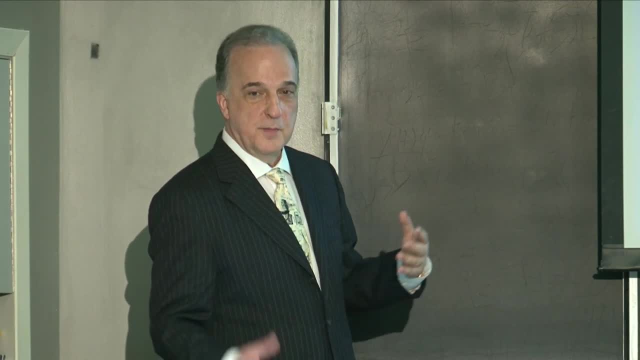 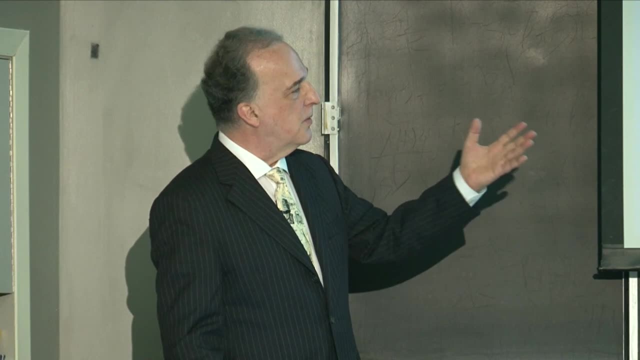 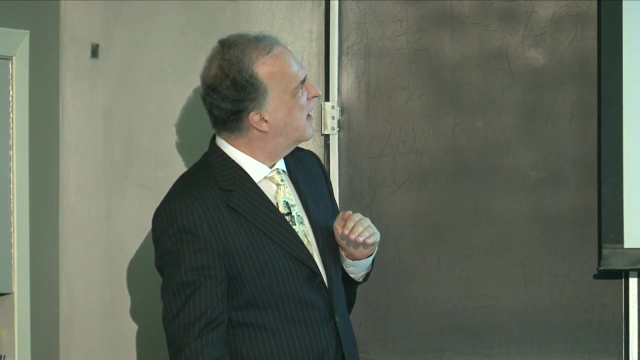 in three of our colleagues getting Nobel Prizes for their particular approach, which is very nice physics. We were looking for something a little bit more practical and simple, and so Dr Novacek proposed that instead of that mirror, if you can put in a holographic. 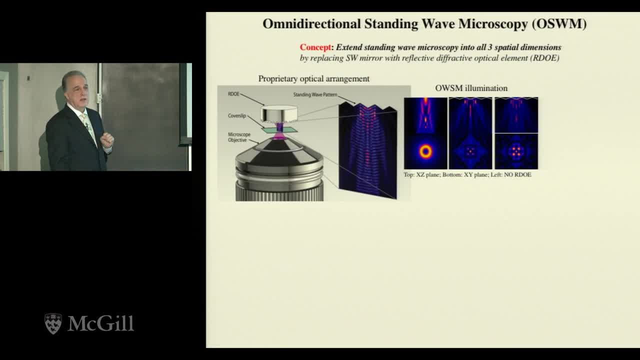 grating, ideally a custom holographic grating- then the fringes would not just go in one direction, but they would go in all directions, and then you would just move that grating and you would be able to cover all three-dimensional space. 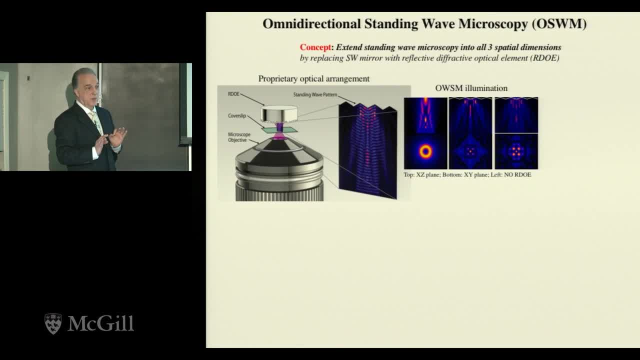 with very delicately Structured, spatially structured light. The problem is that of course you have to put then the 3-D picture back together so you do have super-resolution, but how do you know what's where? And so 25 years ago that was not possible. 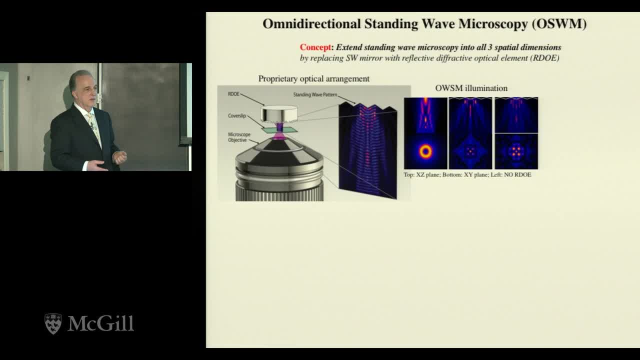 Today you can just buy some graphics processors and put them in your computer and have much more than the equivalent of a supercomputer in 1993.. So we are developing this method. This is the schematic. I'm not going to dwell too much because I have a whole lot more. 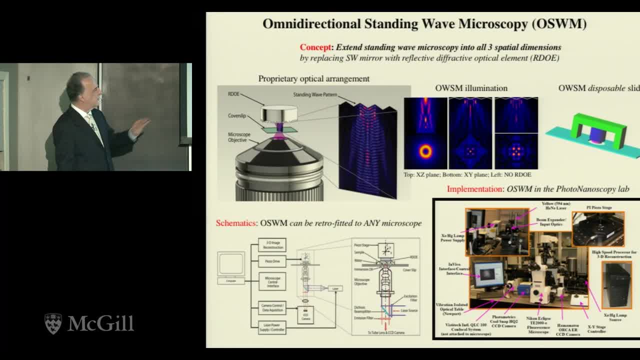 to tell you about, but just to close the void of the microscopy part of this talk. we are starting to apply this and plan to apply this to some very, very specific, clinically relevant things, including a very exciting joint project with Professor Waxman-Hodjo here. 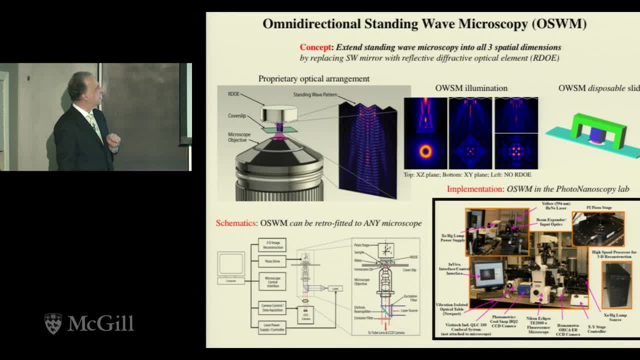 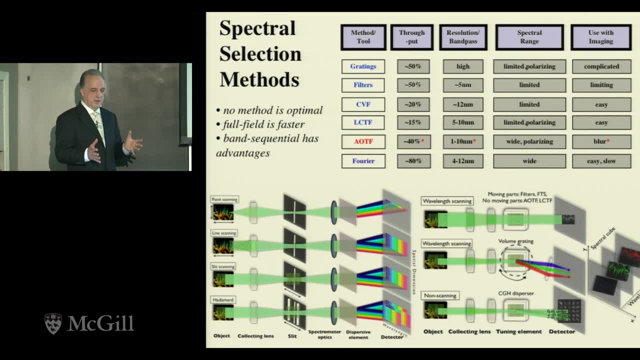 that I'm hoping that he can tell you about, but it's pertaining to Alzheimer's and exosomes. Okay, so let's move in another dimension that can be improved, which is the spectral quality of the light going into the sample and coming out of the sample. 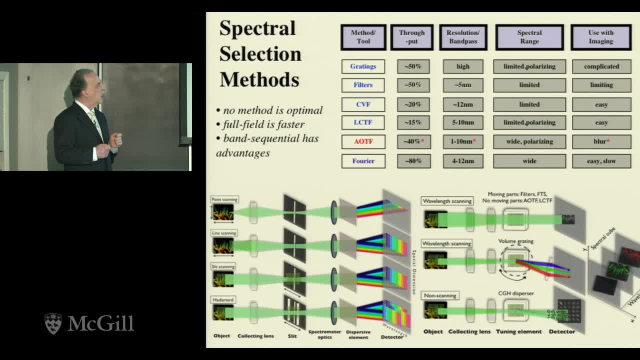 There are many, many ways of doing spectral selection for light, and they are listed here, and they are not even all of them. Okay, so we have pretty much every one of these in our labs, but we got excited about the acoustic optic turnable filters. 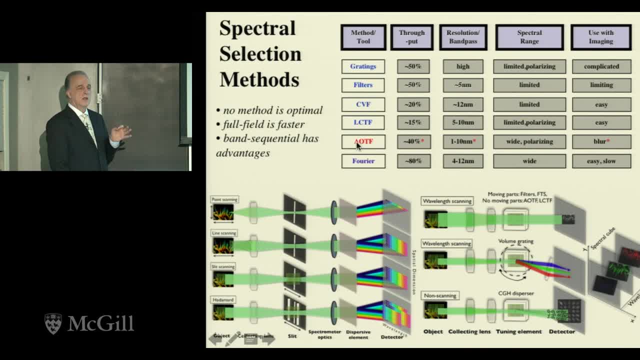 because they have no moving parts and they are really sophisticated instruments that are flying on some of the better satellites, and so we we looked at what are their features and how can they be improved so that they can be used for high resolution imaging. 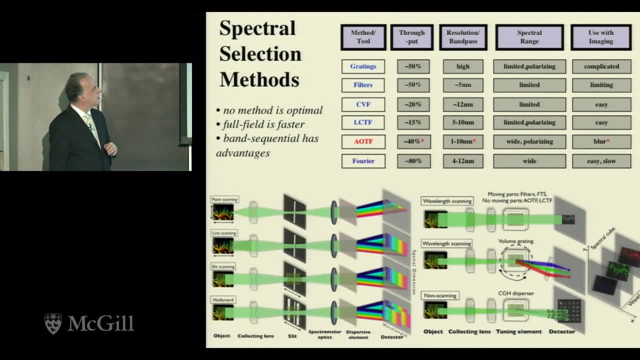 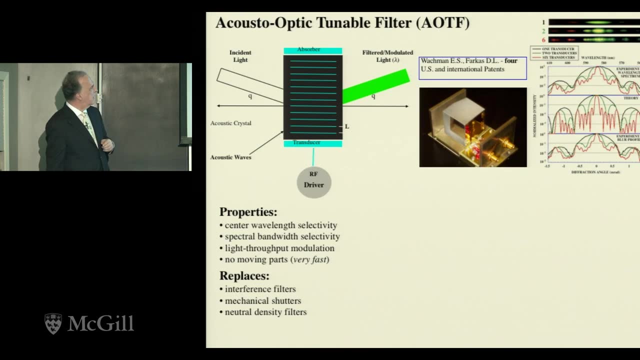 and so this illustrates how the spectral selection is done. but acoustic optic turnable filters are some of the devices by which you can do the spectral acquisition in a way that we prefer, which is so-called band sequential. They replace in microscopy and biomedical imaging. 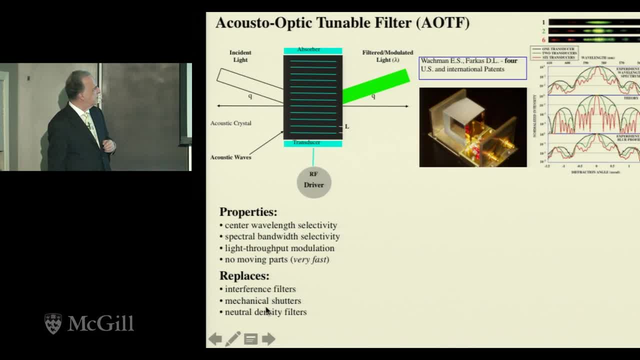 they replace interference filters, mechanical shutters and neutral density filters. it's actually very nice physics behind it. I don't have time to go into it, but it's photon interactions in the crystal. You put ultrasound electrodes onto the crystal and it creates a propagating ultrasound wave. 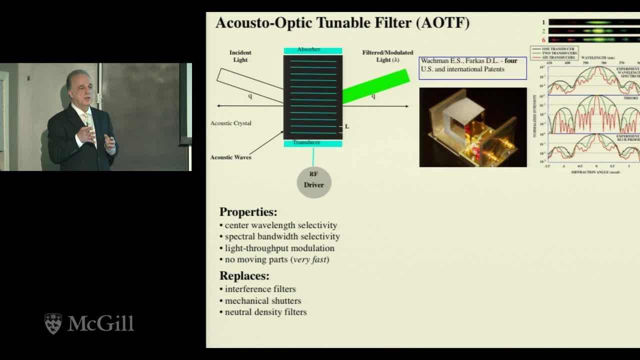 which, in certain crystals that have the right properties, it creates a virtual diffraction grating. Therefore, the white light coming in is diffracted and you control by just electronically tuning the radio frequency. you control the frequency, therefore the wavelengths of the light. 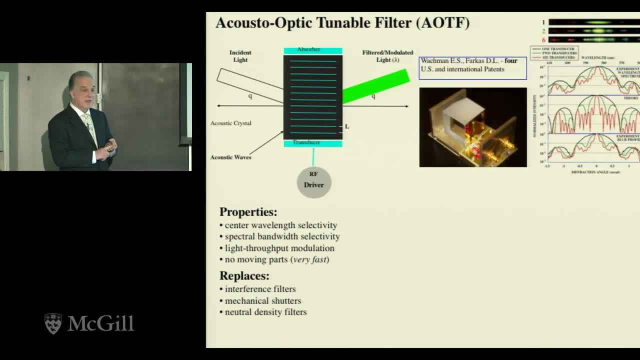 You can control the timing and you can control the intensity, because how much light goes through. So it could be functioning as a microsecond level shutter. It controls pretty much all the features of light that you would like to control And we figured out what were some of the limitations. 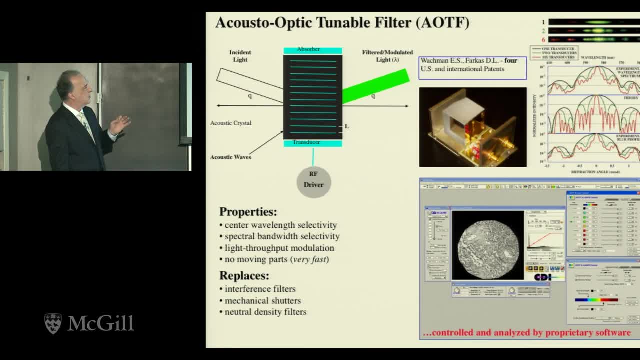 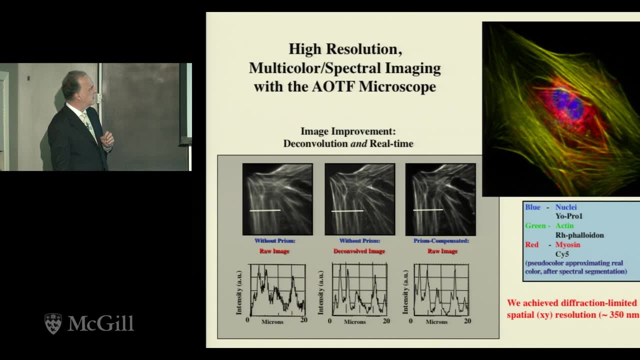 of these and published on it, and so basically we were able to make them good enough for microscopic diffraction, limited spatial resolution imaging, And that's the components of a cell after separation by spectral characterizations through acoustic tunable filters. You can see, for instance, here that there's a doublet here. 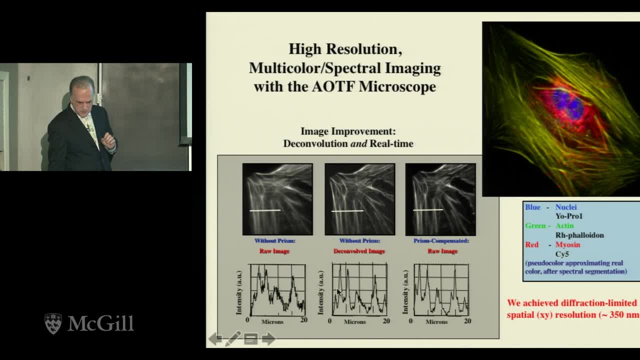 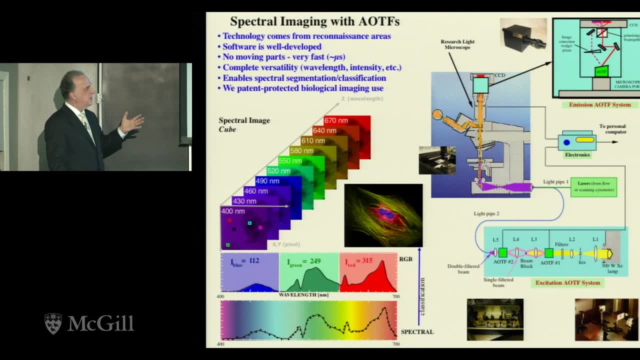 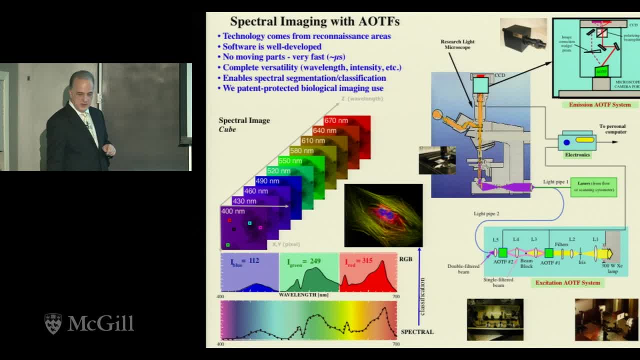 At every pixel you can get the complete spectral signature. So that obviously is quantitatively different from whatever color cameras are doing and which are lumping a lot of information into three channels. So this much more delicate signature allows you to separate something which is just barely different. 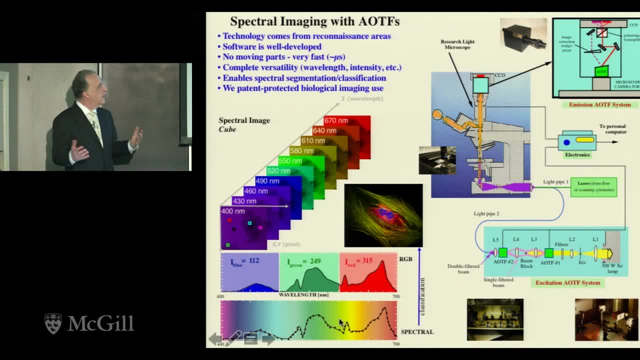 from something else and say this is A, this is B. Okay, So that's a very desirable general capability. so if you can put acoustic optic tunable filters on both the emission side and the excitation side side of a microscope, then you can do quite a versatile set of microscopy experiments. 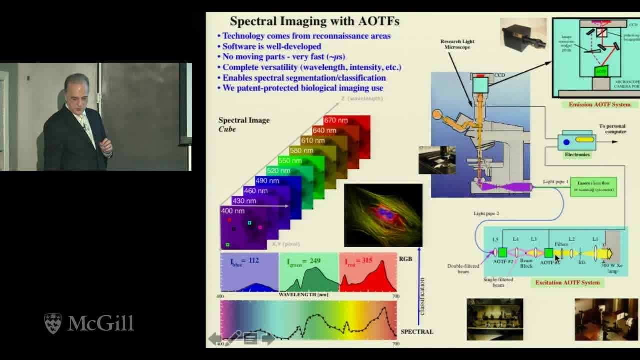 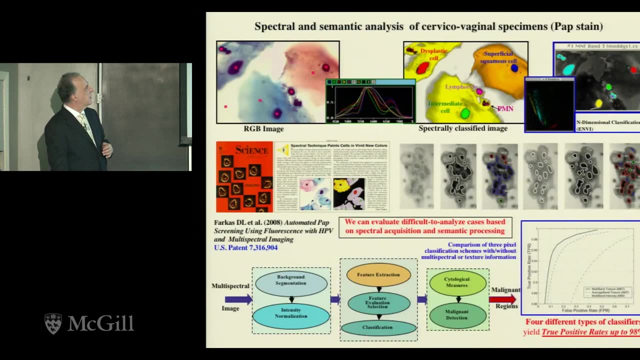 with hyperspectral resolution. But I should say that you can replace the microscope with anything that you prefer. It could be an endoscope, it could be an ophthalmoscope, it could be any optical instrument that could benefit from the additional discrimination ability of hyperspectral imaging. So we applied this to many things. We started with cytopathology. 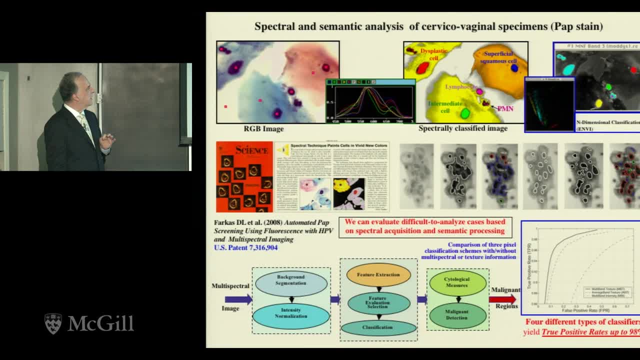 this is pap smears. I'm not going to dwell on it because it's mostly published, but you can get extremely high performance by using spectral segmentation of the images. as you can see here And today, this work is done really by cytotechnologists, who are subjective. 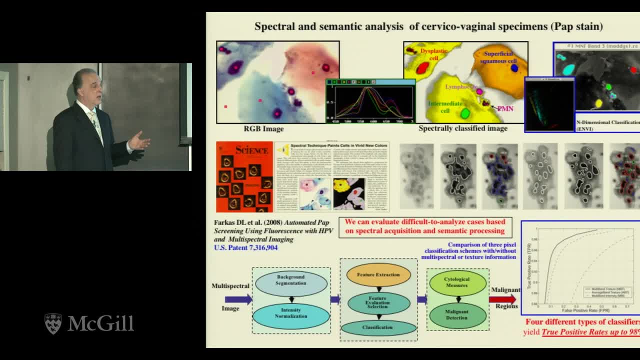 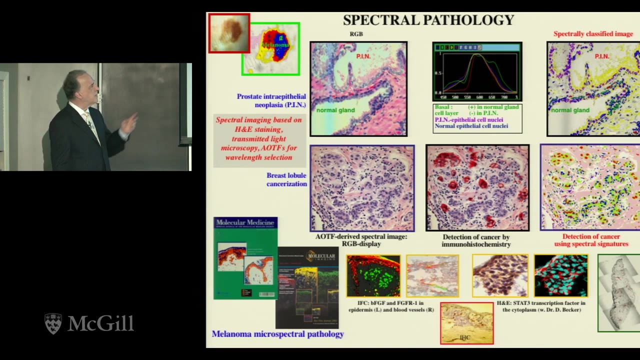 get tired and certainly their performance is not great overall, but in the second four hours of their eight hour shift it gets even worse. So hyperspectral replacement of the determinations is very desirable and we got extremely high specificity and sensitivity with this. You can also do histopathology and again, we published quite a bit on this. 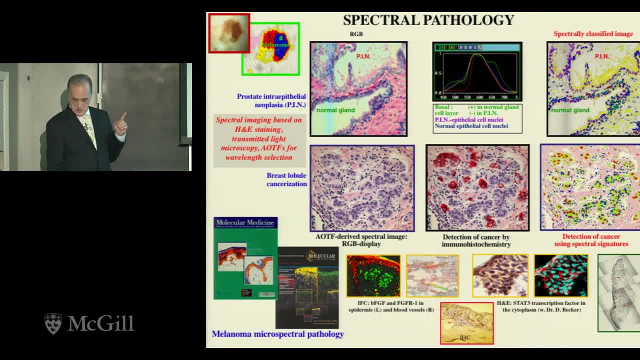 but the point is that we can do by hyperspectral segmentation. we can do as well as some of the really much more specialized methods such as immunohistochemistry does, but without having to do the extra staining and the extra steps. So this was very reproducible. This is a breast cancer example. We also worked on prostate. 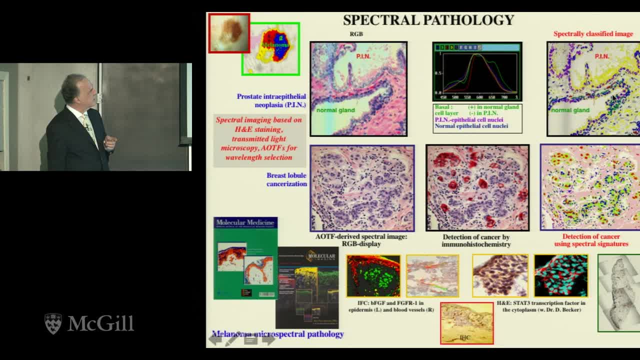 cancer, in which it was easy to see whether this layer of cells is present or not, And then we applied it eventually to what we really were working on very intensely, which is melanoma. I'm going to come back to that in the clinical part of the talk. 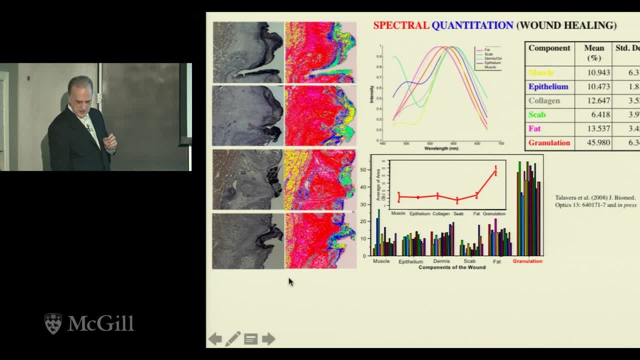 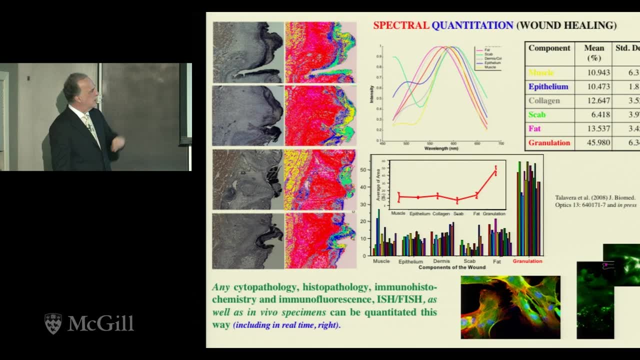 Eventually you can apply it to just about anything. This particular thing here is wound healing. You can characterize very quantitatively what is happening And you can even apply it to in vivo cases all the way on the right, And overall it just allows you to better understand. 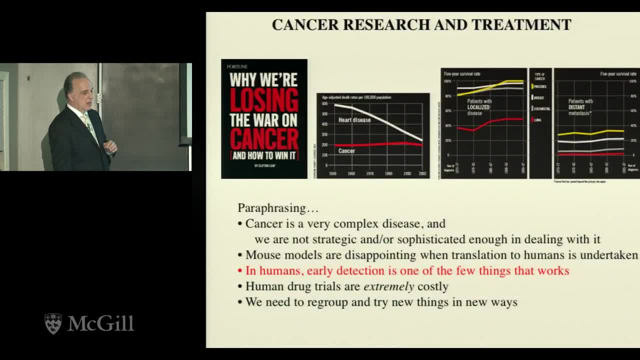 what's happening in your specimen and characterize it quantitatively. So let's turn our attention to cancer, still in the realm of cellular approaches. We don't take our cues from Fortune magazine, but this was, to this day, the most downloaded paper. 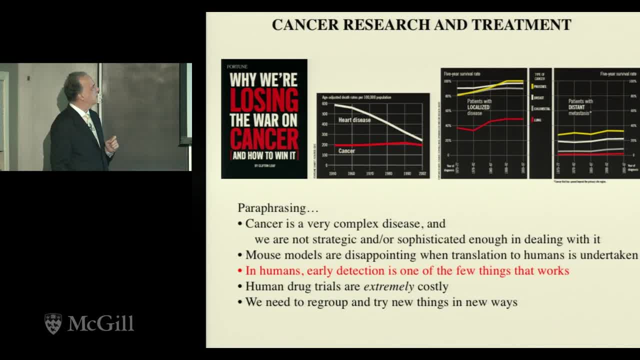 in the history of Fortune magazine And it is a very valuable paper. It actually comes and it was a couple of years ago and it's entitled by a cancer survivor why we are losing the war on cancer. So, paraphrasing: it's a very complex disease. mouse models and animal models have been disappointing. 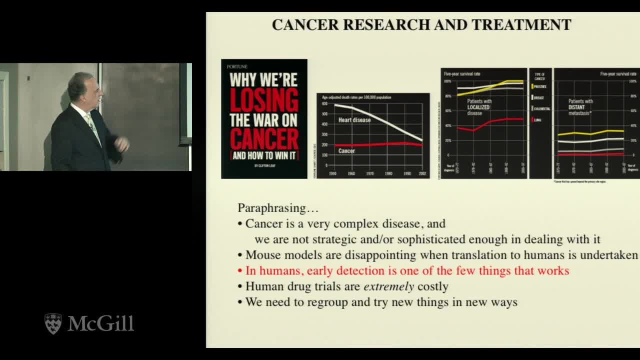 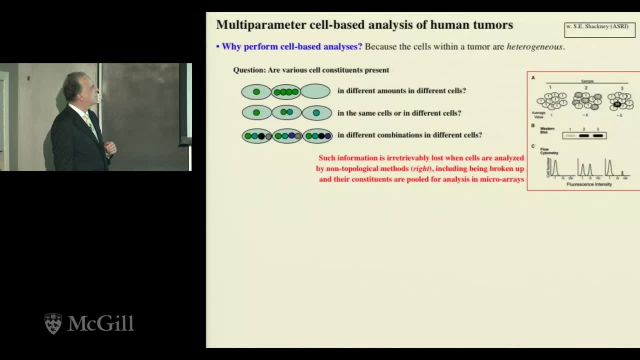 and in humans, early detection is the only thing that kind of works, except for lung cancer, And therefore we might need to regroup and look at some possibly different approaches. So here's one in a moment of enthusiasm. we call it multi-parameter proteomics. 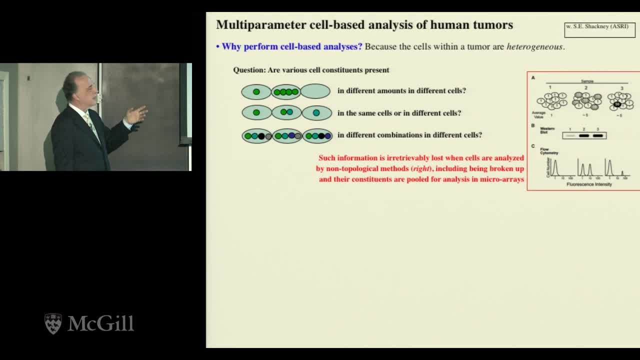 You can start asking questions of this kind. you can read faster than I can talk, but basically are the cellular components present in different cells at different times, or in the same cell? what are they doing? how are they interacting with each other? all of the other methods? 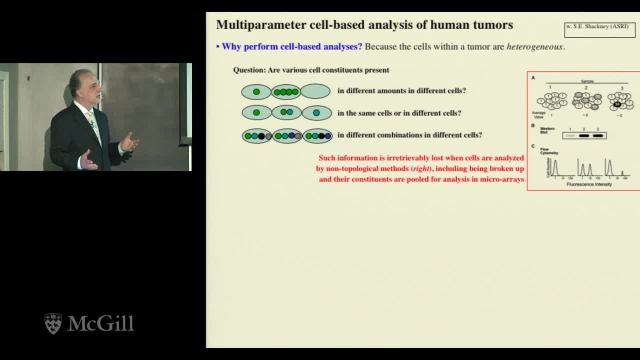 that are currently used- biochemical, molecular, biological- they are all homogenizing the sample and these kinds of questions cannot be asked, So I hope that nobody here is particularly fond of microarrays. is there anybody working on microarrays? Because I'm going to say something pretty bad about them. 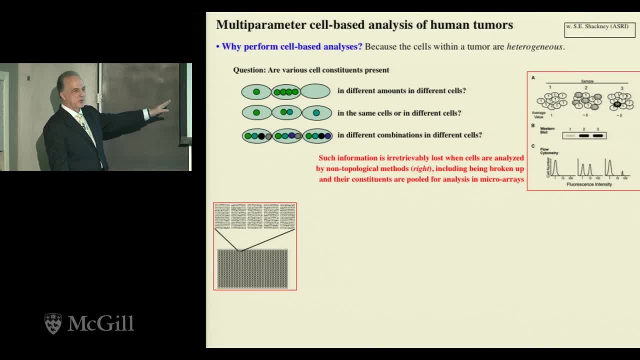 Well, let's put it this way, they have limitations. so when I saw the first microarray that was published by Affymetrix- it was in Science Magazine- I knew that I've seen a picture like this before, and this was in Gulliver's Travels. 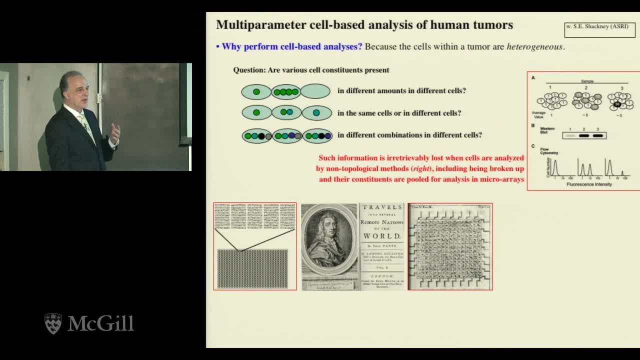 And it was, you know, SWIFT being a big company. Being a very acerbic parodist, he was taking on the Royal Institution and it was describing, at the Grand Academy of Lagado, this impossible, illogical project, and this was one of them. 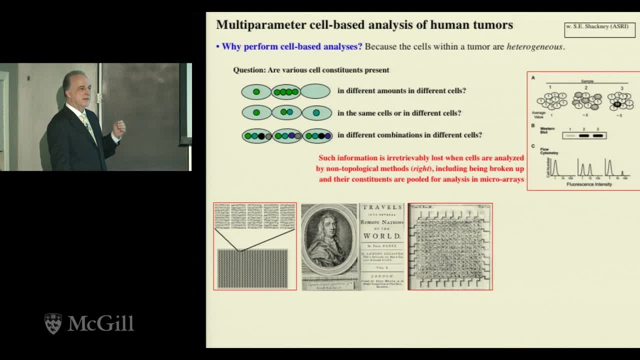 and it was called the literary engine And what it was is that there were 24 students in a class and a professor and 20 students were basically putting all the words on little wooden tablets and with strings and they would pull them, and then the sequence was noted down by the other four students. 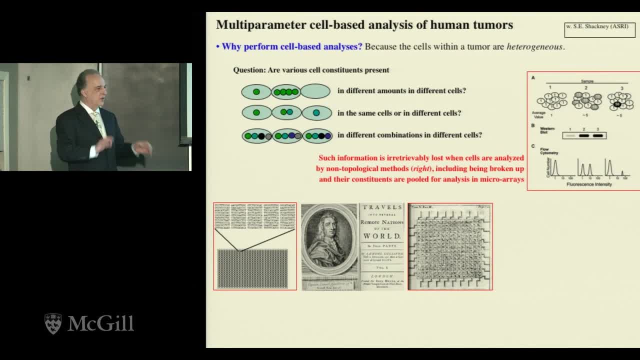 And piled in the corner of the classroom, a huge pile, all of the combinations And the visitor. Gulliver, was told that all of the answers to everything that we seek is in that pile, but we just have to be able to extract it. 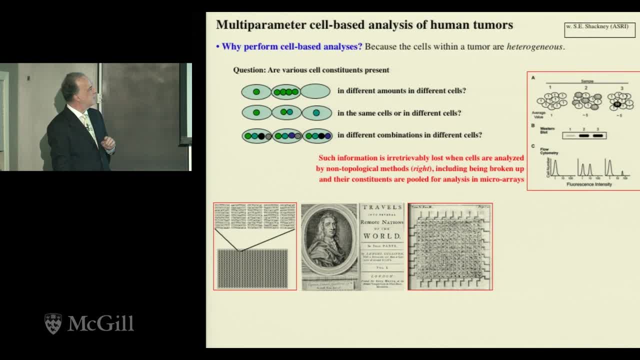 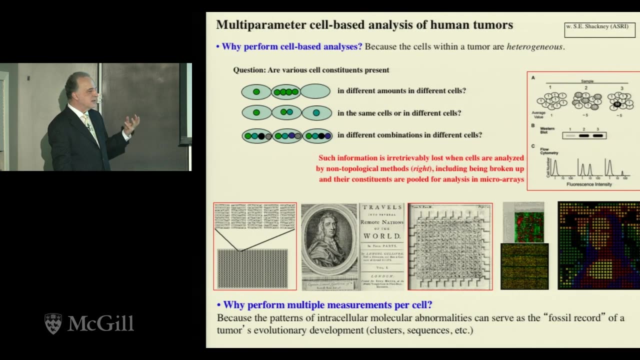 So they were not able, and to this day, by microarrays, we not immediately is it clear what the microarray is telling you Like here. So why perform multiple measurements per cell? Because the patterns of intracellular changes are actually not only telling you where you. 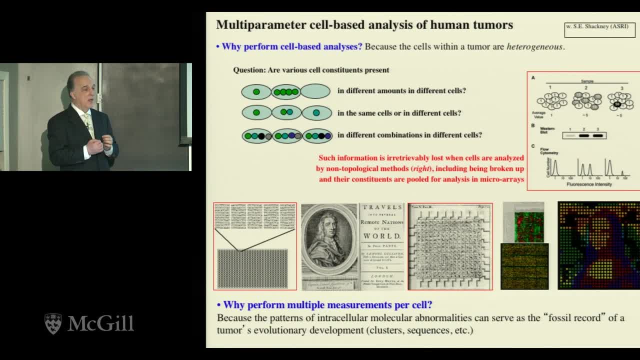 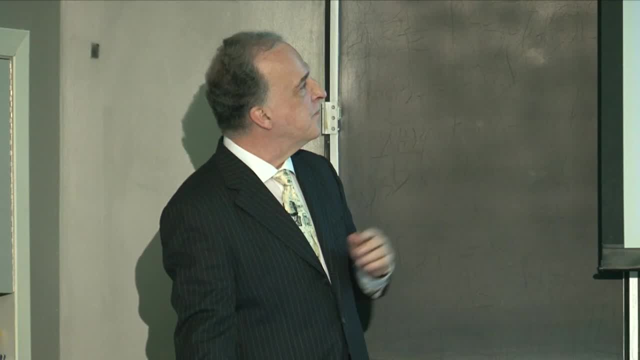 are at with the specimen that you extracted from the patient, but it also tells you the entire fossil history of how you got there, And that is really a very precious capability. So we looked, for instance, with Dr Shackney, we looked at kind of the main players in breast. 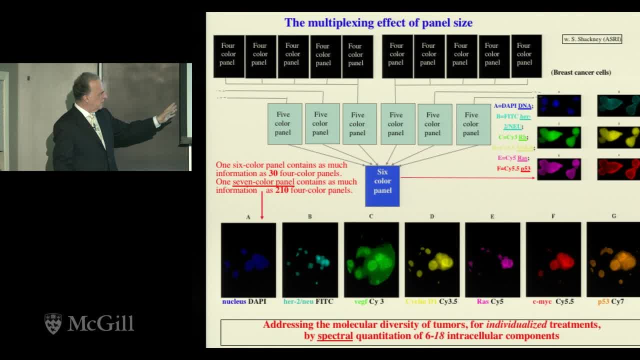 cancer, And this is on the same cells. we were able to label with different fluorescent labels, Hertenu, Cycline D, The nuclei and so forth, to get a much more complete picture And, as you can see, there is a multiplexing effect. 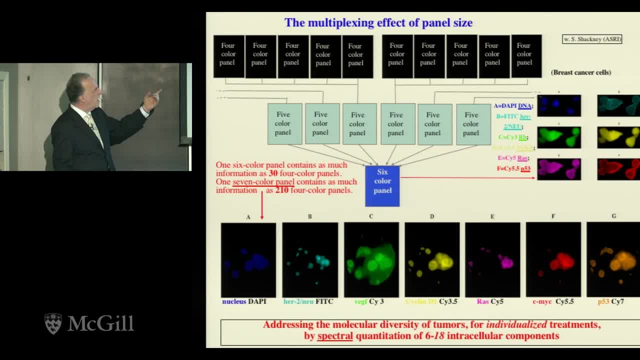 So one seven-color panel contains as much information as 210 four-color panels, And so you would like to know- particularly for the very desirable personalized treatment, you would like to know as much as possible about the cancer that came out of that patient. 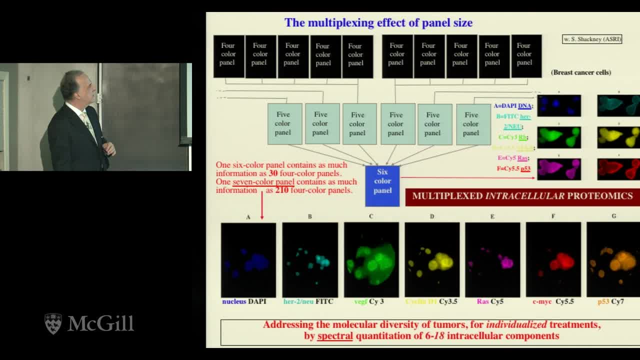 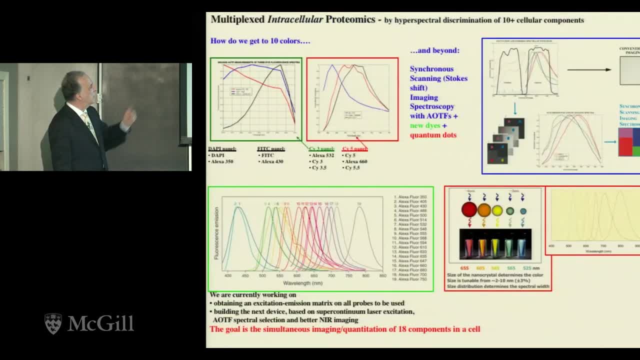 not a general kind of statistically driven approach, And so we were able, so we call this, as I said, multiplexed intracellular. This is still not published Because we were up to 10 colors, which you need hyperspectral imaging to do. 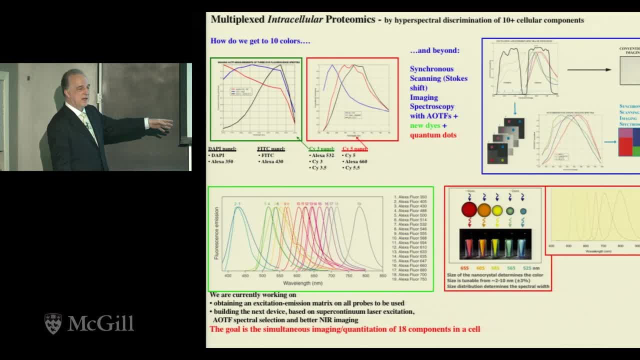 But we were hoping to get to 18.. And there's nothing magical about 18 other than the fact that the world record, as far as we know, is 17 with flow cytometry, And it was done at the NIH a couple of years ago, and multiple physicists need to be in. 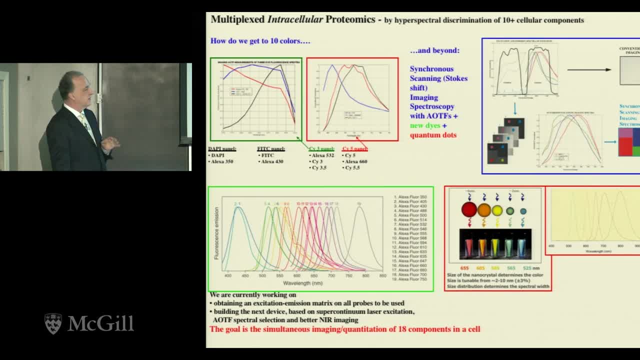 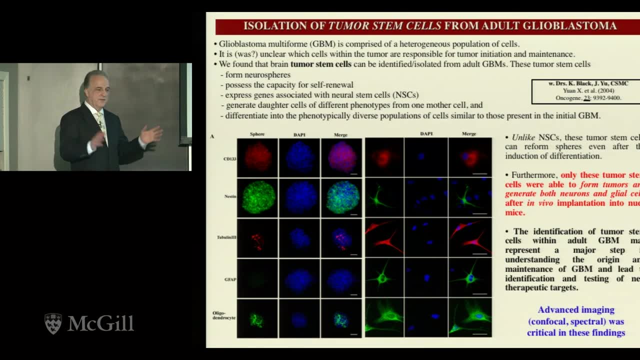 the room and hold hands and chant, but 17,, 17 is the target, And so I'm not going to dwell on this because I have much more to tell you about. So This is a very simple approach, not necessarily with seven colors and so forth, but with confocal. 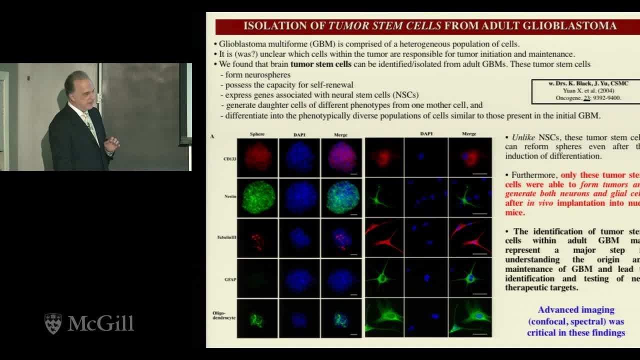 and fluorescence and other good optical methods with microscopy. This was work done at Cedars-Sinai with Dr Blacks and Dr John Hughes' group. We were able, pretty much simultaneously with a group in Toronto, to publish for the first time in a cancer journal on cancer stem cells. 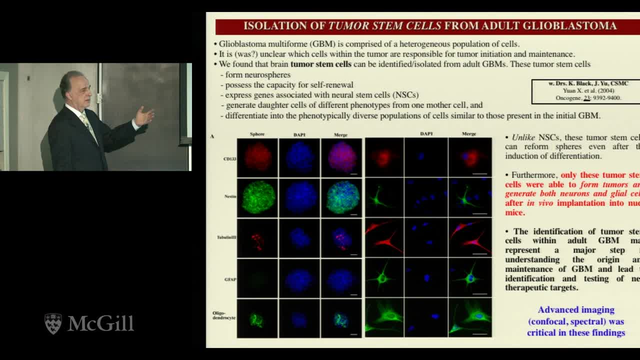 These are really scary cells that can regenerate In animal models. you can regenerate both the regular cells in the brain but also the glioblastomas, And since then obviously there has been a lot of progress in the field. but basically, both pharma and others will tell you that these are the real cells that make cancers come back and be such a bad scenario. So the various treatments get rid of 99% of the cancers, but if these guys are still around these stem cells, they can recreate any of the any of the bad tracks. 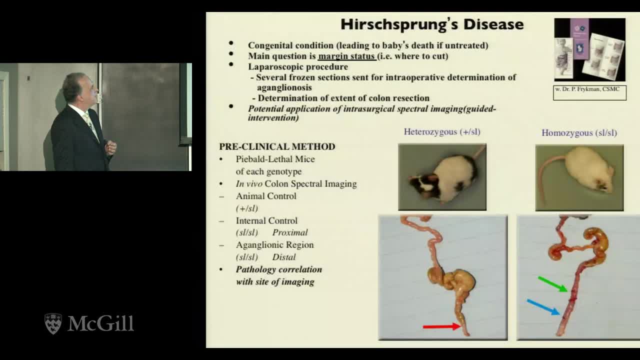 Yeah, Yeah, Yes, Okay. So let's move on now to some animal work. So before tackling things like cancer in animals in preclinical models, we always try to start with something a little bit simpler that we understand better. This is one example. 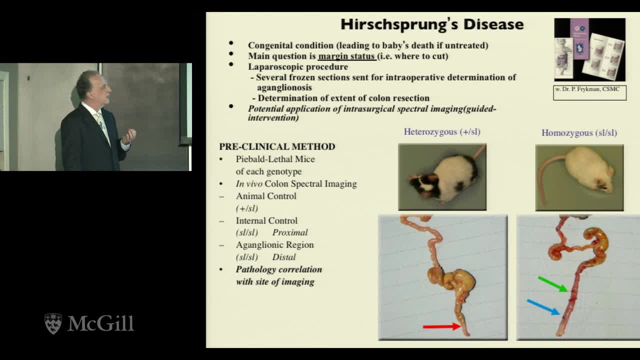 Again, I'm not going to dwell on the specifics, but there's a children's congenital disease called Hirschsprung's disease. The colon of the newborn is basically not fully innervated, Starting at a certain point it's aganglionic and therefore the proper functioning of the 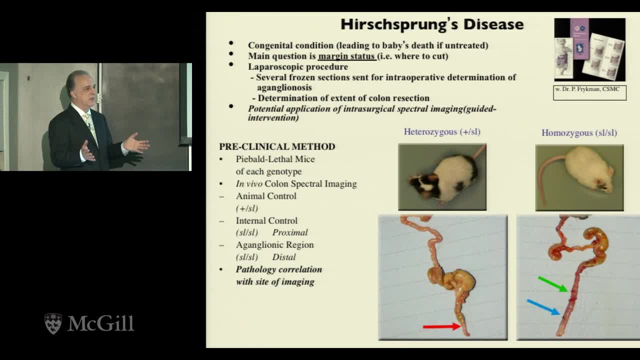 colon is impeded And if you don't intervene, Yeah, And the babies basically would die in a week or two. And so therefore, people discover that this is congenital and therefore intervention is needed. In the old days they used to do open surgery, which is terrible, as you can imagine. 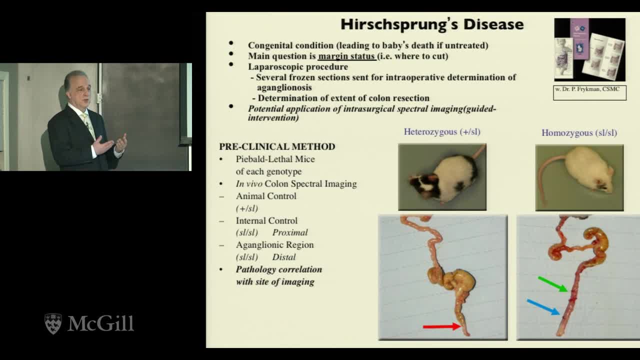 And the only improvement on that in the last couple of years has been that now they do it endoscopically. But still, coming in endoscopically you have to determine where to cut so that the part that is not functional is taken out and then the whole system is reconnected. 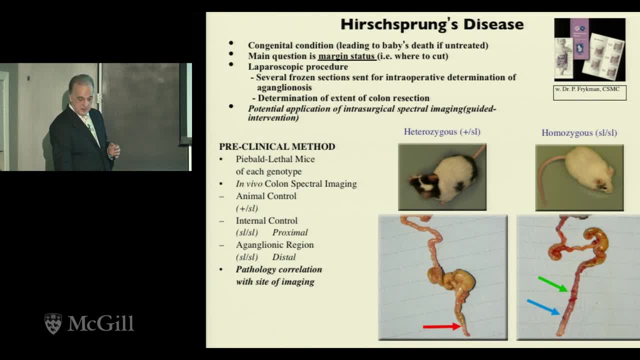 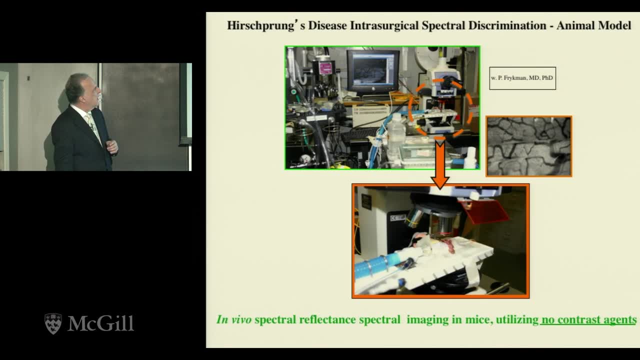 So that cutting has been done based on eyeballing And the better. pediatric surgeons will tell you that One of those surgeons came to us, Dr Frickman, and we did first animal experiments on Hirschsprung's disease and then he obtained an IRB to do also trials on babies at the Children's Hospital. 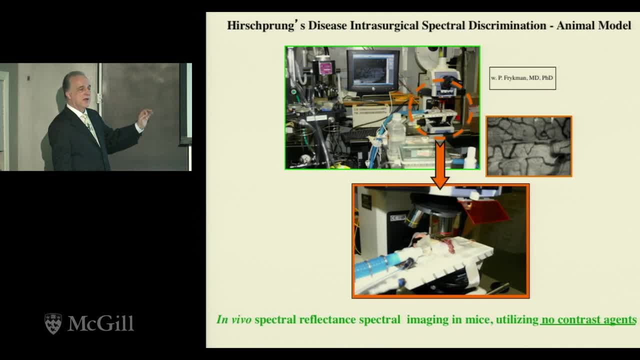 in Los Angeles And all we are doing is reflectance spectral imaging to try to characterize the tissue and see, for instance, on the right on the tissue, where to cut. Okay, So one of those principles: if you cut too much, it's not good. 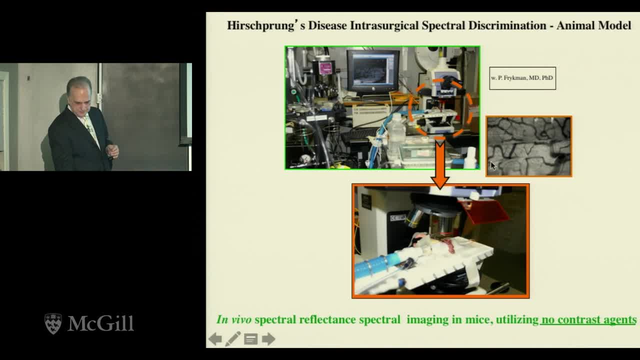 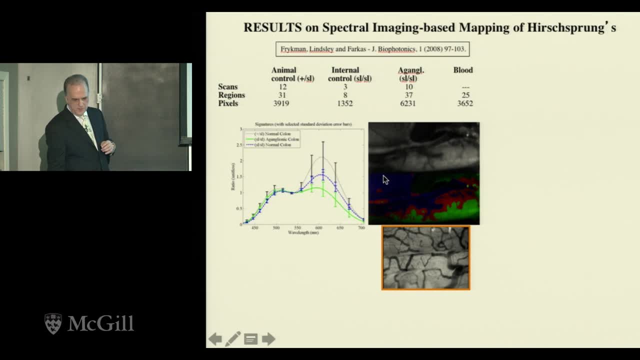 If you cut too little, it's certainly not good, And so we were able to, by spectral segmentation, to find this transitional region that you may see in blue here And then obviously, this is the bad part. So the reason that I'm showing this is that we did take full spectral measurements, but 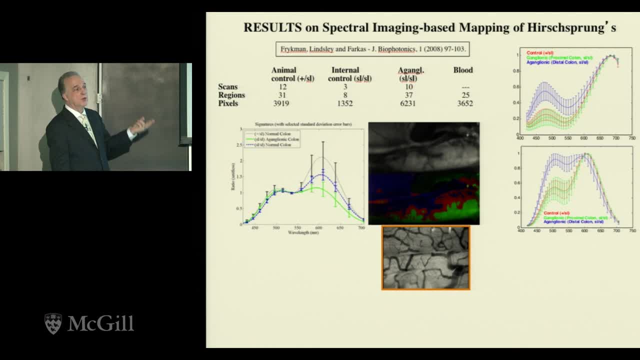 it turns out that ultimately you only need three wavelengths, But you don't know which those three wavelengths are Until you do the full spectral measurements. So we have found that actually, if you take the ratio at 609 nanometers between the intensities, 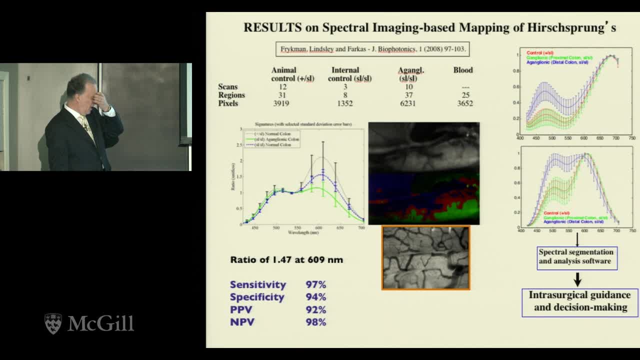 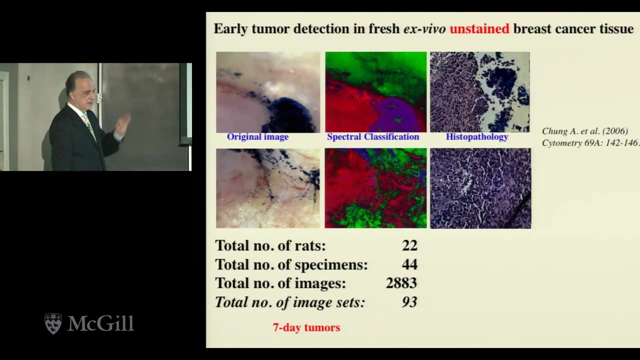 you can get extremely high sensitivity and specificity, determination of where you need to do the surgical intervention. So the topological guidance. This is very rapid and the transition zone is highlighted. It's also published, so I'm not going to dwell on it. 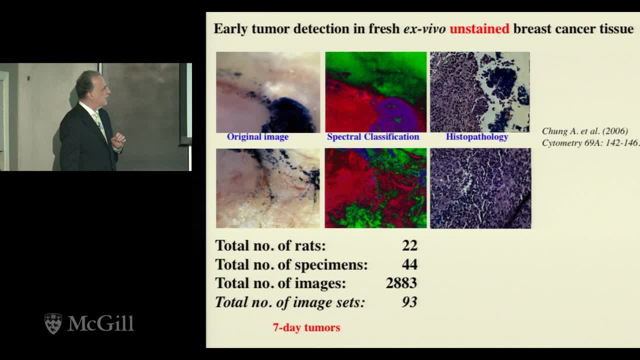 So let's move to Canada. This is the case for cancer, So we were able to use an animal model of cancer, A resident, a surgical resident, who is now a big-time cancer surgeon. Alice Chung was driving this work, So we were inducing cancers in rats. 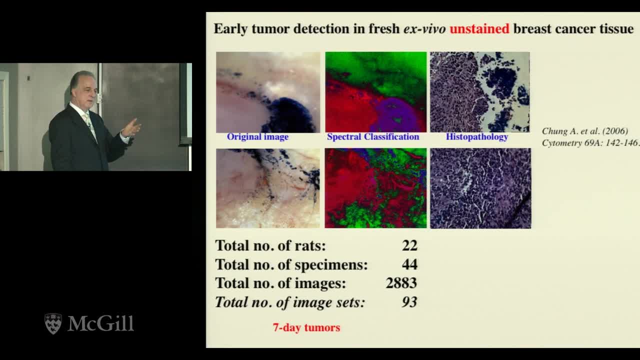 These were human cancer cell lines that were being injected and they would come up in approximately a week. We did not want to look when it's a clear cancer that you can see with an naked eye. We wanted to look at the earliest possible time and see whether there was no contrast. 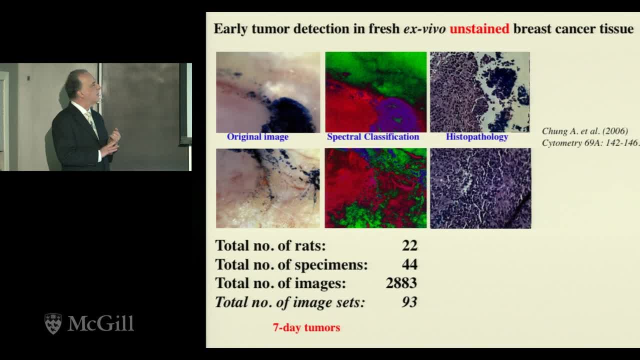 agent- which also is going to be a motif in what I'm telling you about- where there was no contrast agent and that's verified by histopathology whether we can see cancers in these animals. And so we looked at a total of 2,800 images and this was seven day tumors and we were 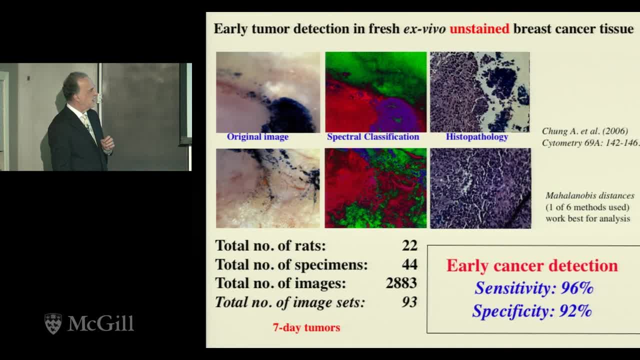 able to, with very high sensitivity and specificity, find these tumors. I should say also that we used six different image analysis methods to look at the spectral data sets and, for reasons that are still not 100% clear, certain methods were better than others. 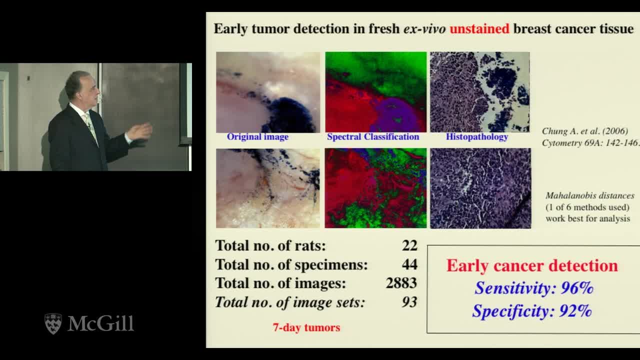 So in this particular case Mahalanobi's distances was better than Euclidean distances or principal components or even support vector machines. So in this particular case that was the way to go. So it also became clear that if you want to tackle something complicated like cancer, 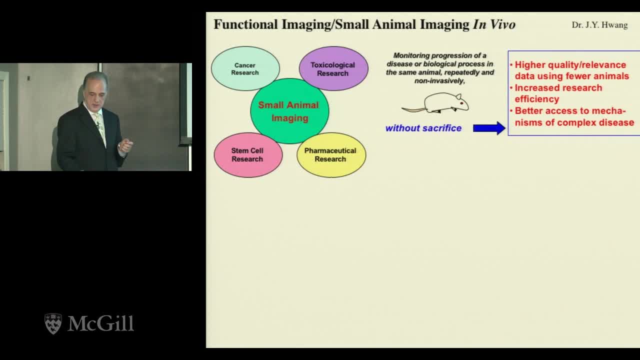 you may want to not look in just one way, but look in multiple different ways. So we started with Jay Huang. He was He was originally a graduate student from USC and then he stayed on as a postdoc and drove the interface between our project and Caltech to develop a small animal imaging. 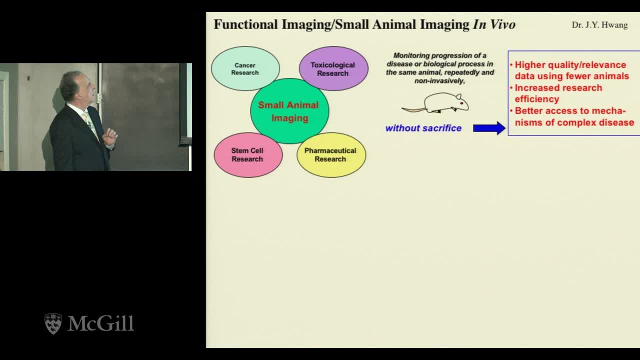 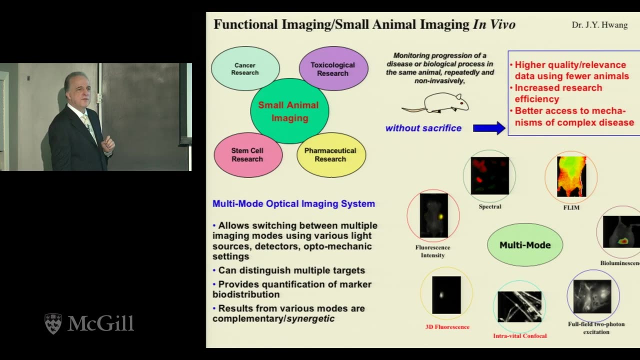 system that is multi-mode imaging. There are multiple reasons why you would want to do multi-mode small animal imaging. You can distinguish multiple targets and you can classify better. So we built a system. We built a system in which there were seven different ways in which you can look at your 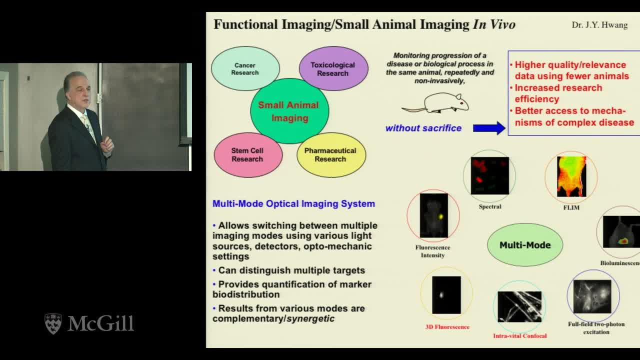 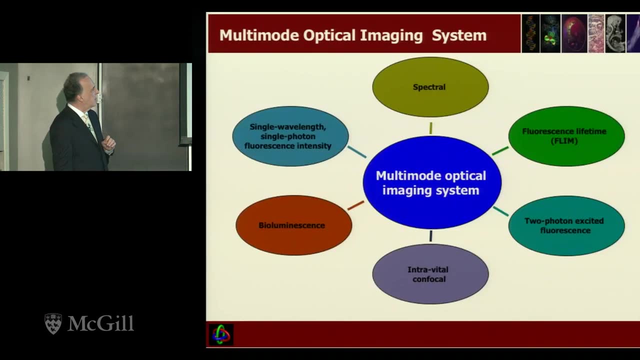 animal models of disease. Some of them are very easy to understand, like spectral and fluorescence, but also lifetime of fluorescence, luminescence, 3D fluorescence and even confocal. And so this is the system, schematically, and the reason that you want to bother putting. 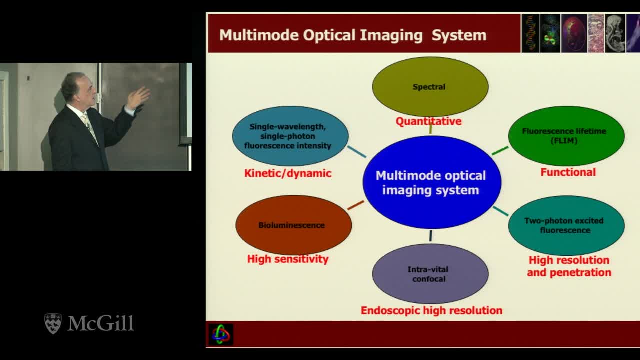 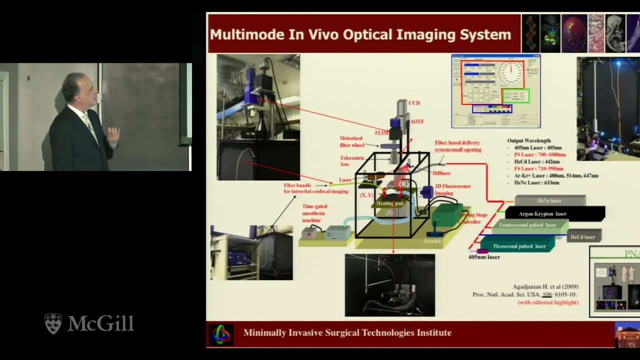 all these methods in is that each is better at something. So spectral is extremely good at quantitation. Intravital confocal gives you endoscopic high resolution. Kinetics are best monitored with single wavelength, single photon, fluorescence and so on. So this is the system schematic. 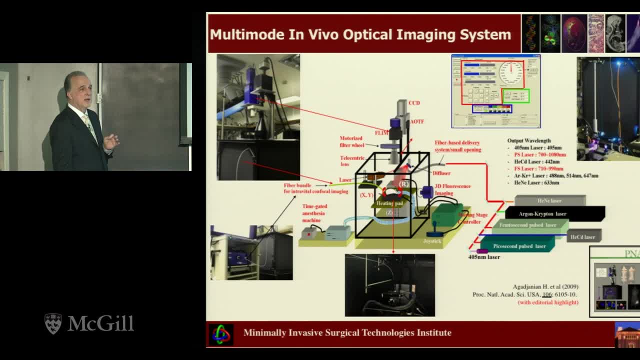 William Blake once said that you never know what is enough until you know what is more than enough. So we had seven lasers in the system. It's not likely that the hospital or even another research lab will go into that sort of trouble. but again, you want to learn more. 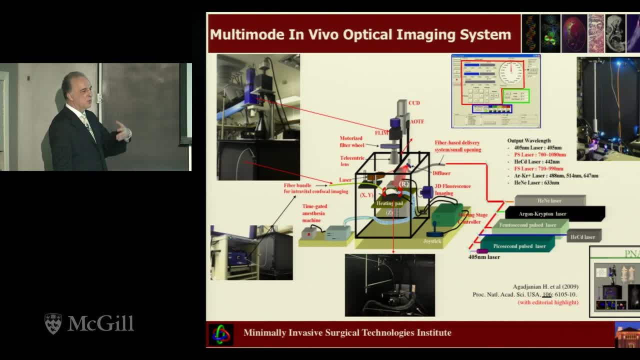 So that you can then refine it, particularly for the clinic, in what are the two methods or three methods that you would like to capture. So this thing was able to do seven, and this is the layout, And this is it in real life. 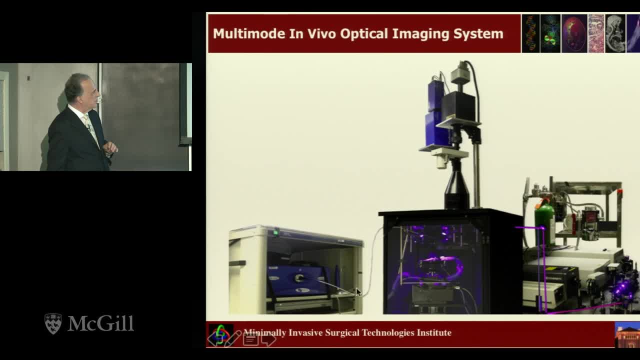 Here on the left. this is a commercial device that we added, So this was the confocal imaging. It's a beautiful system that was developed by a French company called Mauna Kea Technologies, And we were able to do significantly better in terms of contrast. 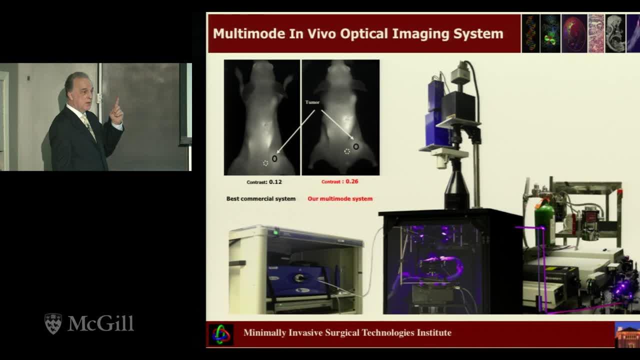 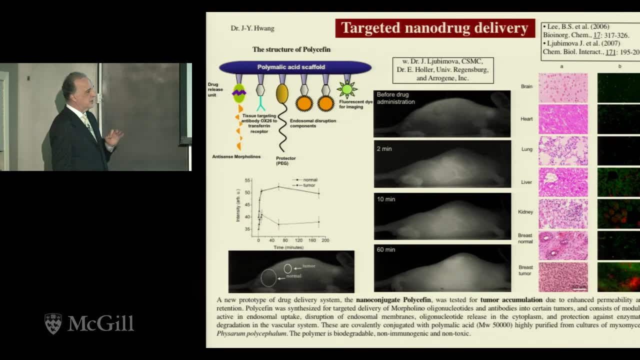 And then the best, most expensive commercial system, but which only had one mode of imaging And we published quite a bit on it. So I'm not going to give you too many examples, just three very quick ones. This one with Dr Lyubimova and her group. it's a nanoconstruct in which you basically 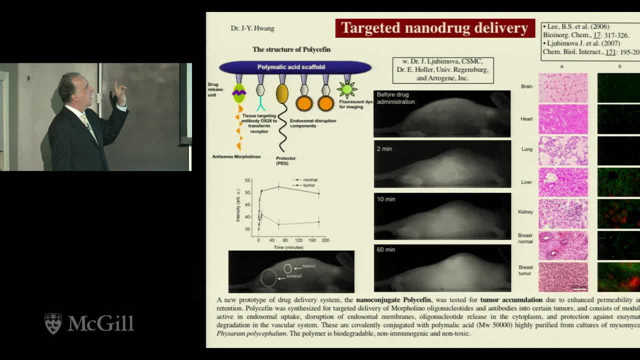 have this drug that you are constructing. It has a tracking moiety which is fluorescent and you can track it through the body of the animal, particularly if it's more towards the red and near infrared. It also has some binding moieties that will make sure that the targeting is pretty specific. 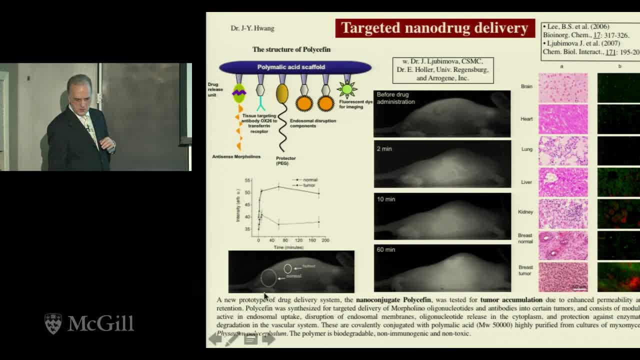 And then it has some destructive elements to it which enables you to basically kill the tumors that it is connecting to. So you can see kinetically how the signal is rising. This is a tumor that we induced in mice And it's confirmed by histopathology and fluorescence here. 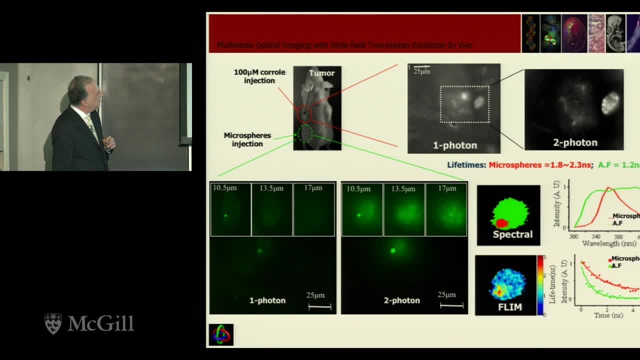 The second application I'm not going to To dwell on this. this is work on corals. This is a family of very interesting molecules that were developed in a collaboration between the Technion and Caltech by Zev Gross and Harry Gray's group. 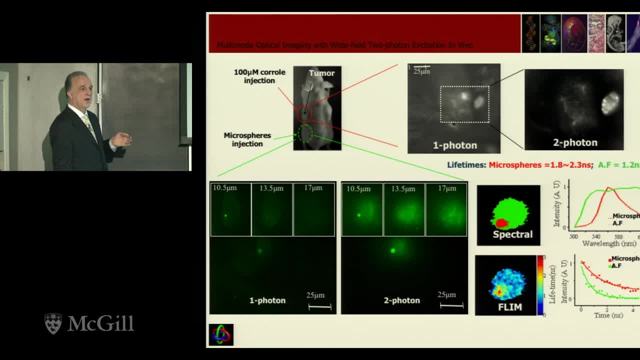 And these molecules are able to function as chemotherapy agents. but then it turns out that if you do certain additional things, they would function as multi-pronged chemotherapy agents. For instance, they also have a pretty strong photodynamic effect. They can kill the cancer cells in at least three different ways. 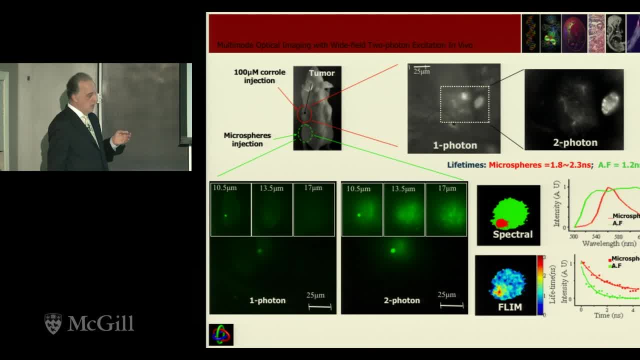 And again we published quite a bit on it. But in order to track them in the early going you need a combination of methods And for instance, here you can see how much deeper you can penetrate with two photons versus one photon. We also did lifetime of fluorescence and spectral segmentation to see where the molecules would. 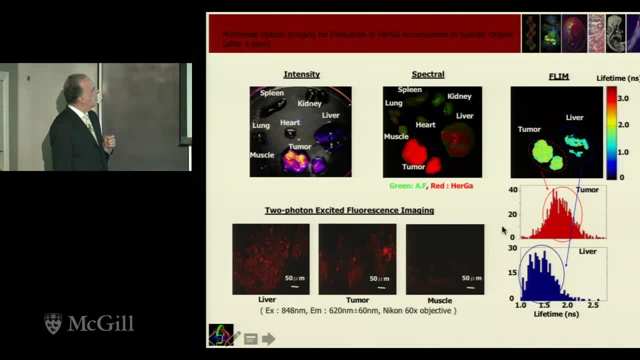 go and attack the tumor And you can see, for instance, that the segmentation is boosted, Boost by spectral and fluorescence. lifetime is pretty clear, much more so than in just taking pictures of the animal's organs, And then, ultimately, you can do a little bit better than that. 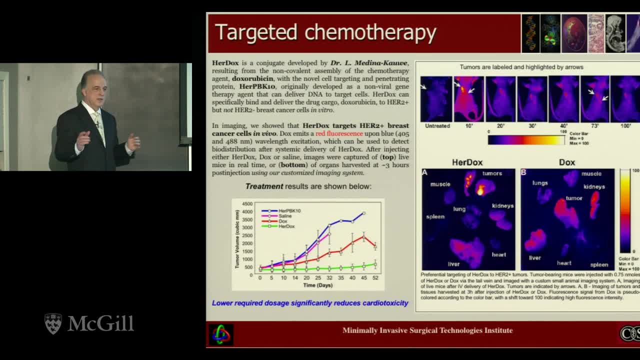 And what you do is you take any of your favorite chemotherapy agents- either because they're already around and approved even for human use, like doxorubicin or these corals, and you can attach them to something that targets extremely well. 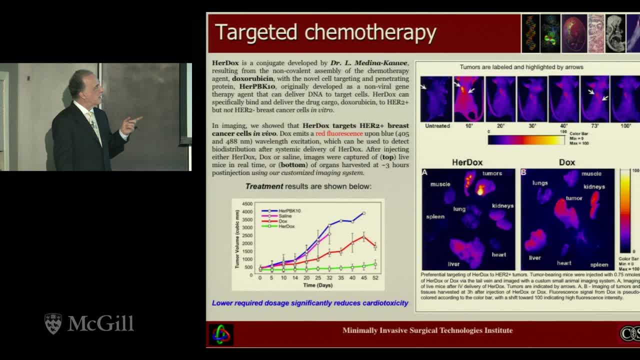 So this is in collaboration with Dr Levin Lali Medinakawe at Cedars-Sinai. they developed a very, very specific targeting agent molecule that was developed originally for gene therapy And it didn't work quite that well in gene therapy. but if you take it and attach doxorubicin, 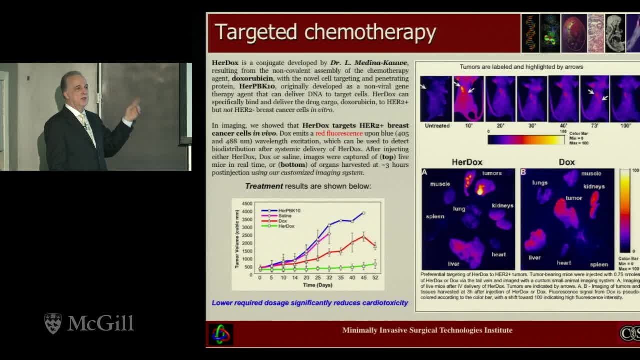 to it. for instance, you can use concentrations as little as 20 to 100 times less than the normal levels of doxorubicin and get the same effect. So here you can see that And you have basically a killing of the tumor with this targeted doxorubicin. 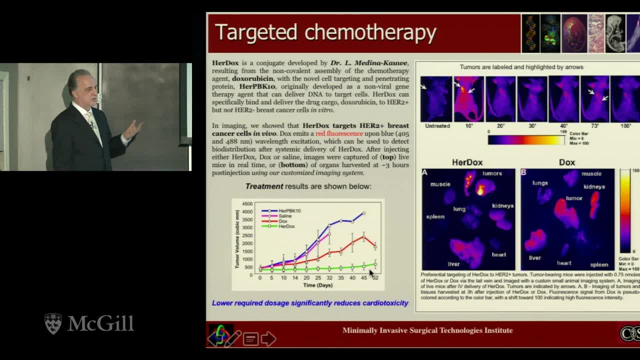 Now we also used it with the corals and it was very nice results in terms of efficacy of killing cancer. So the lower doses obviously prevent all of the bad side effects of chemo and so forth. So this is an exciting way of proceeding. 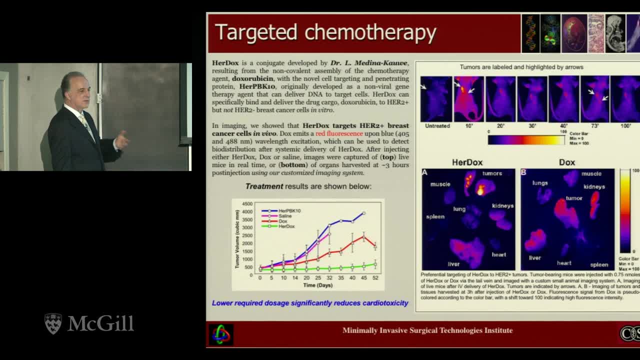 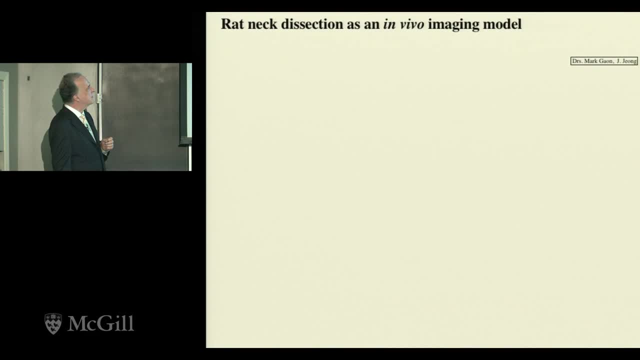 And I don't think that without the optical methods you could have figured out these sort of things from other types of biomedical imaging which is more accepted in the clinic. These are just some of the publications, so I'm not going to go into more details. 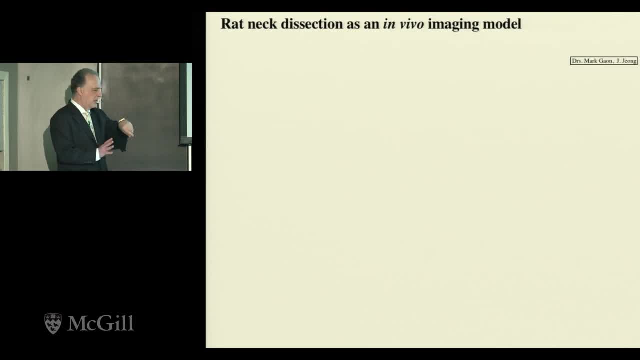 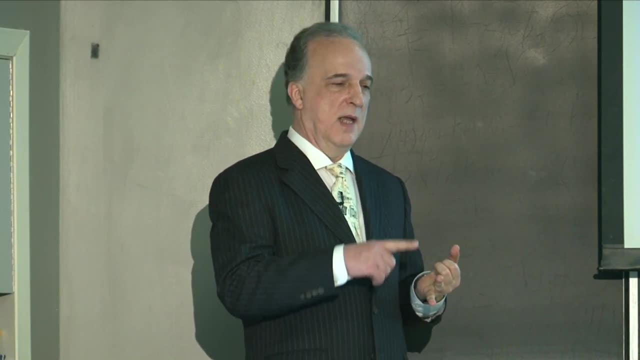 So we would like to do first preclinical and then clinical work, but ideally without using any contrast agents. So one way to go about that is to have your effector molecules, such as the corals, also be a contrast agent, So you don't need to rely on the availability and the targeting ability and so forth of 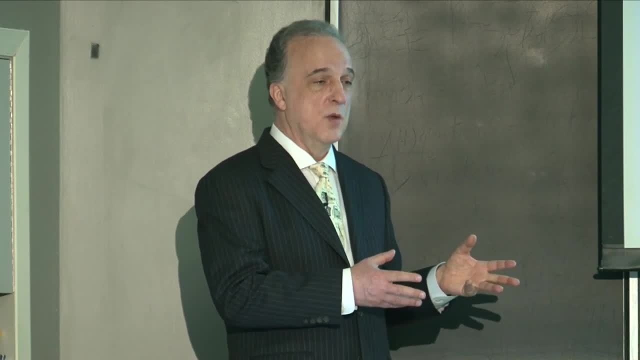 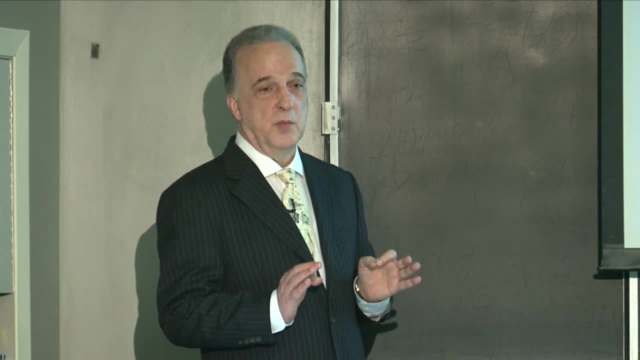 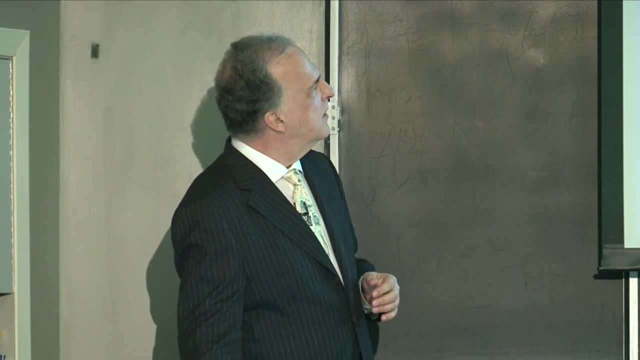 contrast agents, But you just rely on the molecules that you're using anyway To get rid of the cancer. The other way to go about this, which is a little bit more difficult, is to just use intrinsic signatures of the body, And for that I would say, generally speaking, you need better optical technologies. 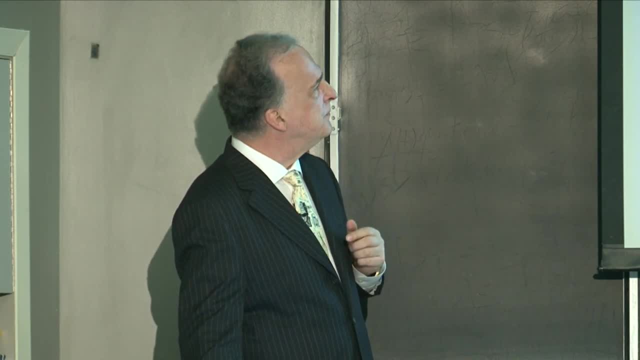 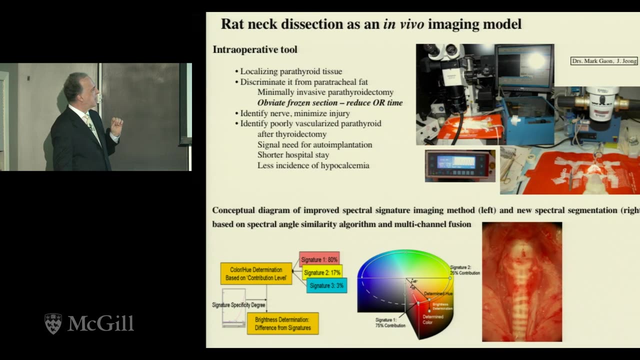 So, again, starting with something that is not quite as complicated as cancer, we were looking at the necks of rats being imaged for thyroid and parathyroid, and Ji-Hoon Jung, in our labs, developed a, A rather sophisticated spectral analysis program to look at non-stained tissue. 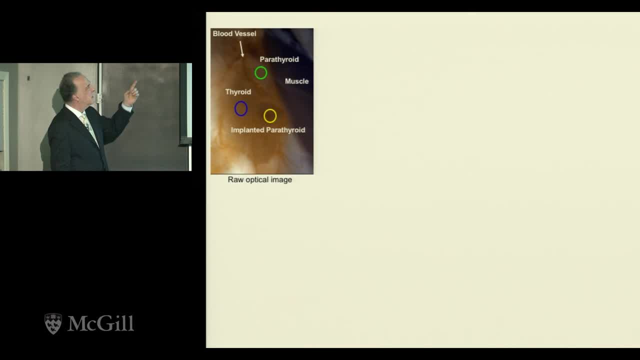 And so if you just look at it with the naked eye, you can't tell what's what. If you look at it with regular spectral segmentation, it's very tough to see what is going on, whether it's the parathyroid, whether it's the thyroid, whether it's muscle. 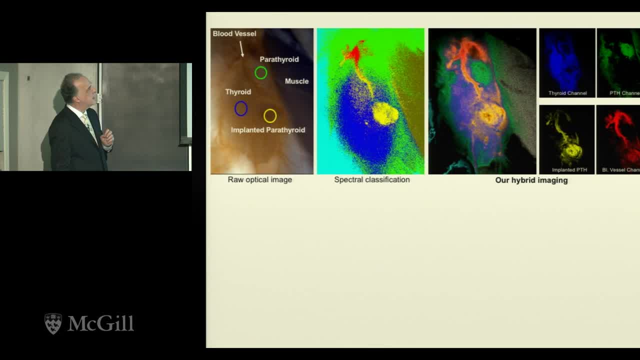 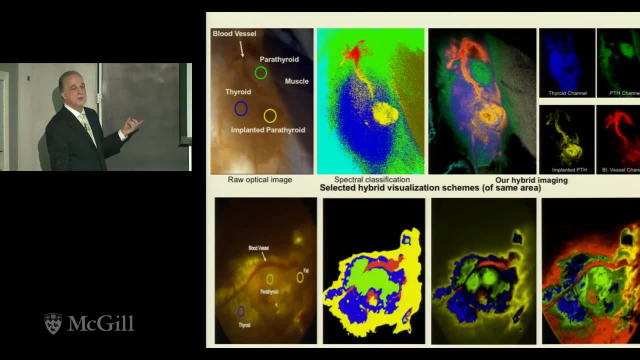 But as you start getting a little bit more sophisticated with the analysis, you can actually separate into different channels the various interesting components And then you can remap them depending on what you are interested in. If you are interested in, I mean, what happens to, let's say, a cancer, you can highlight that. 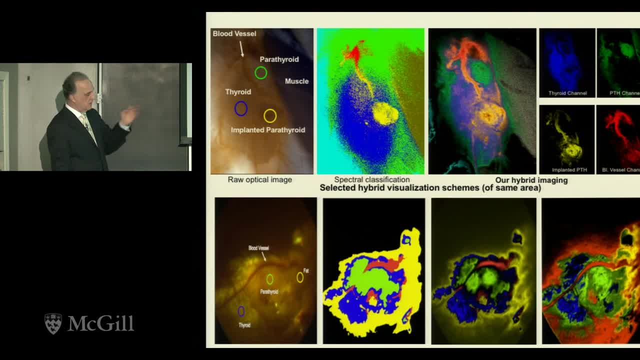 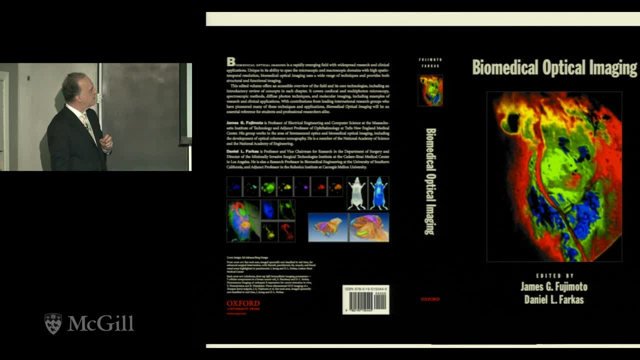 If you are interested in what happens in terms of the vascularity, you can highlight that, And so this so-called florid picture on the right ended up on a cover of a book that we did a couple of years ago with Jim Fujimoto. 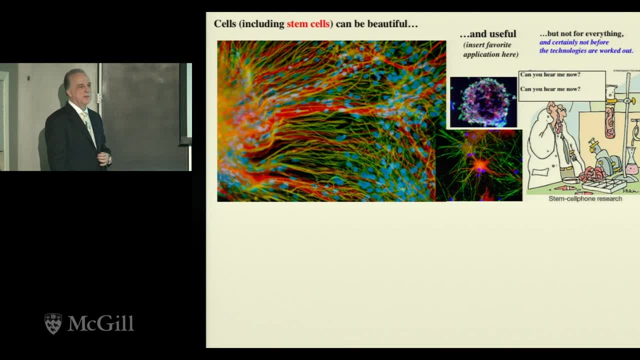 So let's take a two-minute, three-minute detour and talk about stem cells, because everybody likes stem cells. They are a very exciting part of regenerative medicine in general and stem cells in principle are wonderful. But what is kind of an unstated assumption is that once you put these magical cells into, 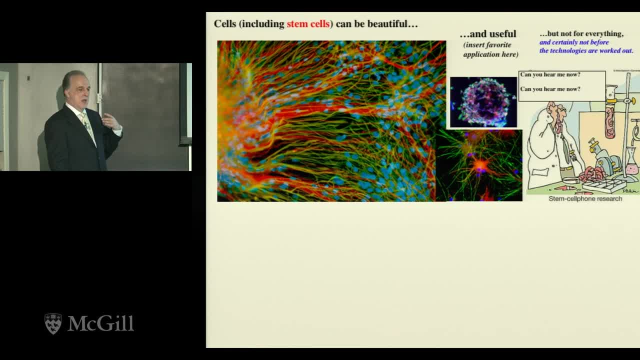 the body in order to achieve some clinical outcome. all of the things that you hope to happen happen and none of the things that you don't want to happen happen, And that's a nice assumption, but you would like to, rather, you would prefer to see it. 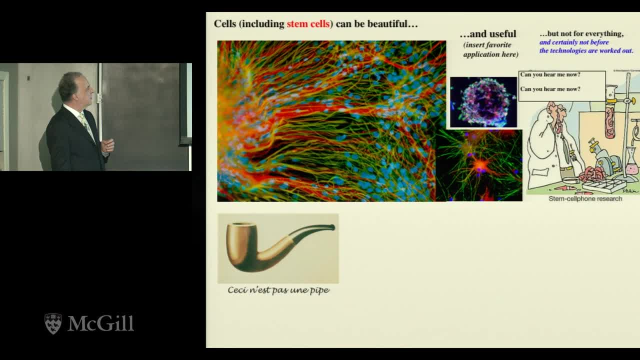 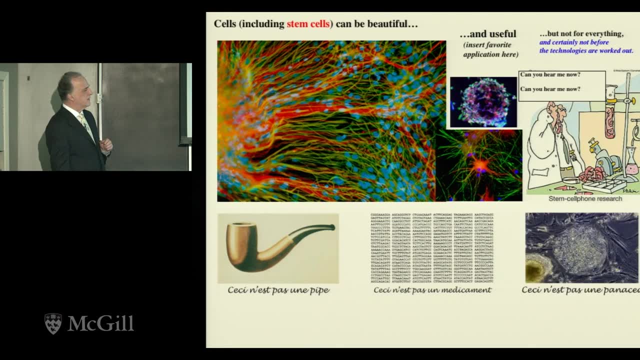 And so, with apologies to Monsieur Magritte, just like this is not a pipe and this is not a drug, This is not a panacea of the stem cells, But if you can track them in the body, then maybe you can start seeing something about. 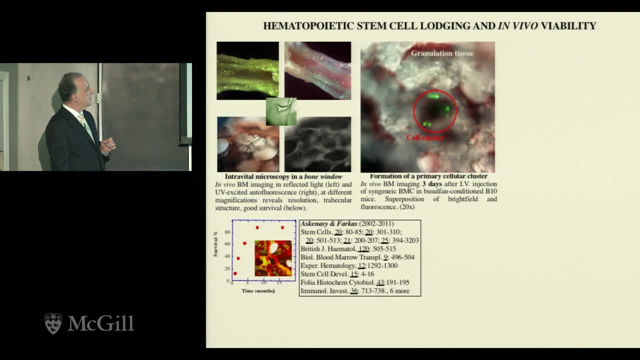 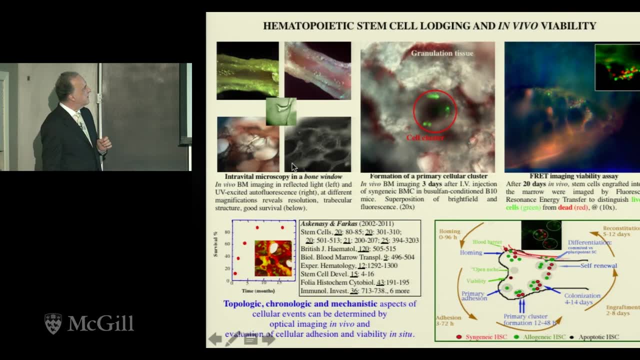 the mechanism of action. So it's just one slide here because it summarizes years of work. but- and I'll try to point, So this is mostly with Dr Askenazy- We were able to label stem cells and inject them into animals, into the femurs, through 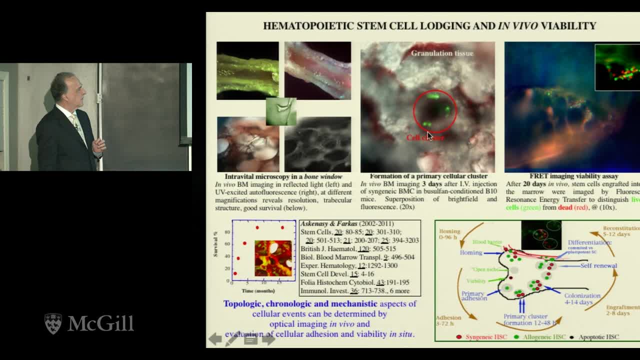 circulation. They made it into the femurs of animals. So this is the first slide, This is the second slide, And this is the second slide And we can see that they are in the femurs of mice And they were embedding and grafting into the tissue there. 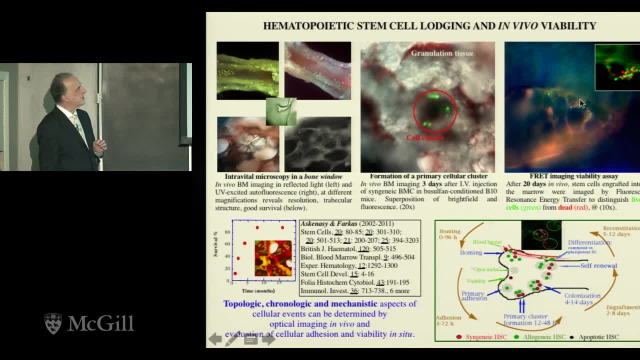 And we even came up with some methods by which, through fluorescence resonance energy transfer, up to three weeks after the injection we can see them in vivo and we can also tell the live ones from the dead ones. This is done with PKH, DICE and first-order energy transfer. 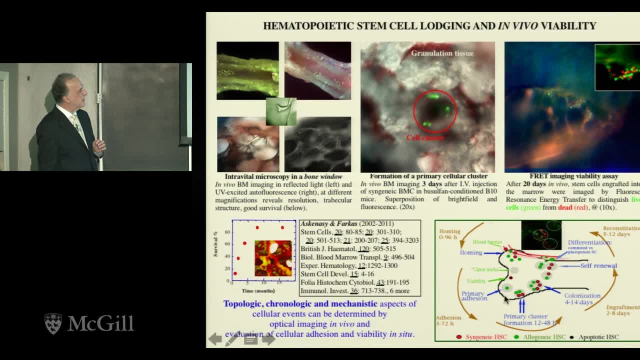 If you are able to do this sort of tracking, you can start putting together, putting together a story of what happens in terms of sequence, as the hematopoietic stem cells go about their work in the bone marrow, And so this kind of work is done now at Mass. 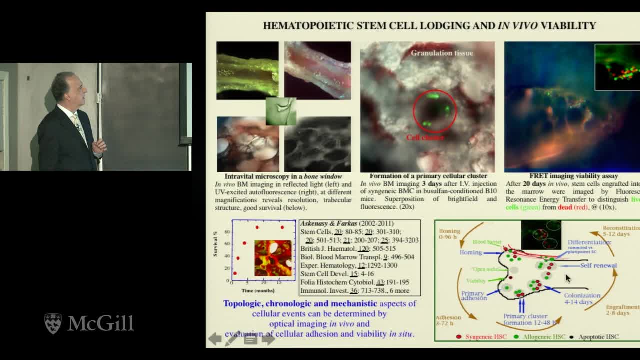 General and the Wellman labs and they have done fantastic enhancements to the approach and they can monitor stem cells live very convincingly. You can also look at dendritic cells, which are kind of the cleanup immunological cells of the body and that's pretty exciting. I don't have time to tell you this story, but 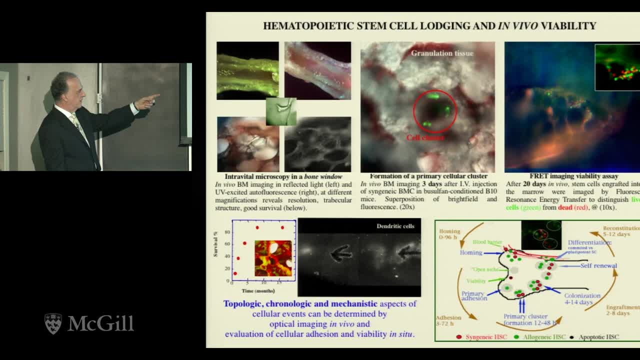 basically the stem cells, the dendritic cells, thought that the marker arrow that we put just to find the locus where we injected them is something that is deleterious to the animal, so they were basically eating it up while we were going and taking a ten minute break. 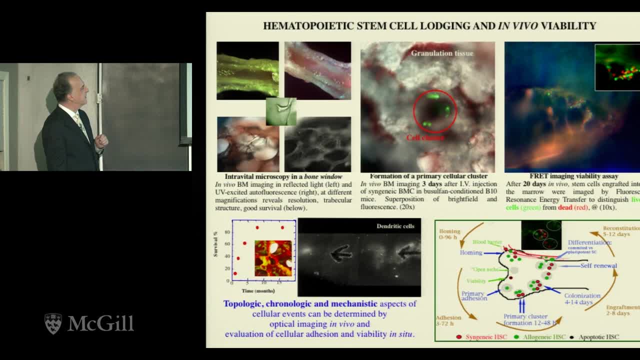 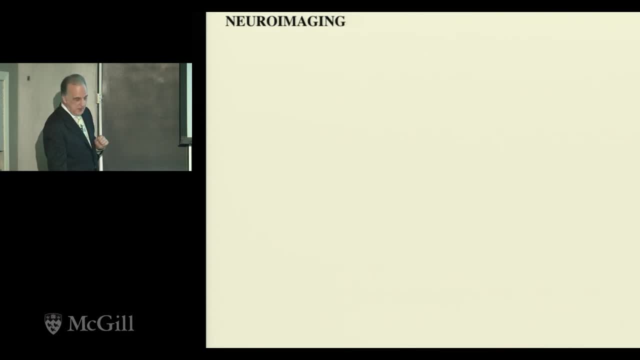 So that was interesting to see- that the chemistry triggers the dendritic cells. So you can put together the topology and you can put together the mechanism. Subtitles by the Amaraorg community. Okay, so let's move on to neuroimaging. I don't know whether you recognize this gentleman. 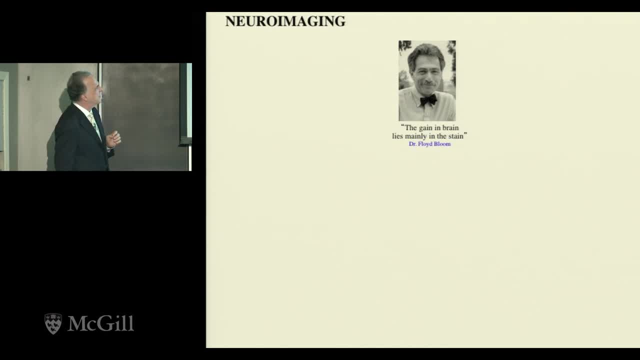 He used to be the editor in chief of Science Magazine. He's a really illustrious neuroscientist, Floyd Bloom, And he tells us that the gain in brain lies mainly in the stain. So he's not happy with the level of progress and the kind of progress that is being made. The reason: 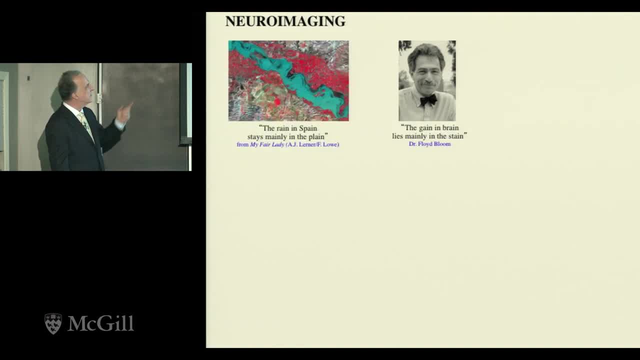 that that sounds like something familiar is because of this. The original quote is: the rain in space stays mainly in the stain, It's mainly in the plane, And that's what happens actually by hyperspectral imaging. when the rain in space stays mainly in the plane, The massive flooding is induced And 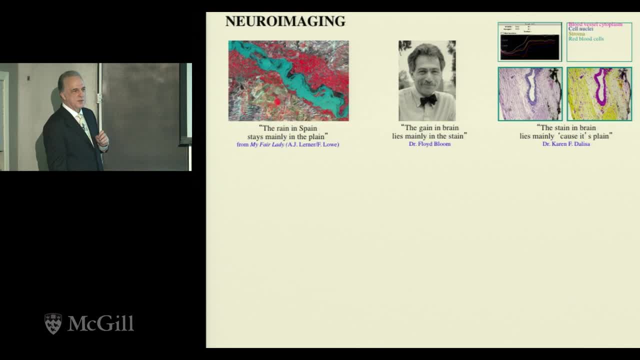 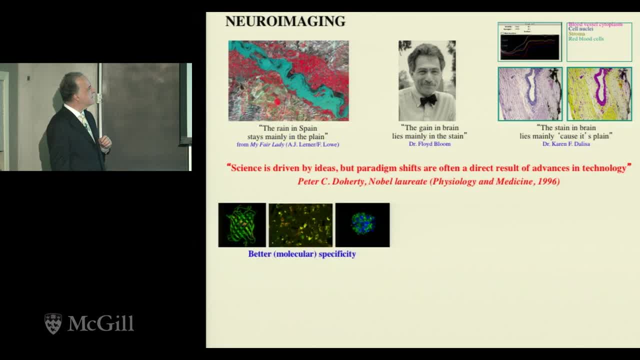 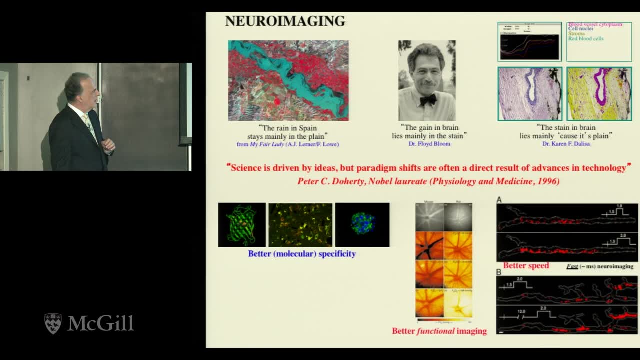 improvements in technology. This is what Peter Doherty is telling us. So what would be better? Well, better molecule specificity would be better, better functional imaging, better speed and better places and ways to look. So I'm going to illustrate, not the top one. 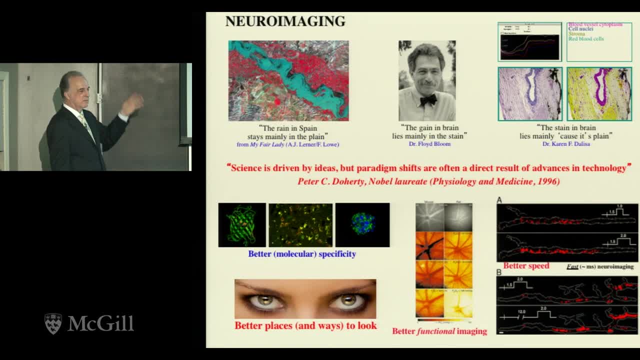 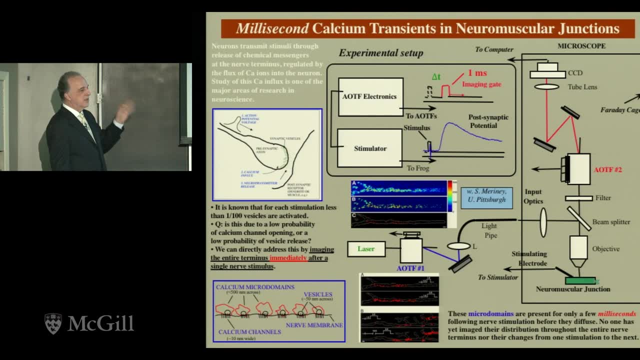 because that was done extremely impressively by people like Roger Chen And Nobel prizes were given out. I'm going to look quickly at the other three. So the first one: speed With the acousto-optic turnover filters. remember, there's no moving parts. therefore you can have very, very fast imaging. 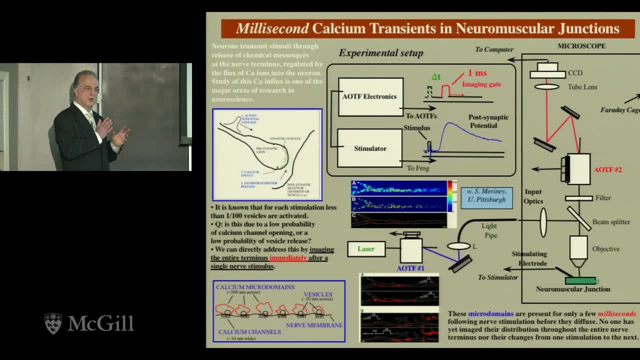 So we were able to look at sub-millisecond temporal resolution imaging at a neuromuscular junction and look at what is happening to the calcium domains that are firing upon neural excitation, And with this microscope that had both the temporal and the spectral acquisition driven by acousto-optic turnover filters. 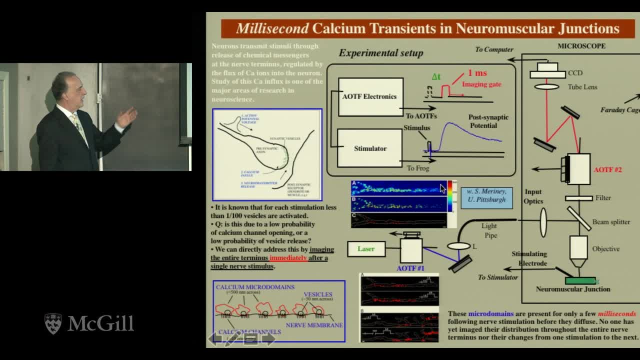 we were able to look at sub-millisecond scale, at the very primary events, And think about it. in typical neurosciences, to this day, the standard for speed is video rate. By the time the first video frame comes around, everything is delocalized. 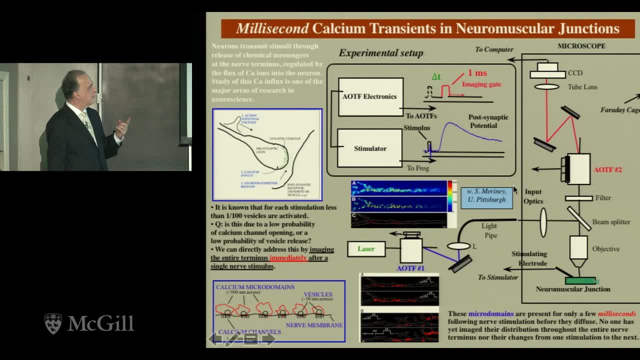 So if you want to look at discrete events, you better have resolution of the order of a millisecond or better. So we were able to have that and you can see here that at this neuromuscular junction even one millisecond makes a difference in terms of how things look like. 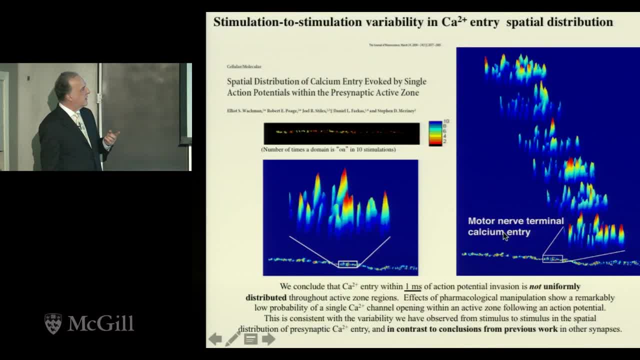 And if you fire consecutively on that neuromuscular junction, you can see that on every firing a different set of domains comes on, which was totally the opposite of what the dogma was in the field at the time, and so therefore it made it a little bit more difficult to publish. 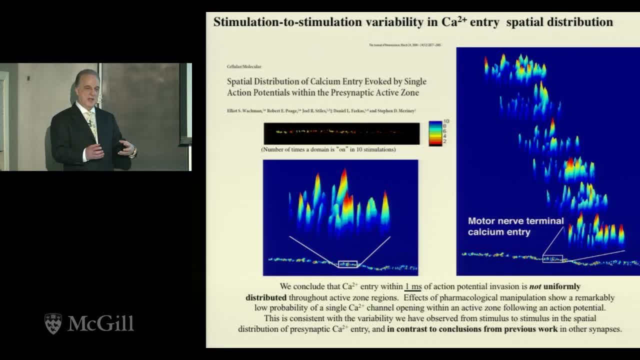 But it makes sense biologically because what you want is some redundancy so that if there's some sort of functional or structural damage, that you would still have a reasonably functional neuromuscular junction, And so this had a lot of modeling also that went into an appendix. 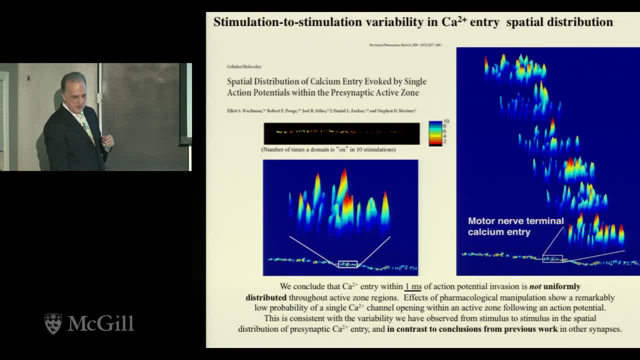 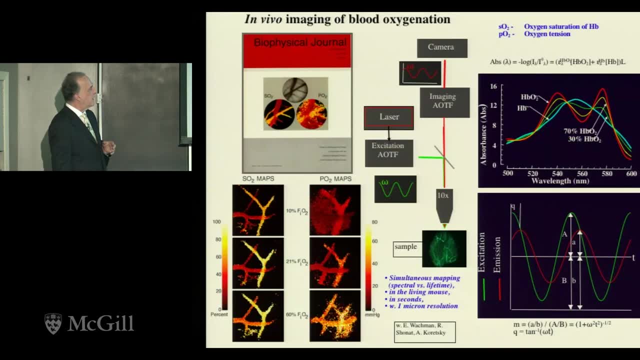 that was done with the Pittsburgh Supercomputing Center and they made us jump through hoops to publish this, But speed was a very good thing to add to the capabilities. Okay, still with an acoustic optic microscope in which you can also do spectral and temporal control. 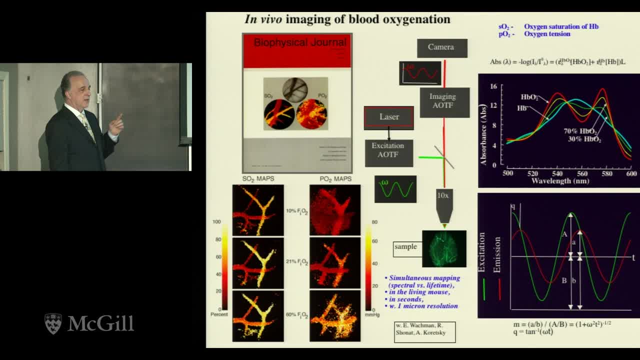 we were looking in living animals in the brain, at two things: oxygen saturation of hemoglobin and oxygen tension. Oxygen saturation of hemoglobin is pretty easy to understand, so basically in the spectrum in between 500 and 600 and again around 800,. 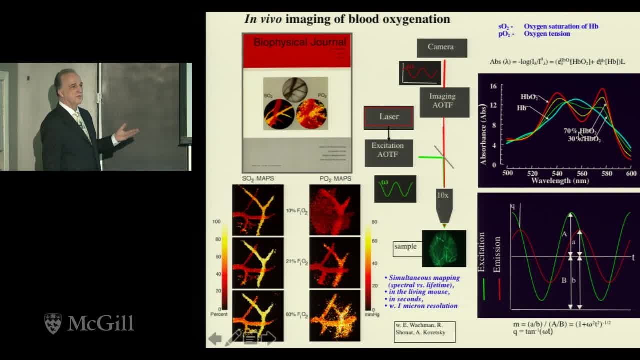 there's very clear spectral changes upon changing oxygenation from oxygenated to deoxygenated. So we could map in the brain of a living animal and tell arteries and veins apart and have the animal breathe different levels of oxygen: normoxic, hypoxic and hypoxic. 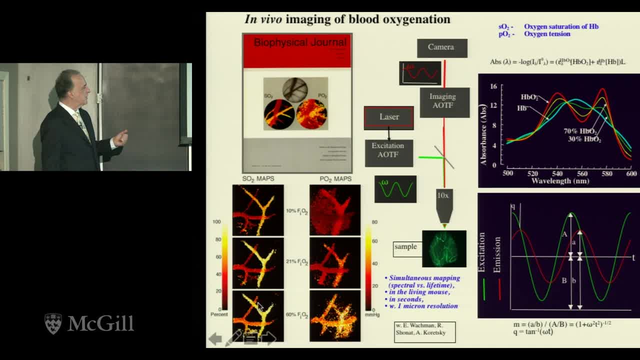 And see how the changes are induced. What is much more difficult to do is to look at oxygen tension. So most current experimentation that will tell you that they measure oxygen tension, they actually measure oxygen saturation and assume that the two are connected by a sigmoidal curve. 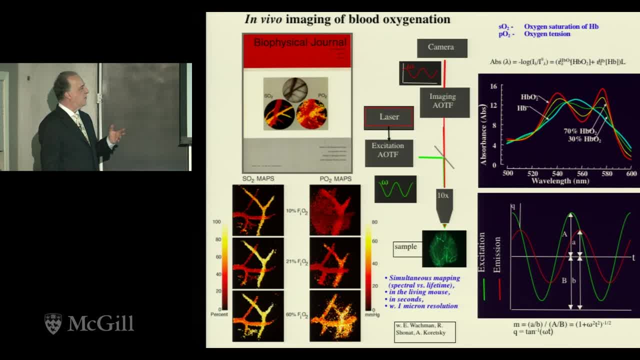 that never changes. It turns out that it changes even from strain of mice to other strain of mice. But we were able to map both of those in the timeframe of about a second or two and see the changes in oxygen tension as well as oxygen saturation. 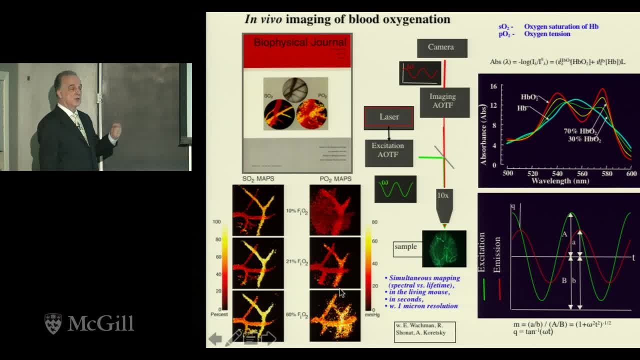 The way that this is done is by lifetime of phosphorescence. Phosphorescence is quenched by oxygen, So there was beautiful work done, mostly at the University of Pennsylvania in Philadelphia, developing these probes that allowed you to go from full oxygen to practically zero oxygen. 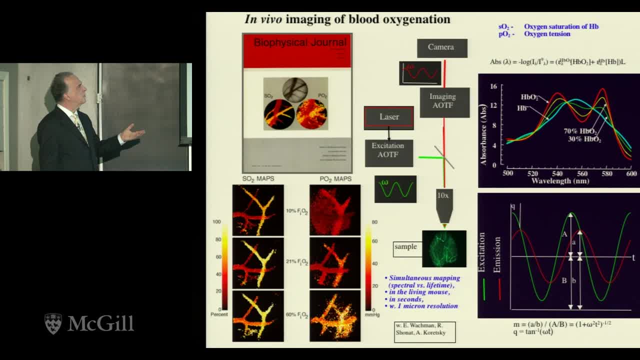 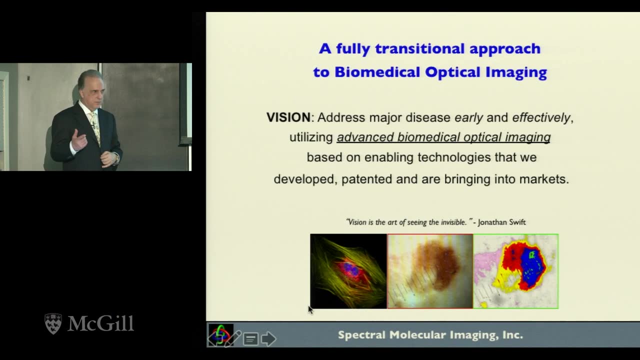 by changing phosphorescence lifetime from 200 microseconds to 2 milliseconds. So with the speed of the AOTS we were able to map those and come up with maps like this. Okay, so, having covered that, I hope I can go on a little bit. 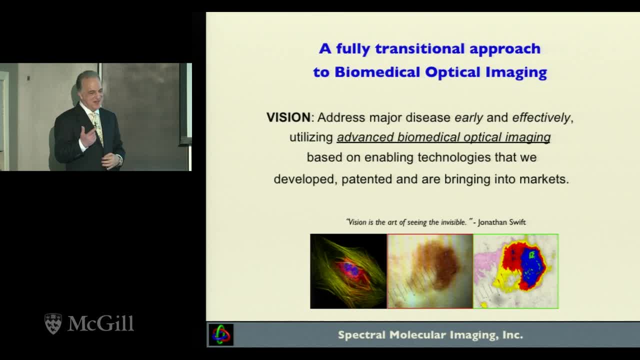 because I have a lot of, I'll start skipping some. But how do we try to bring all of this to the clinic? Okay, so we would like to bring advanced biomedical imaging to the clinic. So we have a strategy: identify major needs and try. 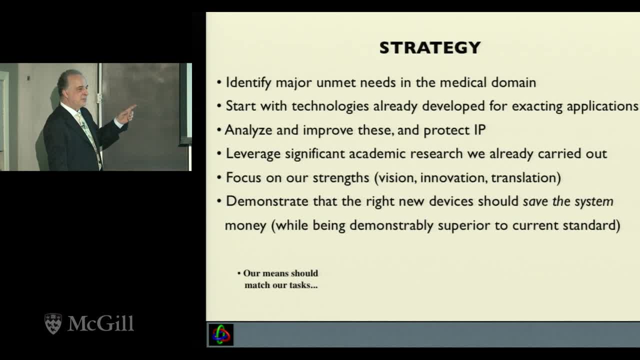 to apply the best things that we have found to it. But the main methodological point I'd like to make is that our means should match our tasks- unlike here, And the other conclusion is that strategy is even more important than technology, as illustrated here. 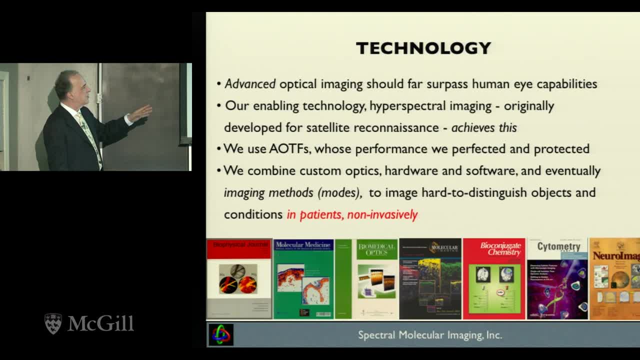 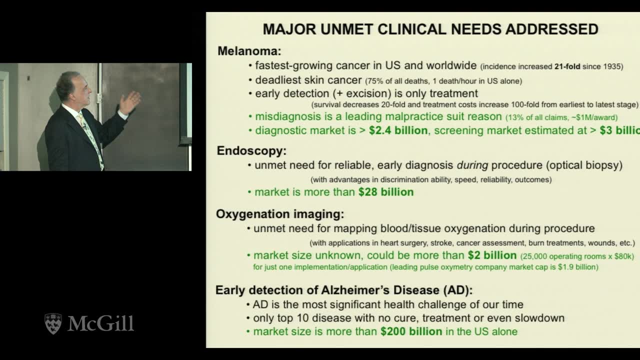 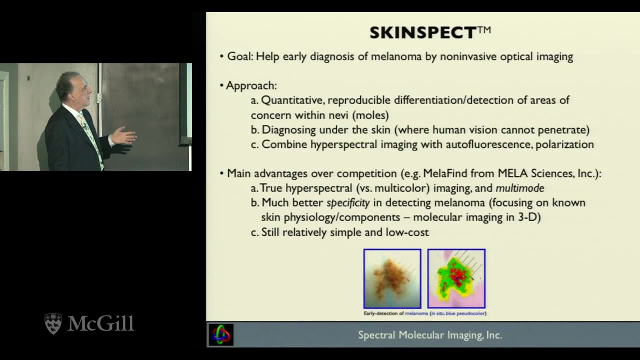 So I told you about some of the technologies that are published. Let's take on some difficult problems: melanoma, better endoscopy oxygenation, imaging for things like burns and wounds and such and early detection of Alzheimer's. We developed a device called SkinSpect that we applied. 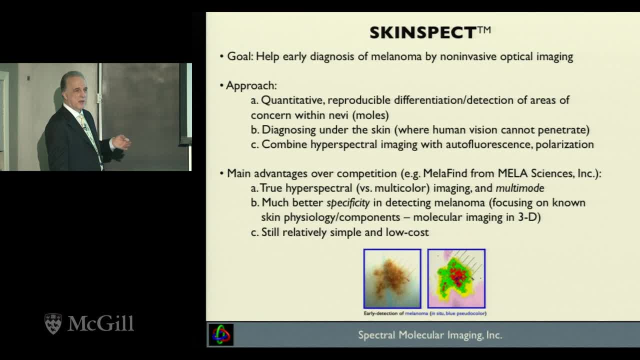 to originally to early detection of melanoma, in which case the clinical scenario is very pleasant. It's 99% cure. If you find it late, it's very low percentage of cure. Main advantages is that we are trying to map everything that is. 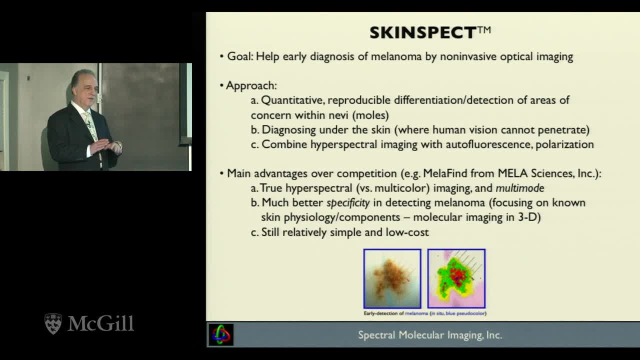 of relevance in the skin in 3D quantitatively, even if they sit on top of each other, which they do like melanin and Oxy and Deoxy hemoglobin and collagen, As opposed to other systems in the literature in which they are basically trying to develop an expert system. 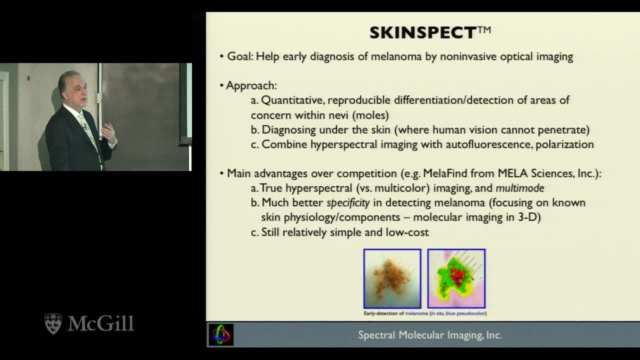 and only be able to look at melanoma. And even with melanoma, the more data you get, the worse the system performance gets. In our case, we build libraries, we build better understanding, so therefore, the better the system performance gets. 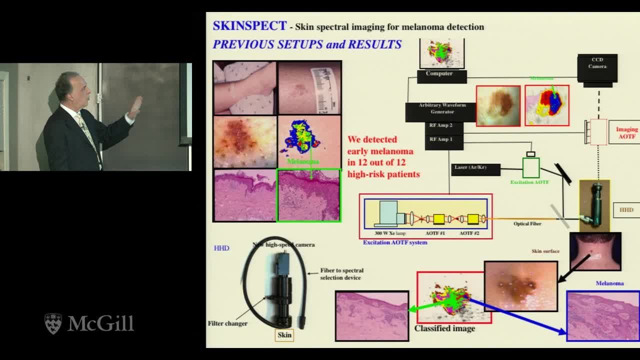 This was early work on 12 volunteers only with spectral imaging, and we were able to find in 12 out of 12 very early melanoma arising in those moles that were going to be removed. anyway, This was done in Pittsburgh and I'm not going to dwell too much on it. 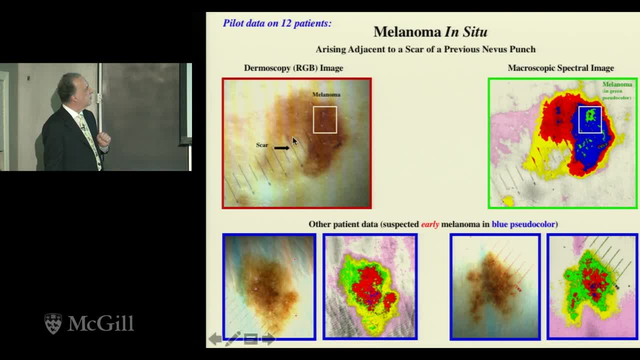 But I'll show you one particularly unpleasant example in which this patient had an ugly mole. He went to a community hospital and they removed it by punch biopsy And a couple of months later the mole started growing again. the pigmented nevus and early melanoma was growing in it. 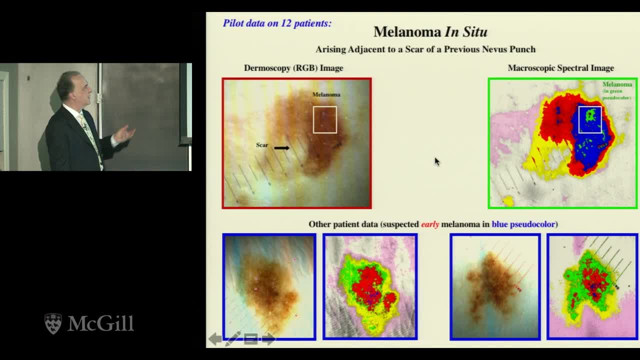 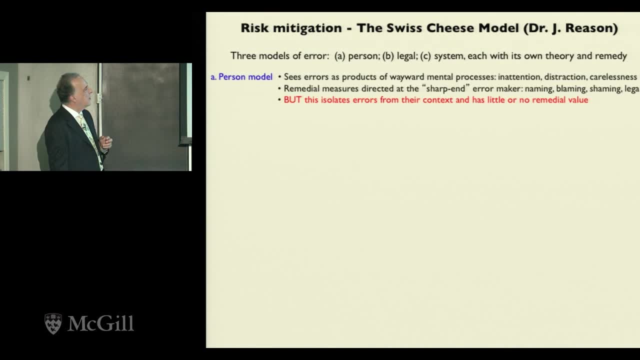 And so it would be nice to be able to always find what needs to come off and how much spatially. So a very brief detour into risk mitigation. I don't know whether you know, but in the United States at least, medical errors have jumped. 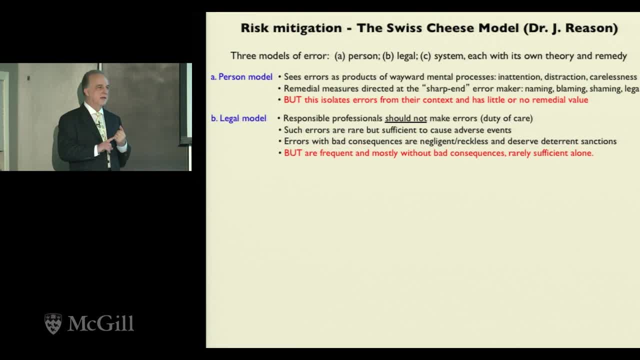 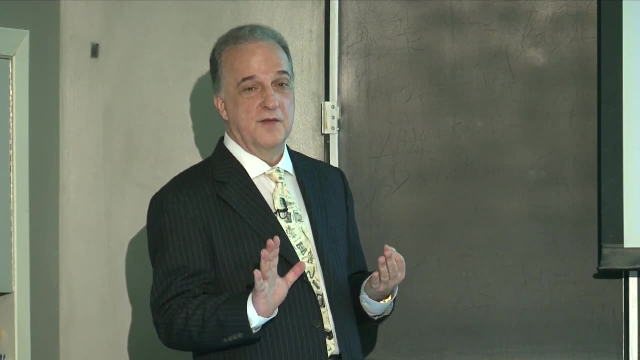 to number three in cause of death. So it's cancer, cardiovascular medical errors. It's staggering and probably underreported. So if you look at other fields of human endeavor where there's risk, this is equivalent to five large planes falling out of the sky every day. 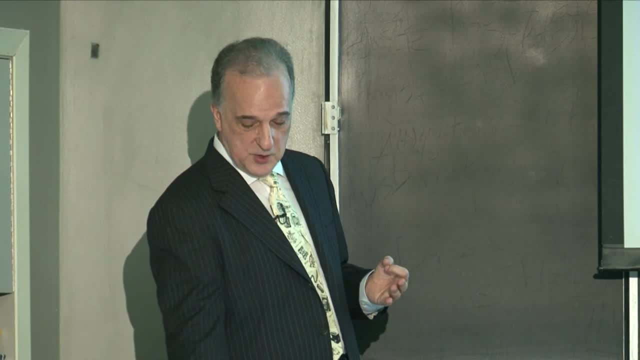 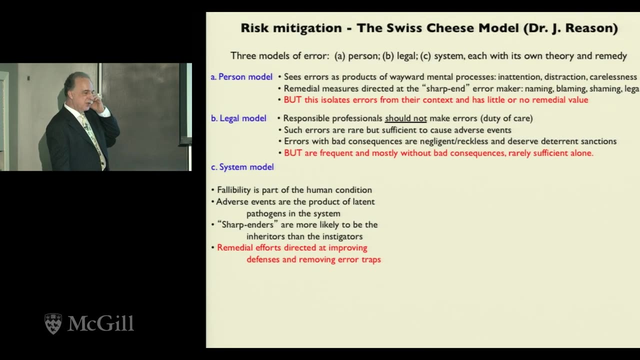 So maybe other fields of human endeavor have figured out a few things about risk mitigation. So I started reading this literature and found out. of all the models, I found one that I liked. It's by a British gentleman, probably a curmudgeon. 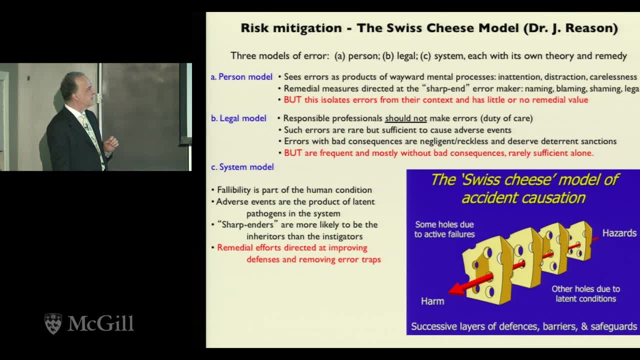 that is, believe it or not, his name is Dr Reason. So Dr Reason says: okay, here's a hazard, here's you, You're trying to do something about this. so therefore, you're interposing something between the hazard and yourself. 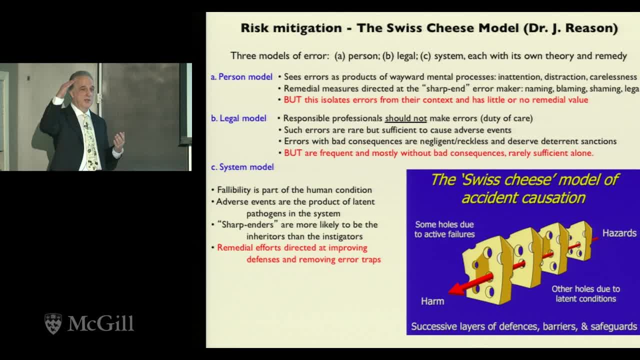 However, we are human. everything we do is flawed. so, therefore, what you're interposing is like a slice of Swiss cheese: it has holes in it, and the bad thing can hit you through the holes. So what's the most logical thing to do? 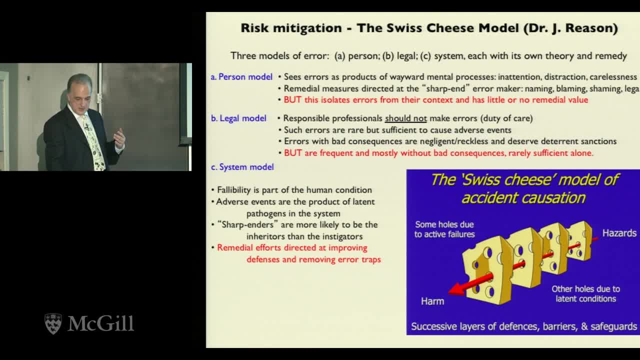 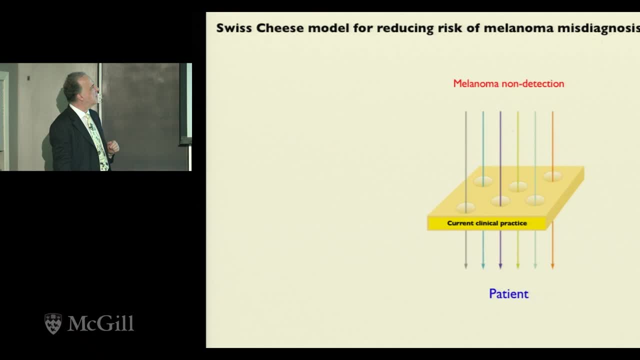 Put a couple of slices of cheese because the holes don't align. So that to us is basically saying: do multi-mode imaging Right? So here's current melanoma detection and you can hit the patient in multiple different ways. If you stack the slices, it's less likely. 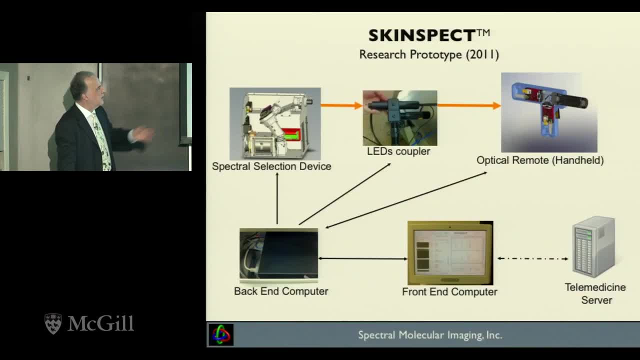 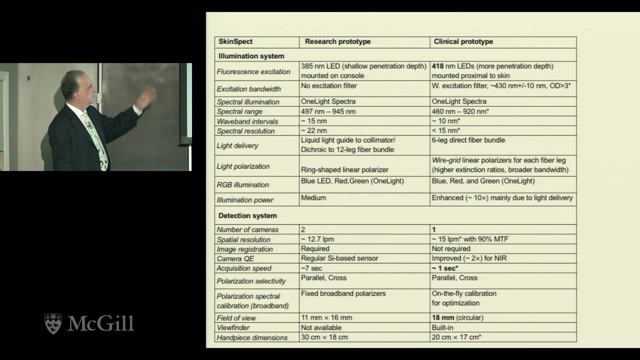 that you're going to miss something. So we started building this device. It's a handheld with a cart with full spectral capabilities, but with several other methods that we put on it: Polarization, control, autofluorescence. We had iterations. The more we go, the more the system gets better and slimmer. 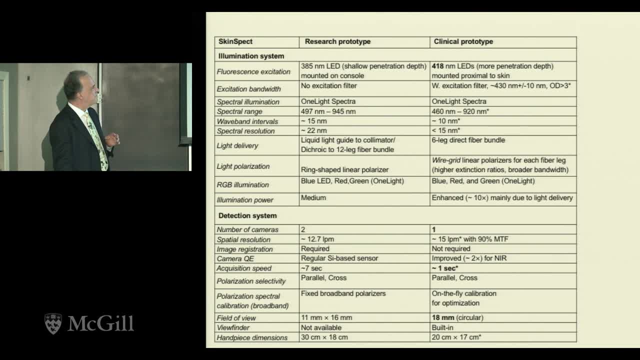 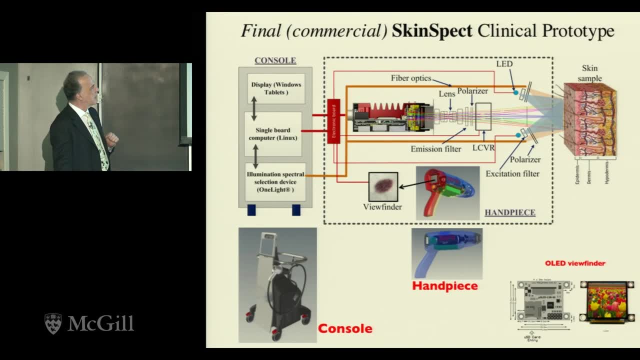 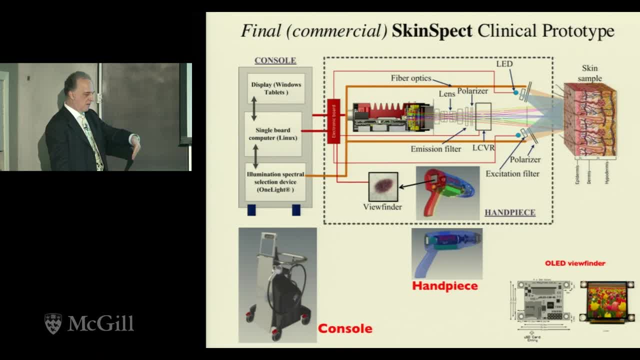 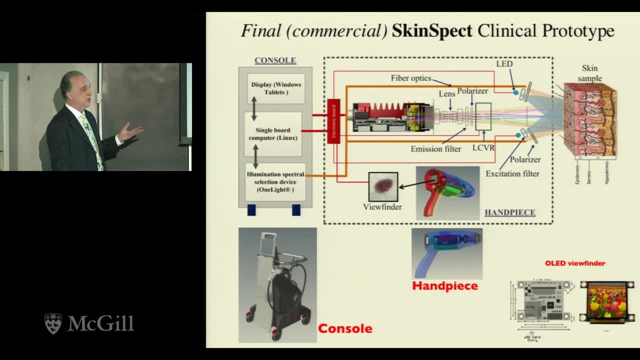 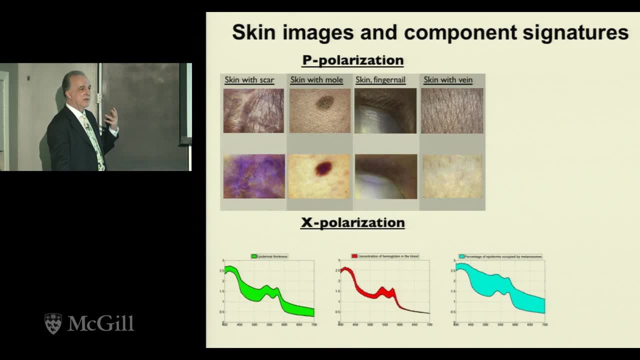 And you basically get about 100 plus images- actually 106 images- And of course you have to process them. And polarization is important because you don't want to look at the light that just gets specularly reflected, that contains no information. So this is work mostly by Dr Fartash Rasefi, who's actually 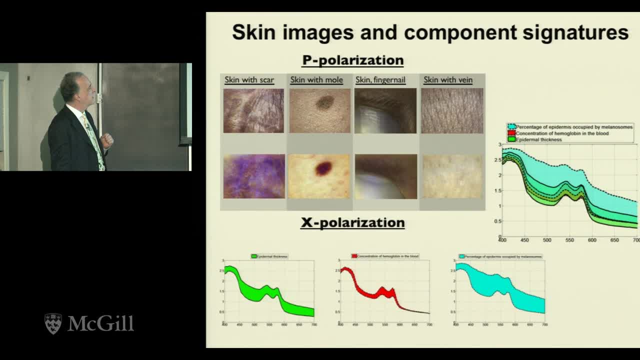 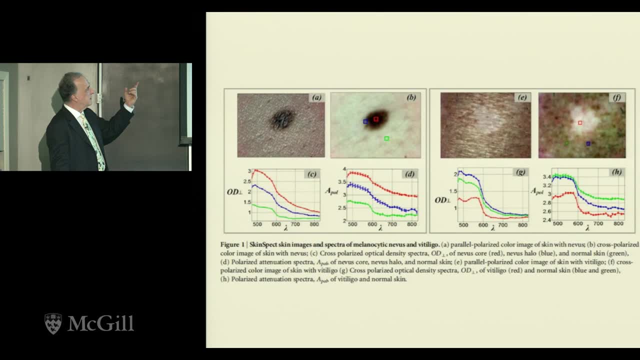 in the audience here and has been working with me for a number of years. It's published in actually multiple papers. I'm not going to dwell on the details, But basically you can look at either darker things than the skin, such as moles, nevi or psoriasis or anything else. 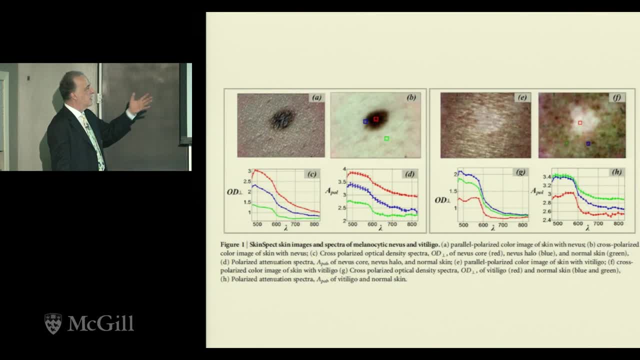 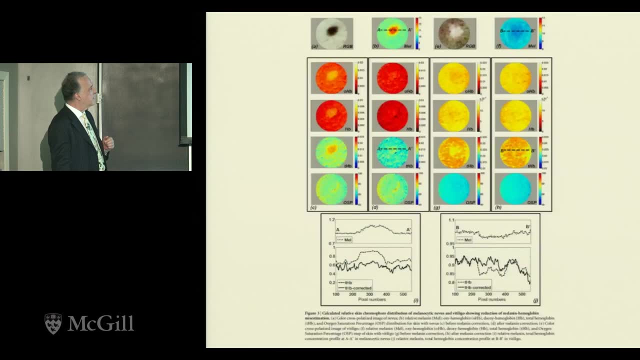 And you can map quantitatively these various components of the skin that are sitting on top of each other and under the surface, So the human eye cannot penetrate. The human eye cannot go into the near infrared. So it's useful. And then you find out that there's a lot of data. 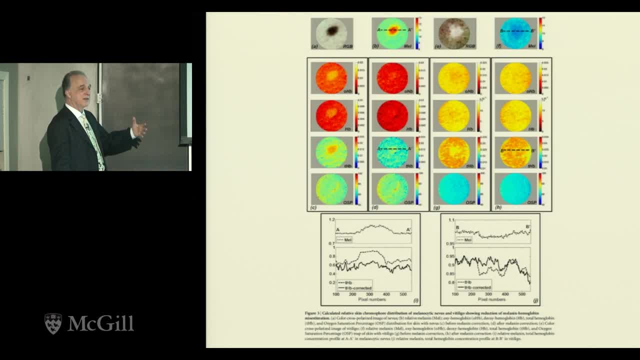 in the literature that, basically because they didn't have all of the wavelengths necessary to do the discrimination, they're coming to the wrong conclusions because the melanoma, the melanin images, are affected by the presence of oxy and deoxyhemoglobin and the other way around. 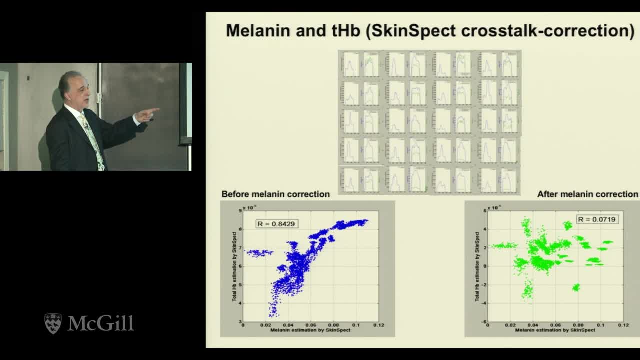 And so we developed a method by which a correction can be induced. So you can see that if you don't do the correction spectrally there's very high correlation between the hemoglobin and oxygenation and melanin. But once you do the correction, 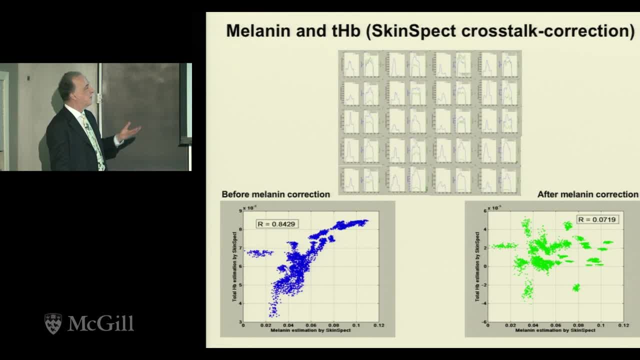 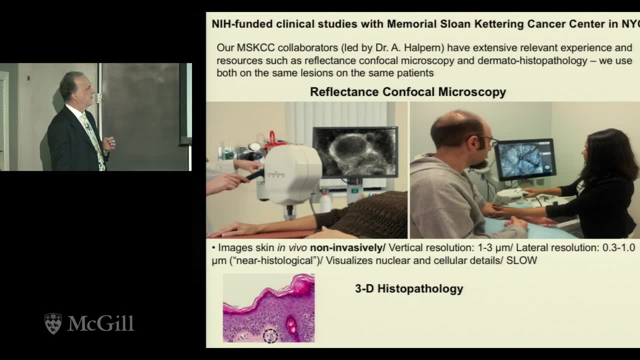 there's practically no correlation whatsoever. Therefore, you are confident that you are mapping all of them. We have a couple of very nice clinical collaborations at University of California, Irvine, and at Memorial Sloan-Kettering. The beauty of these places is that they have pretty much every other method known to man. 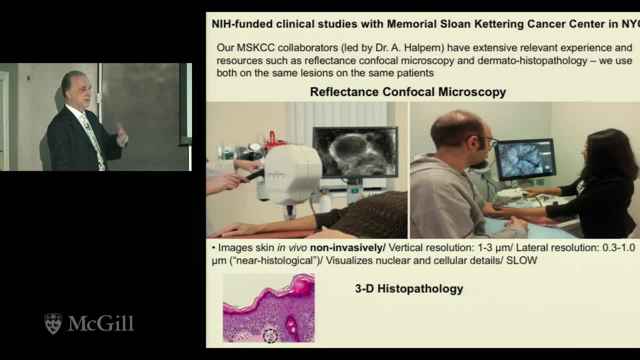 to look at the skin. So therefore, we can always compare our results with not only histopathology but also other methods such as, in this case, 3D histopathology done by confocal microscopy at Sloan-Kettering. This is a pretty ugly picture, but it's a pretty good picture. 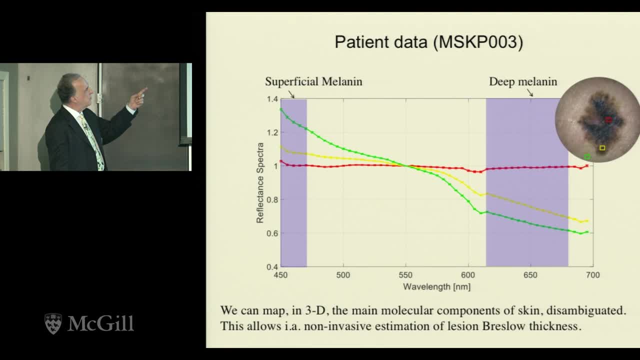 This is basically melanoma. You can see that you can map both superficial melanin and deep melanin with our method And you can deduce certain things such as the so-called Breslau thickness, which is very indicative of the evolution of the disease. 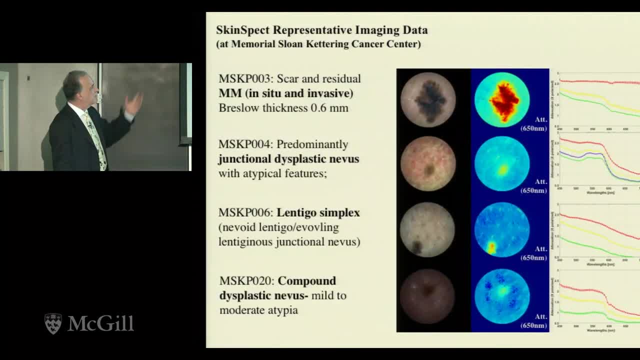 and what stage the melanoma is. You can tell melanoma from dysplastic nevi, from lentigo simplex and from compound dysplastic nevi just by not just imaging but quantitating that imaging On the right-hand side. 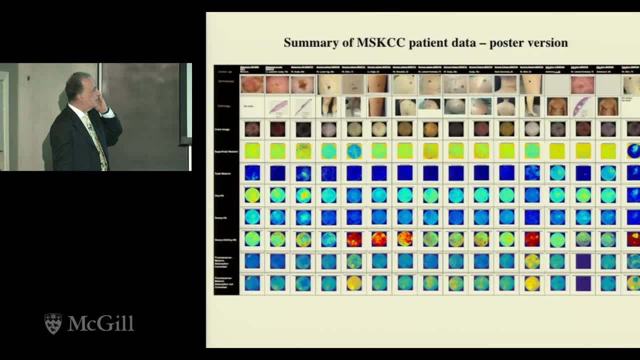 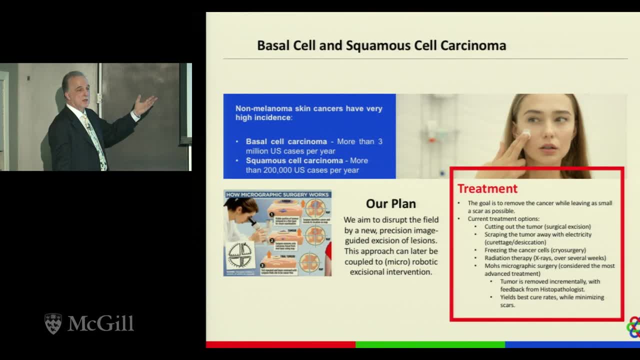 As I said, we have lots of correlated measurements, as shown here, And of course, you can use it for anything else in the skin, such as basal cell and squamous cell carcinoma, which have much higher incidence than melanoma. They are not the killers that melanoma is. 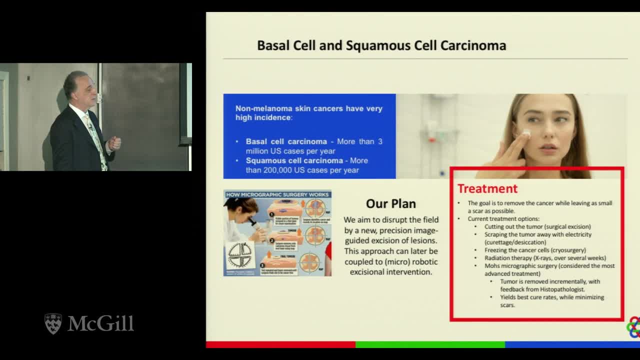 But the way that they are done today, by iterative hacking called most microscopic surgery, is not the best way to do it. So, if you can outline, put a dotted line around where you would need to cut, especially because these things are mostly on the face. 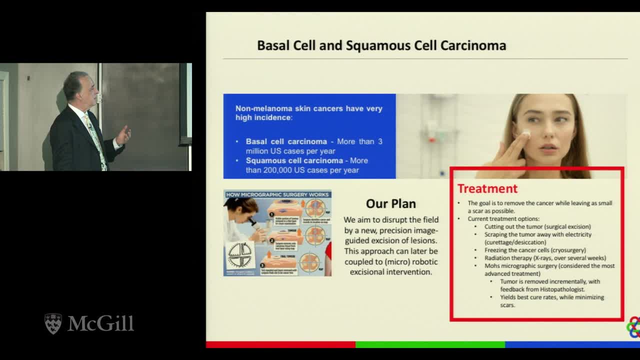 you can do that. You can have a much better image-guided intervention and possibly you can do it by robotic approaches. You can also use it for cosmetic purposes. I didn't bring slides about that, But you can tell that you can look at anything before. 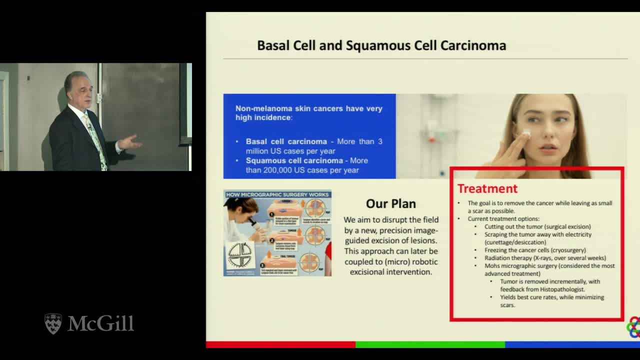 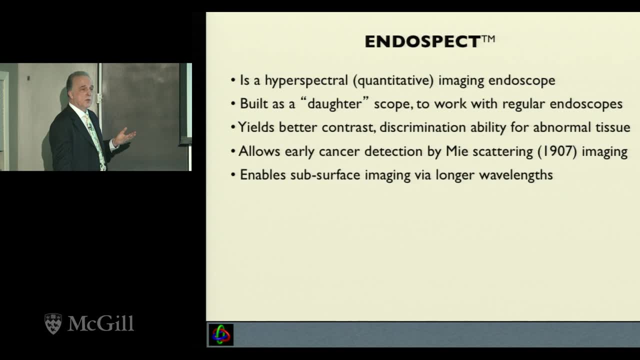 and after and see how well anything works. You can use it for burns, You can use it for wounds, You can use it for things of that sort. Let's move to endoscopy. The best places, by the way, to look optically are first outside. 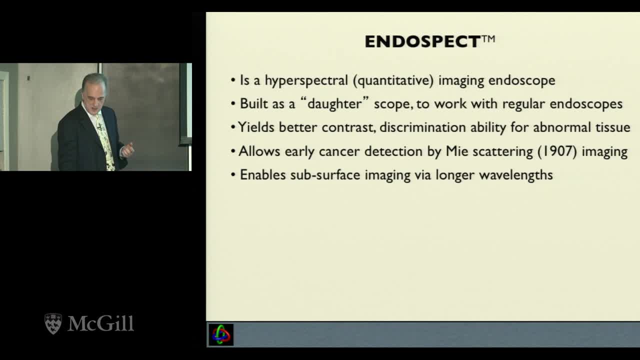 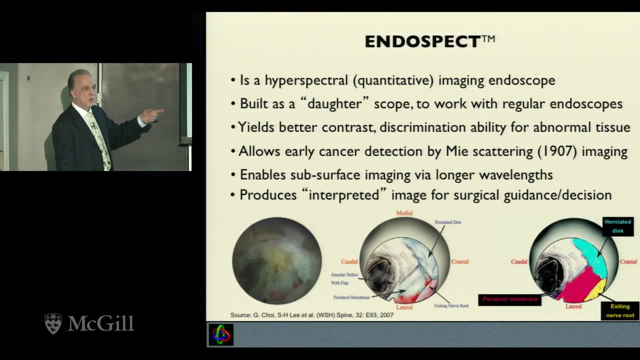 of the body, which is the skin, then at the tip of an endoscope and then in the eye. So let's move to endoscopy. So can you build a hyperspectral endoscope And basically, as you go around and do your endoscopy. 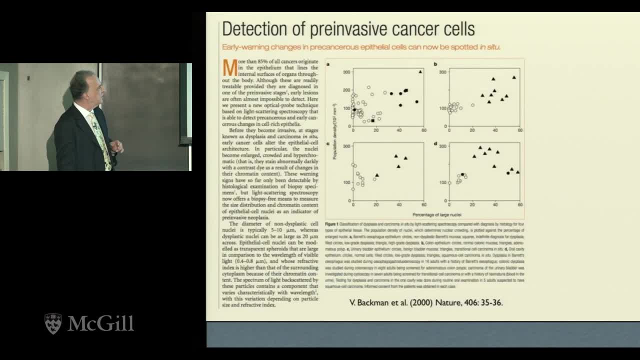 know what to touch and what not to touch, know what to remove and what not to remove. There was an early paper in 2000 by a Harvard MIT collaboration led by Vadim Bakman. This was with Dr Feld who unfortunately is not. 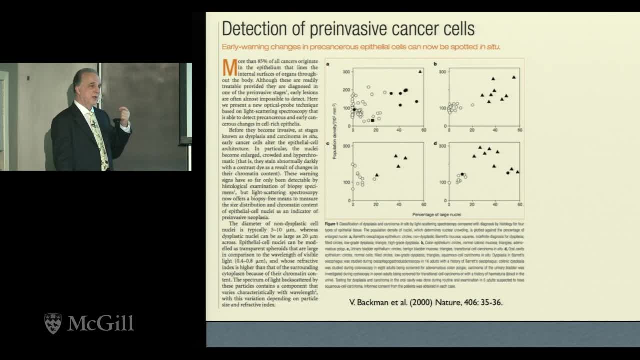 with us anymore in which they did a spectrally-based mean scattering detection of GI cancers And it was a very impressive paper in Nature with a single figure and basically saying: this is cancer, this is not cancer, based on just the spectral signature. 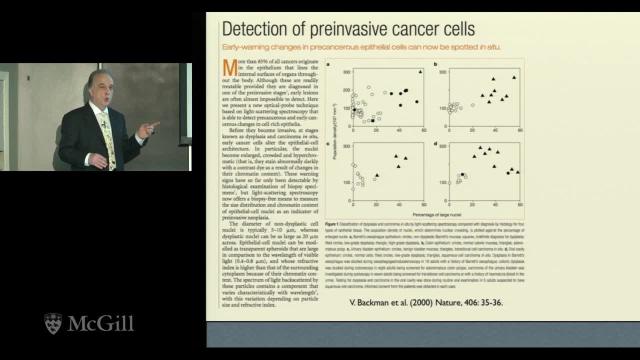 The theory was given by Gustave Mey in December of 1907, and it tells you that if you put light down on something and the light scattered back, basically a spectral oscillations that depend on nothing else but the size of the scatterers. 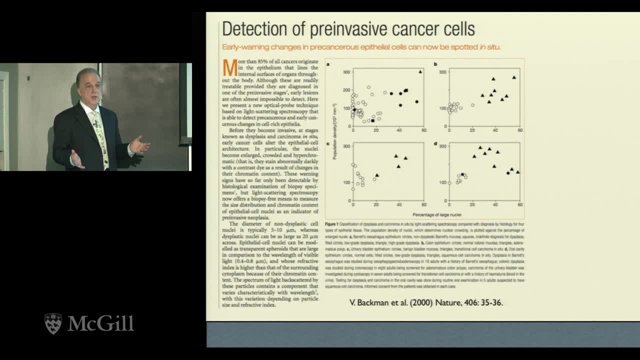 The only scatterers in the tissue, in human tissue of note, are the nuclei. So if the nuclei are slightly enlarged, such as in dysplasia, and certainly, as in cancer, much enlarged, you can tell without having that actual resolution, because mean scattering is basically able. 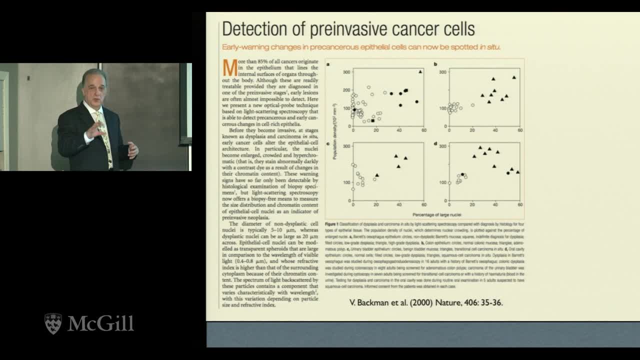 to give you a little elevation map, like maps of what the nuclei are enlarged. This one was not done like that, This one point measurements. So basically you had to come with your endoscope that actually touched the GI from the inside, the GI tract. 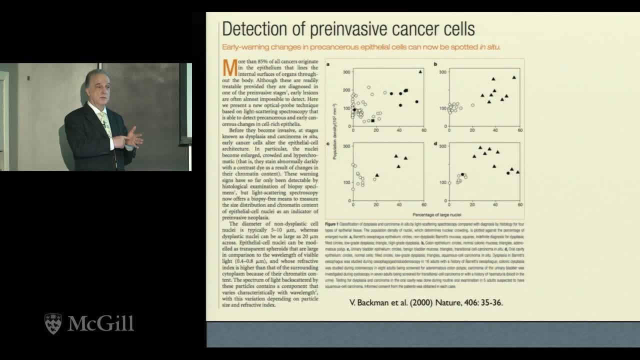 and have to get multiple points in order to get your measurement. The reason I think that this was not followed up on is because the surgeons don't want to have to touch in 100 places or 200 places, So what's logical to do is to pull back and instead. 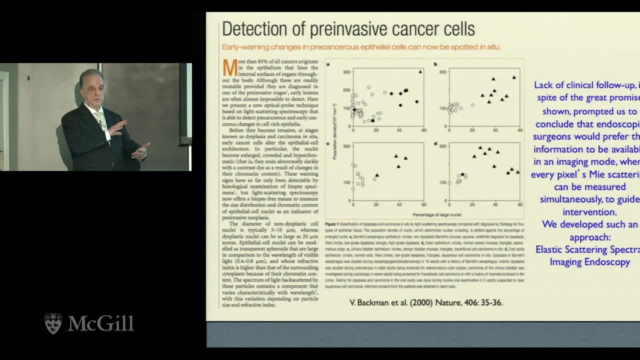 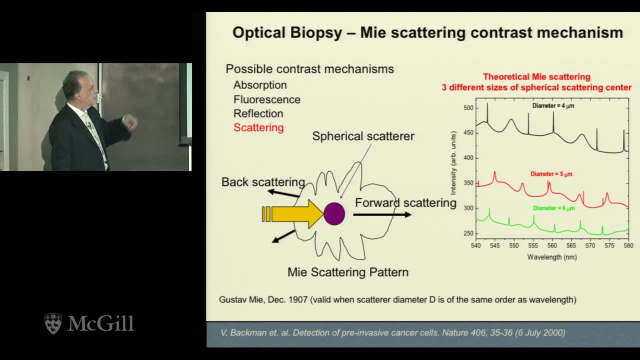 of doing it one point at a time, have full hyperspectral imaging of the endoscopic field of view and try to do mean scattering in that way. So the theory, as I said, is well understood. We built a hyperspectral endoscope to look. 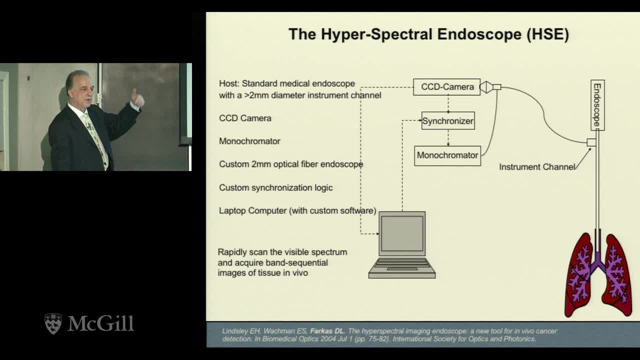 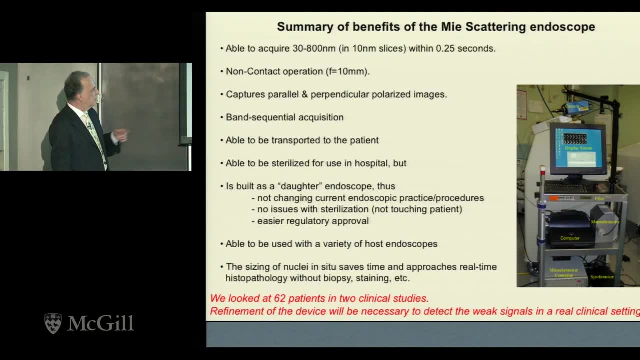 at this sort of scattering. We actually built it as skinny enough that it could fit into the instrument channel of an existing endoscope, so therefore you don't have to change your procedures. Looked at 62 pages And basically we saw that it's deployable in the clinic. 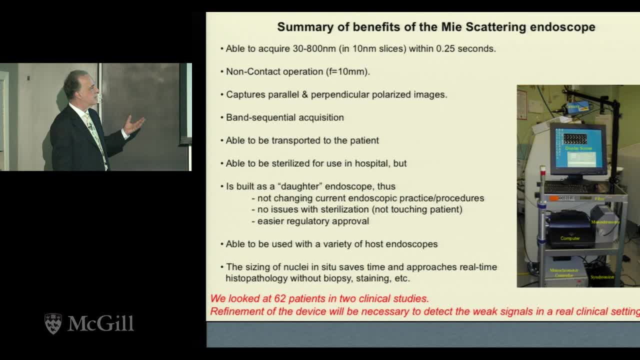 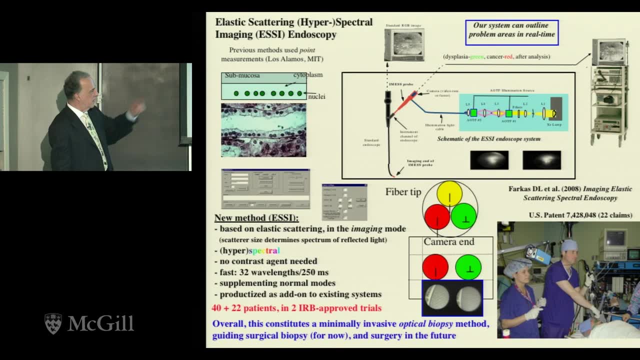 but that the quality of the results is not that great because we didn't have quite the spectral resolution that you need. So these are some of the results. That's how the endoscope looks like. So there are two fibers on the camera end and three. 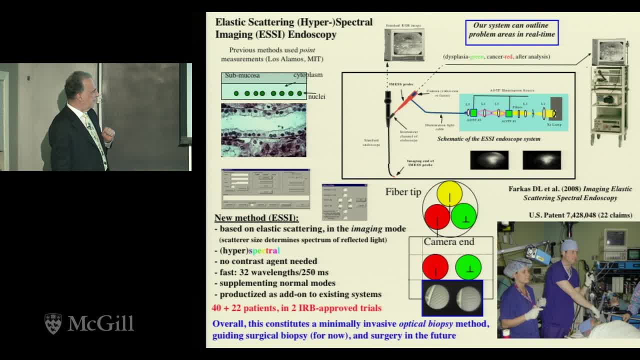 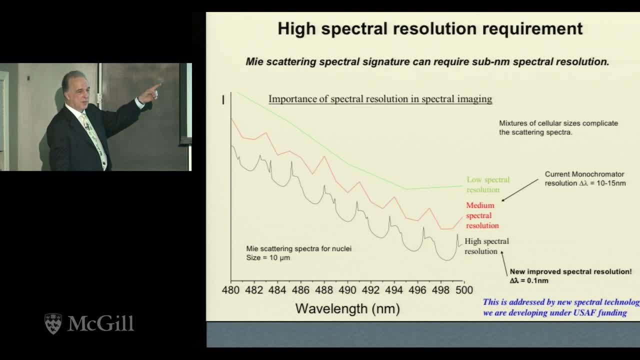 on the tip for excitation, We can get all the data in 250 milliseconds. but here's the main point: If you take something off the shelf, you get the green line on top- very poor spectral resolution If you get a reasonably good spectral resolution. 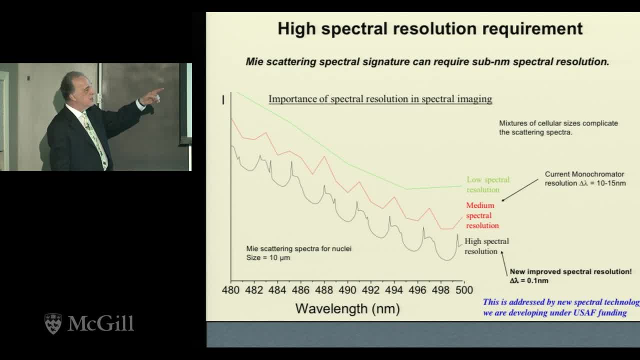 such as with the acoustic optic thermal filters, you can start seeing the oscillations, But if you can get something, such as the spectral technologies that we are developing under Air Force funding and that I'm not going to talk about, you have sub-nanometer resolution. 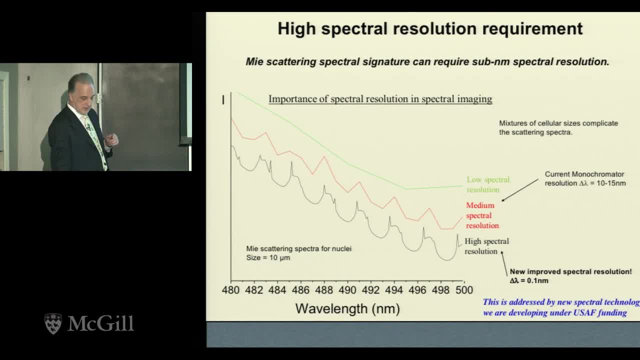 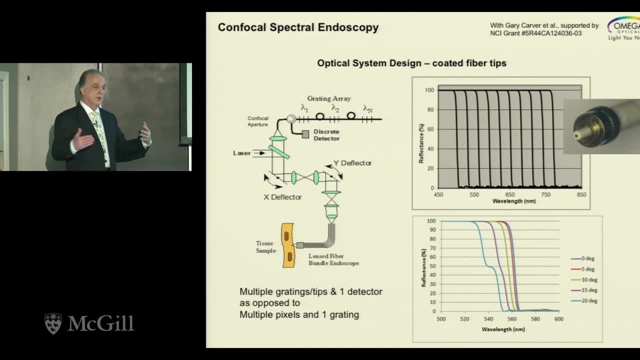 you can start seeing very nicely the mean scattering peaks And with that you can say how big are the nuclei in the region that you're looking at. Another way to go with endoscopy is remember. I want to connect detection and the endoscope. 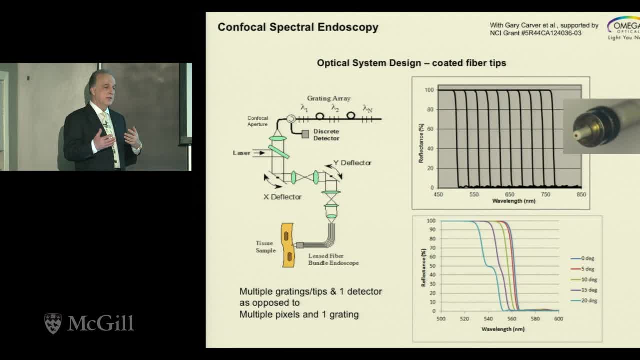 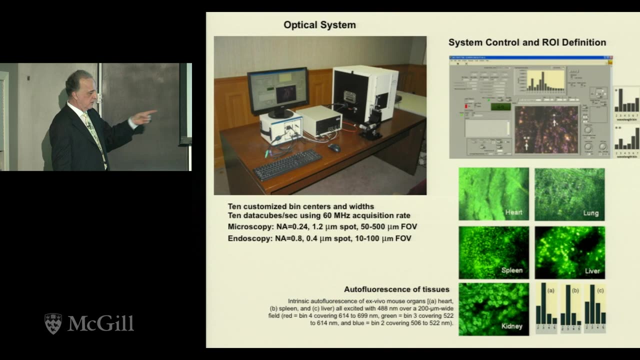 Treatment. Another way to do hyperspectral is to do it at every location and do it in a scanning confocal mode. So this was done with Gary Carver in collaboration And what we built is an endoscope that was spectral and confocal scanning. 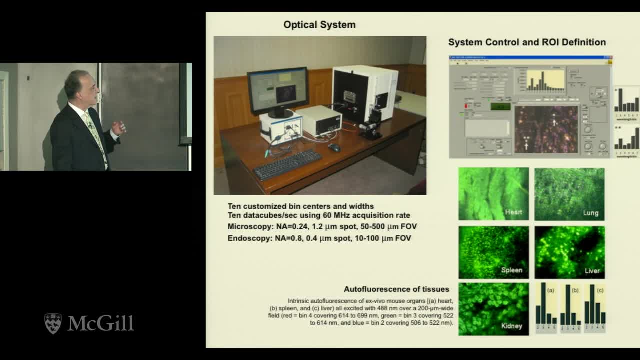 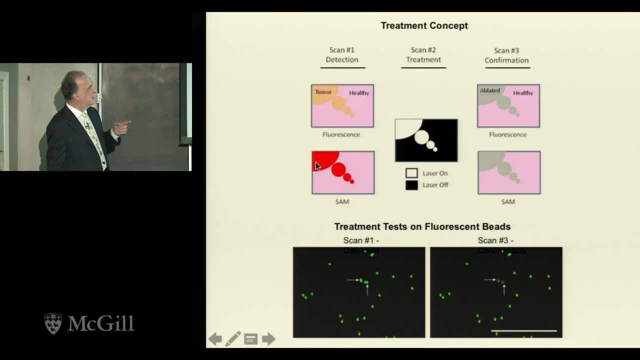 You could look at autofluorescence- very high signals, healthy signals- But the point that we built it for is this: You can decide what it is that you don't want there, such as cancer, And then, as you have taken the image, 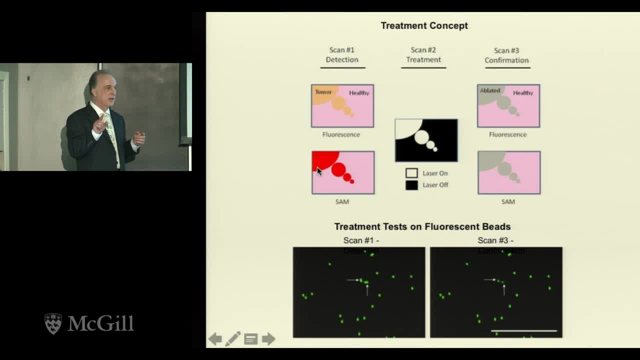 by having touched every point, every pixel, you come back with a bigger laser and just fire it over the points that you would like to remove. So this is really surgical intervention. So we show that it works here for beads- fluorescent beads- and then for tissue. 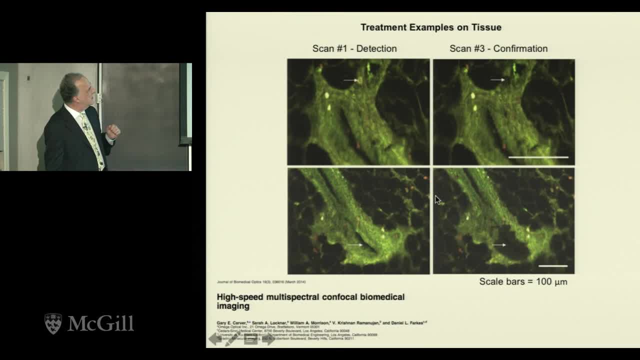 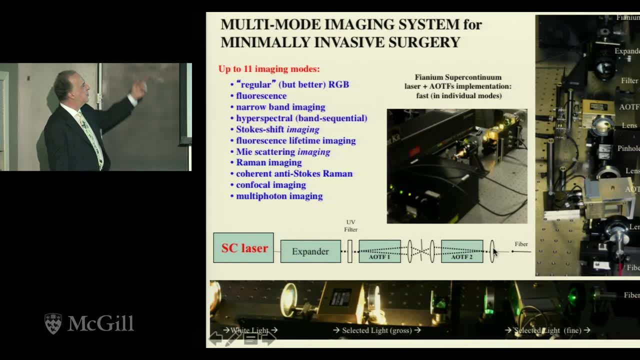 You can see here that we remove this and we remove this And again, this was published. OK, Eventually you can put all this together. You can put all your multimode modes onto an endoscope. So this was a very fancy endoscope. 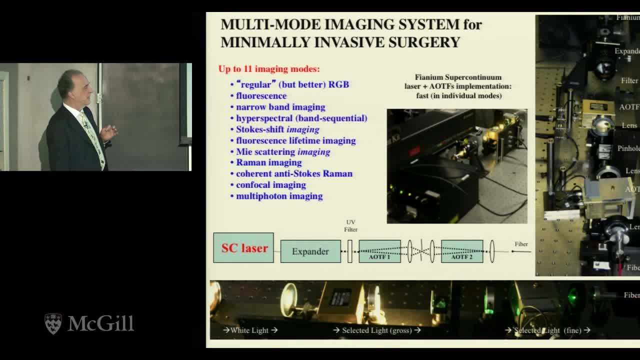 that we ended up building at Cedars-Sinai in circa 2008,- 2009.. And you start to worry about how are these things going to be deployed in the clinic? Well, you need a new kind of operating room in which you can just roll something in and connect it. 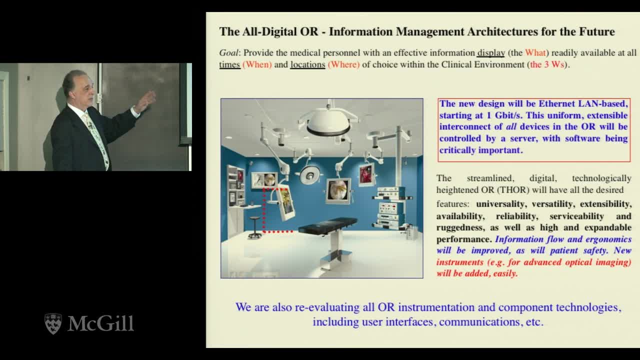 So we developed an operating room of the future. Doesn't look like this, unfortunately, But conceptually it looks like this: that anything that has an internet connection can play a role in this kind of operation. that is already in the room, OK. 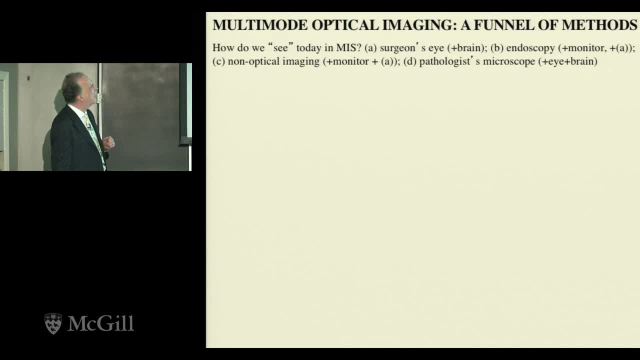 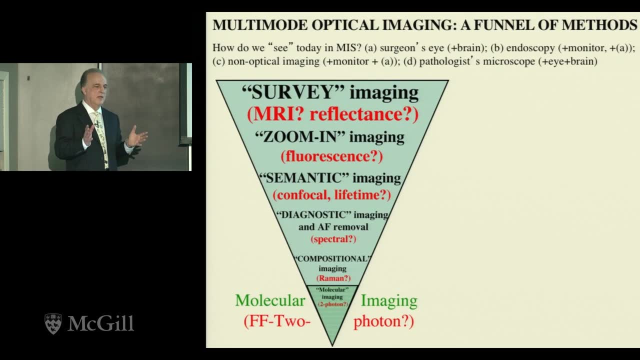 Quickly now. The multimode approach that we are proposing- and it kind of enhances your capability of determining what's going on in the tissue- doesn't need to be methods that are juxtaposed next to each other. It's much better to work with a funnel of methods. 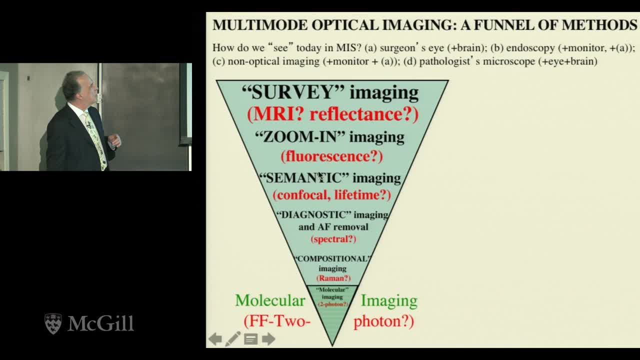 in which you can kind of look, then look, then really look, and then for diagnostic purposes, in very few selected places, you can look with the expensive, difficult methods to deploy. I'm not going to have time to talk about this, but it's kind of fun. 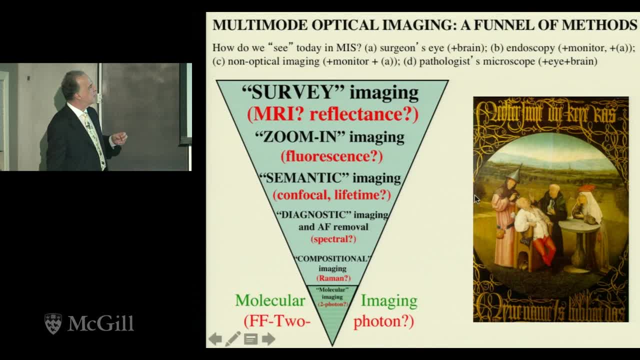 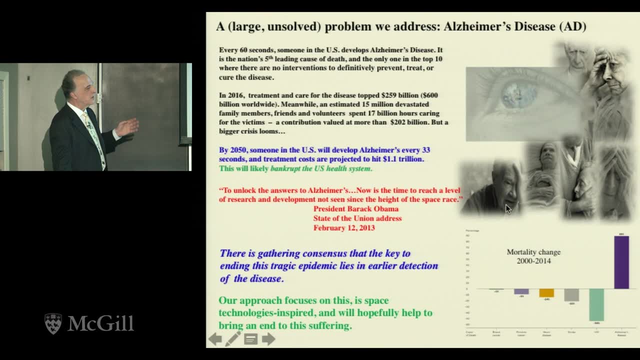 It's a Hieronymus Bosch that hangs in the Prado, And it's the only place where I found a funnel approach to it. This is actually called the Stone of Dementia, So I'm coming to Alzheimer in a second here. OK, 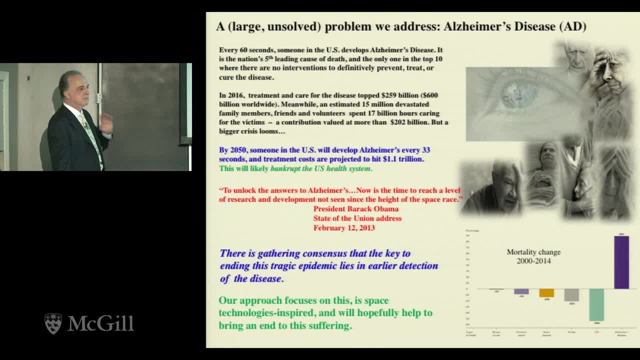 So let's talk about Alzheimer's just to end The health crisis of our generation. no question, By the baby boomers growing up and getting old. in a few years it will become totally bankruptcy-inducing for the health system. Today the expenditures are $259 billion just. 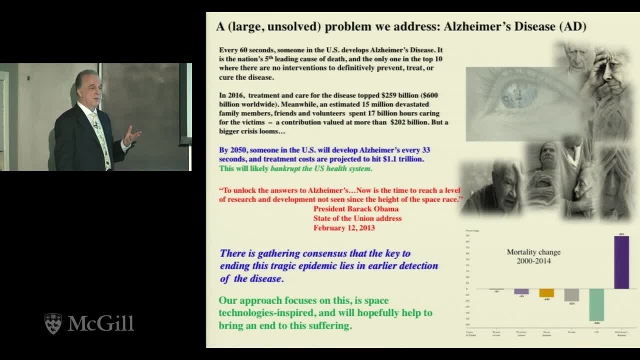 in the US per year and another about $250 billion for the caregiving by family and others. So if you look here, this is really shocking- Out of all the major diseases. I don't know whether you can read this, But it has. 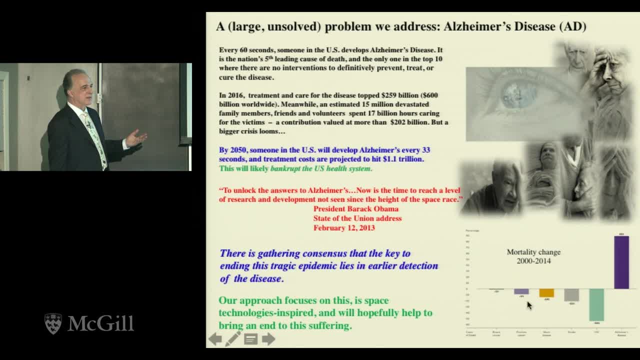 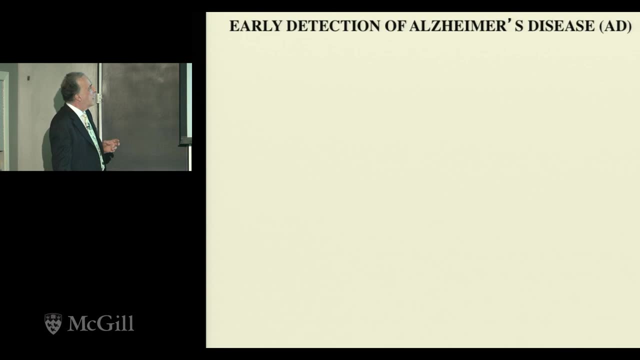 The usual suspects: AIDS, breast cancer and so forth, all on the decline in terms of mortality. Alzheimer's shot up significantly, and even more so the year after this statistic was given. So early detection would be best, as shown here. 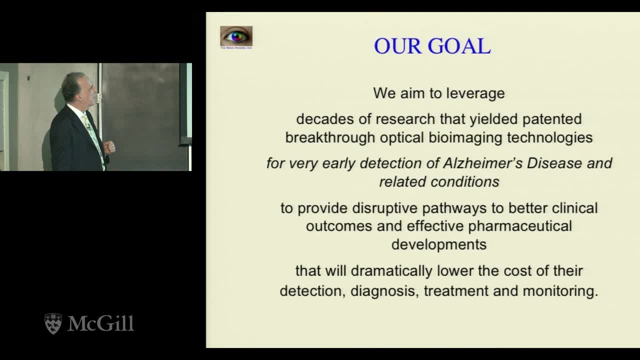 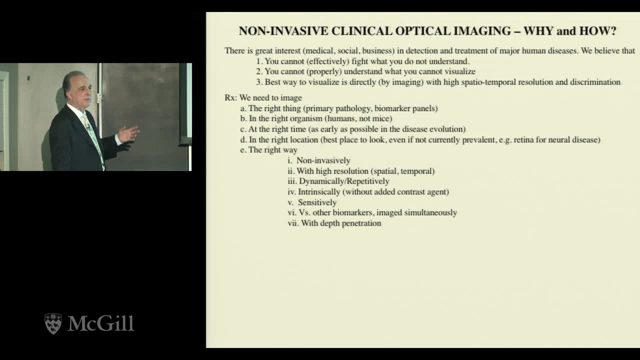 We know this for many years. We aim to leverage what we have learned in order to do this early detection. This is too verbose. I'm not going to take you through it, But basically you would like to. in order to do something cogent, you need to understand it. 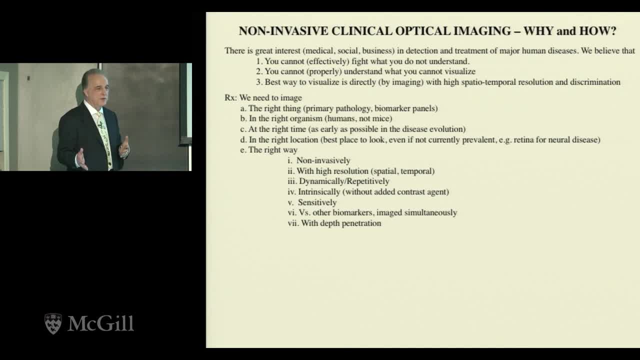 To understand it you need to make a mental picture of it. What's easier for the mental picture than making an actual picture? So imaging is highly recommended, And that imaging better be non-invasive, fast, dynamic, quantitative. do it on the right things. 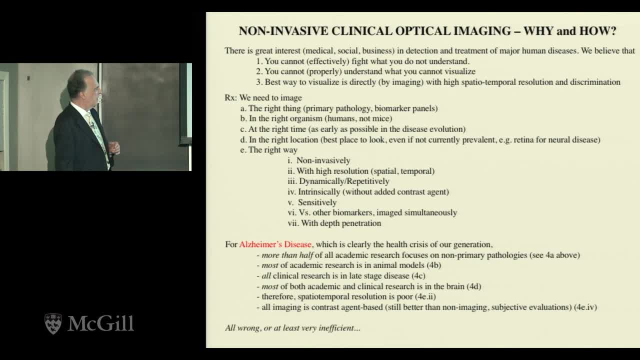 with the right places and also not requiring contrasting. So for Alzheimer's disease, more than half of all academic research focuses on non-primary pathologies. Most of academic research is in animals. All clinical research is in late stage disease, at which point I don't think that much help can be given. 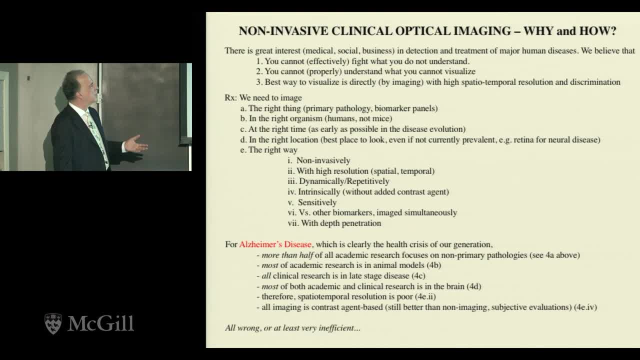 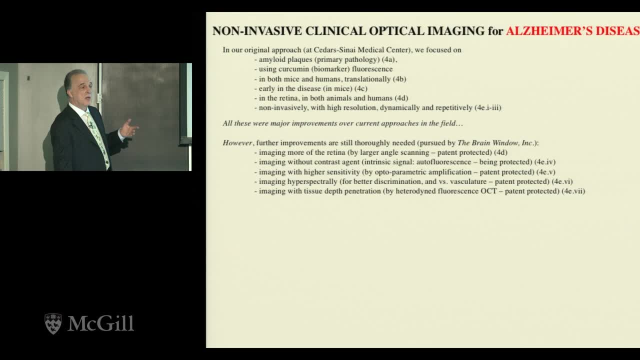 So there are many problems with current approaches. We think that we improved on some of that by basically looking in the eye. The retina is neural tissue. We feel that it's reflective of what's going on in the brain, but it's much more accessible to the brain. 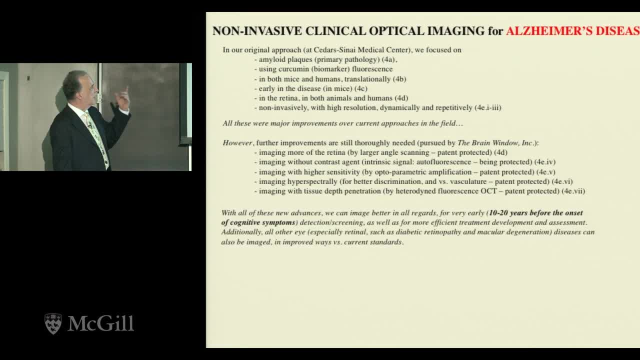 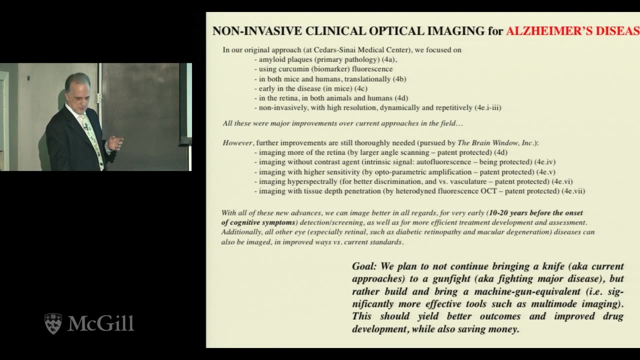 It's much more accessible to optical imaging. So we think that that was the way to go, but it required a biomarker. So very much towards the end of this, I want to show you what you can do without a biomarker. So our goal is not to continue bringing a knife to a gunfight. 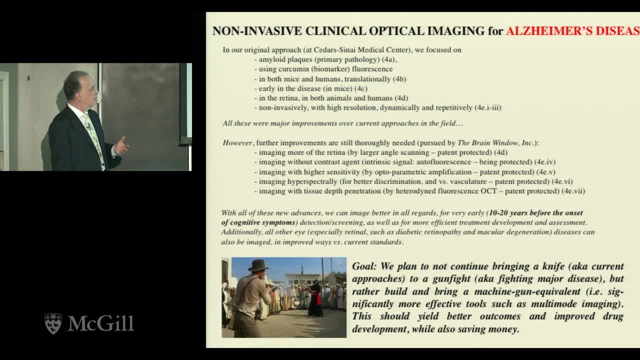 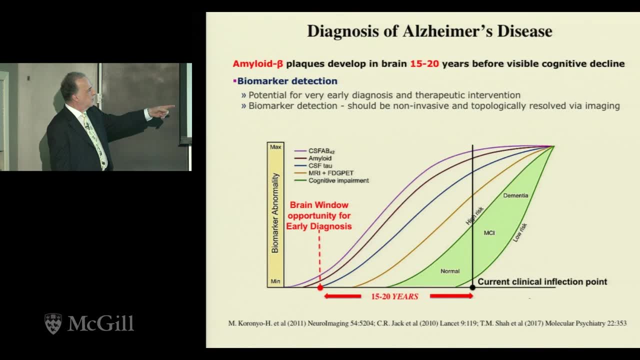 such as current approaches, but do the opposite of that. And you probably all know this scene, so I'm not going to play it, OK, So ideally you want to look 15 to 20 years before you see any cognitive decay symptoms. 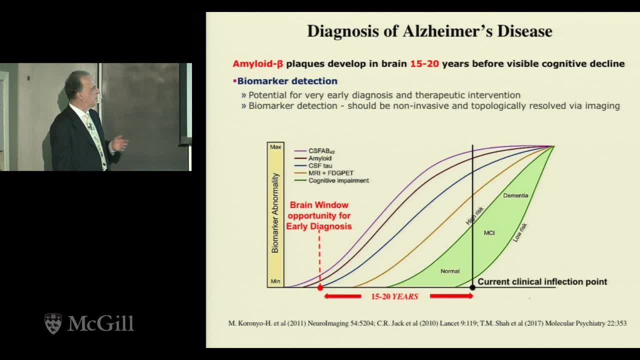 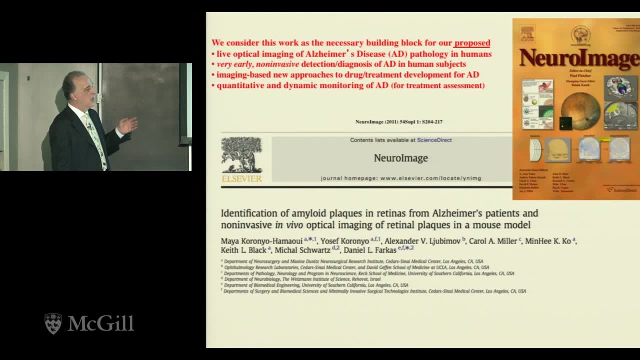 And the only way to do that, we feel, is in the retina, with optical imaging. This was a paper that we published a few years ago and it was a first step towards that goal. This was done in animal models of mutant mice that got very quickly the rise of Alzheimer's in them. 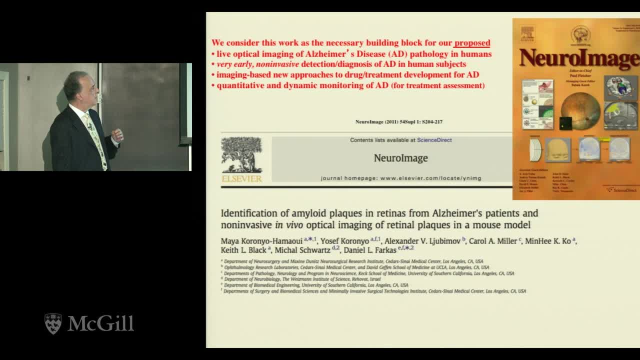 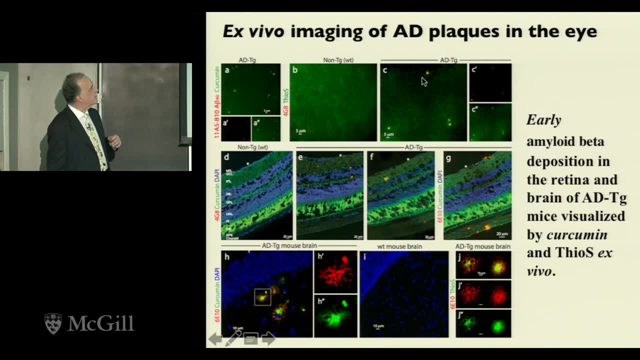 and also on some human archival tissues, And it was done optically. You can see that in the mutants you have the appearance of amyloid plaques. These are the A primary pathology. It doesn't even matter whether you believe in the amyloid hypothesis. 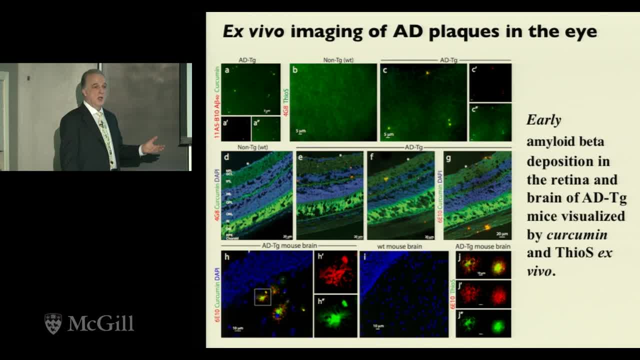 It doesn't need to be causative pathology, It just has to be early pathology. So the same way that if you want to find an accident on the road, it's probably what the people are standing around. They didn't cause the accident. 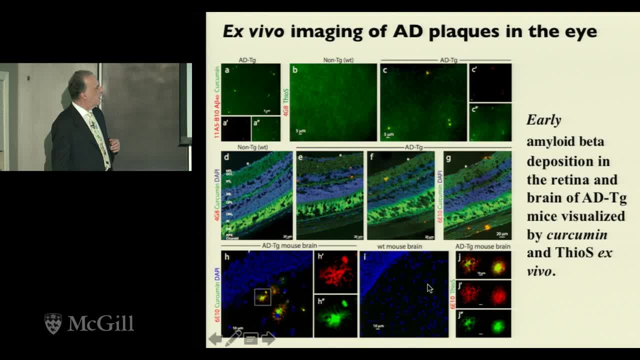 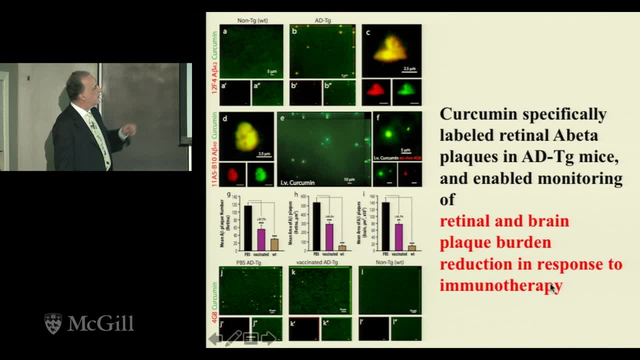 but that's probably what the accident is. So we can confirm that with multiple different controls by antibodies and so forth, we can see actual plaques. You can actually do something about them with some immune treatments and also you can look in living animals. 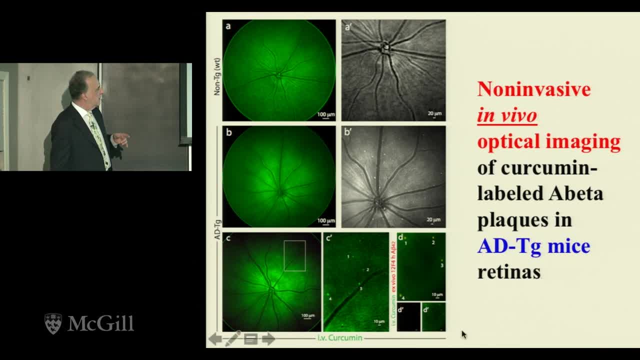 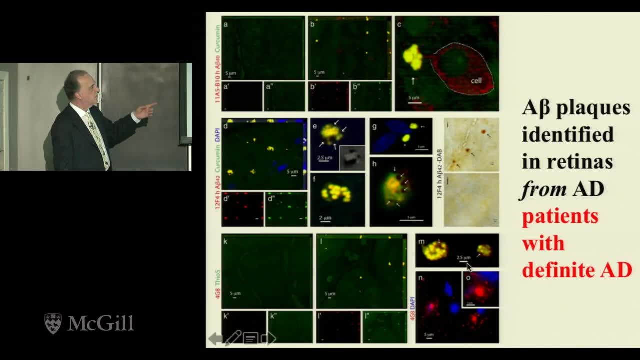 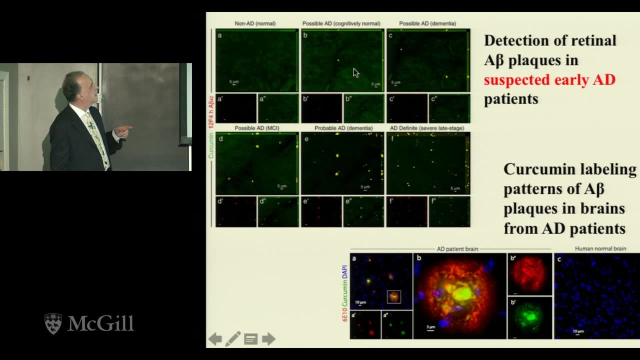 This was the first time that this was ever done and we can see the plaques. We could see the plaques in living animals And also in patients who had definite Alzheimer's and even in patients that had suspected Alzheimer's- and obviously less plaques, but still. 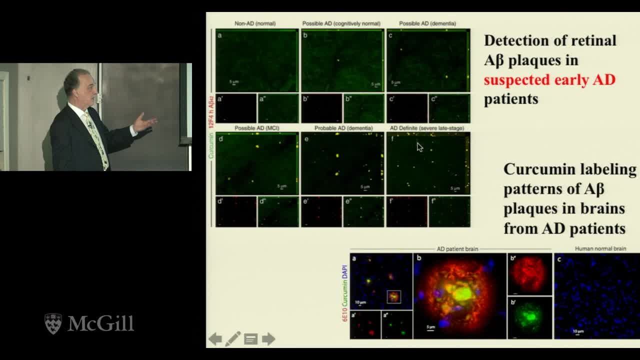 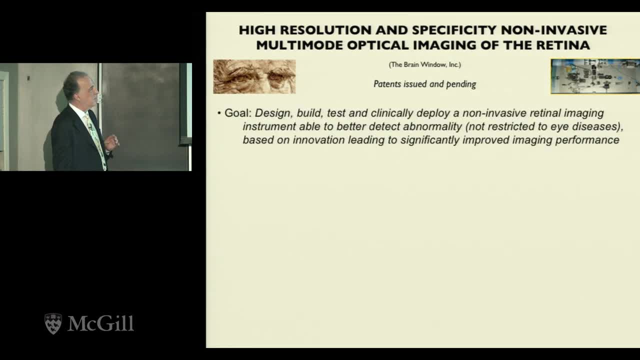 And you could match to the temporal evolution. This is not a large study. We didn't have the resources to do a large study, But instead of talking about the large study, let's talk about what could be done. that would, in my opinion, enhance this. 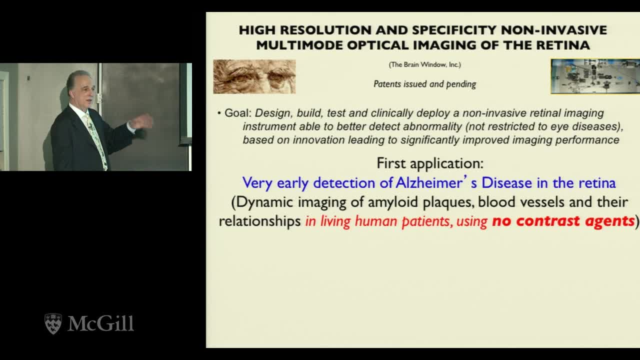 Let's look, not with contrast agents that you add in because you don't know how well they can target and you don't know how well you can image them. This was a good contrast agent called curcumin. We want to do it without contrast agents. 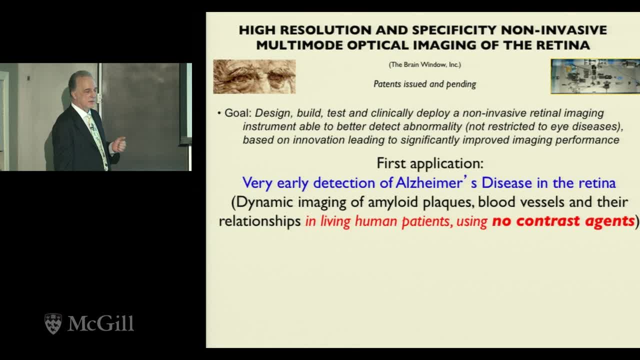 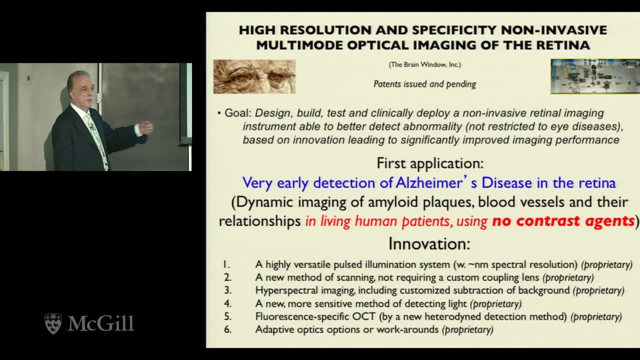 It turns out that the primary pathology molecules the amyloid plaques and the monofluorescence autofluorescence. So for that you need a large number of new technologies, Because you need a more sensitive system. you need a system that looks everywhere in the retina. 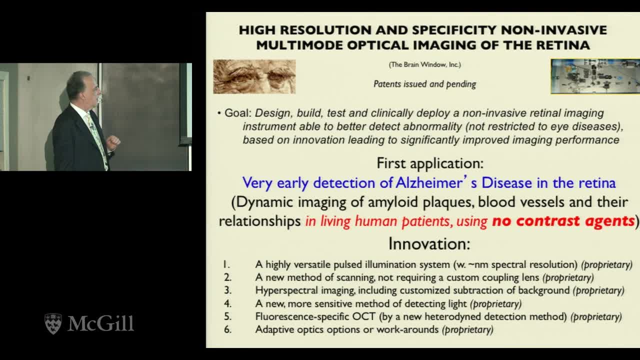 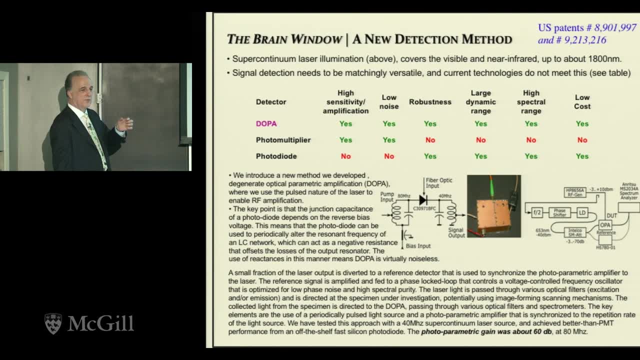 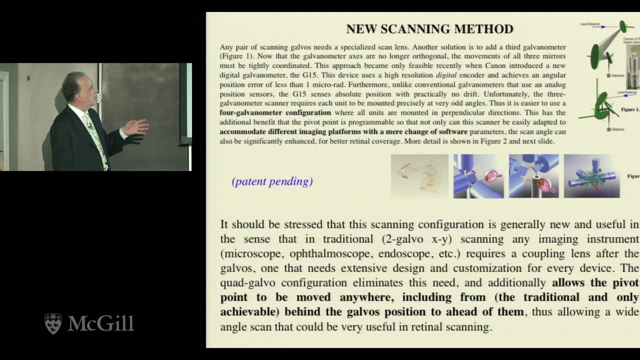 not just in the middle and so on. So we have a new kind of detector. It's patented. It's basically turning any photodiode into something more sensitive than a photomultiplier for detecting low photon fluxes. We have a new way of scanning. 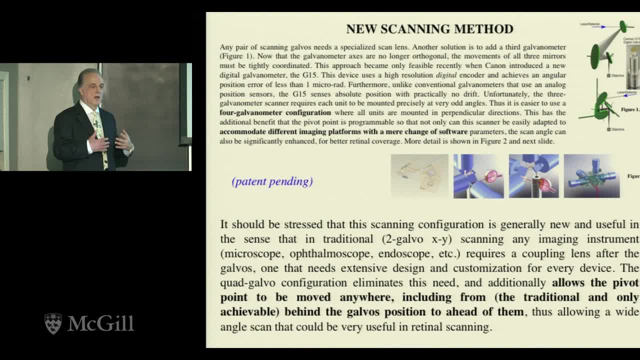 which involves concerted quad galvos, four galvos that are very precise in their positioning. That allows you to take the pivot point of the scan from the mirror or behind the mirror, like in all other scanners, and put it in front of the mirror under computer control. 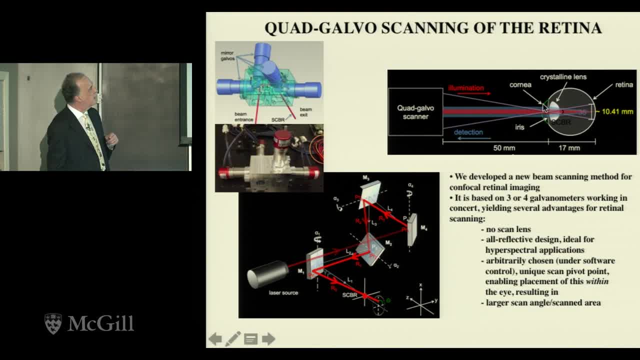 including putting it at the entry of the eye, so therefore you don't need to dilate the eye. You can cover a larger area of the retina- And this is being patented- And eventually develop a multimode hyperspectral ophthalmic scanner that looks at the retina. 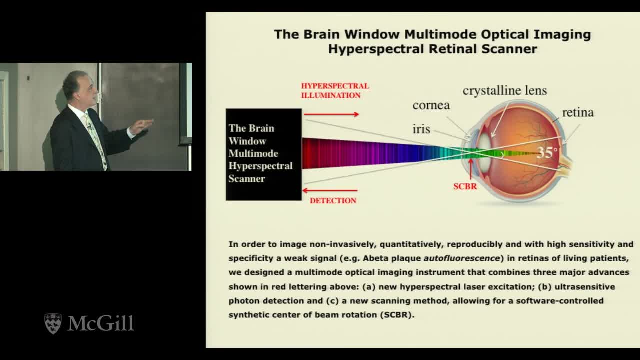 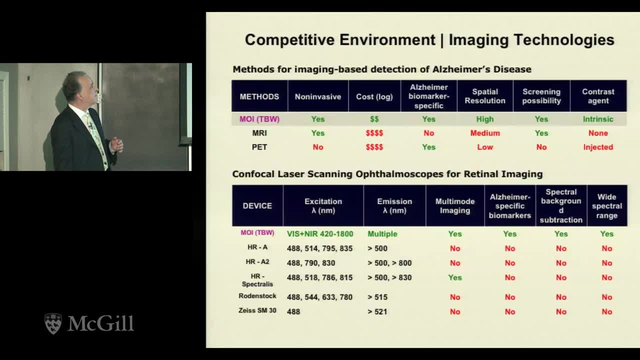 not only for these amyloid plaques- autofluorescence- but also for correlated things that you would like to know what is happening to them, such as vasculature. Comparison with other methods of imaging: This is our method, compared with MRI and PET. 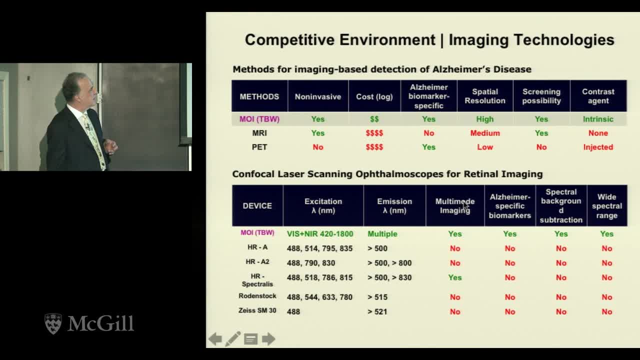 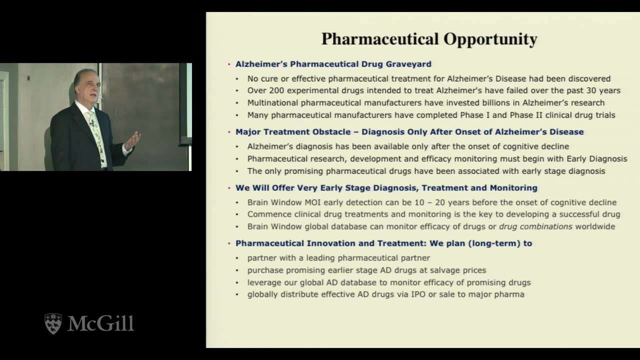 so you see the advantages And compared to other confocal laser scanning ophthalmoscopes, it's basically a little bit more versatile and covering more of the retina, More of the desired features, And there's a pharmaceutical opportunity, because about 99% of all 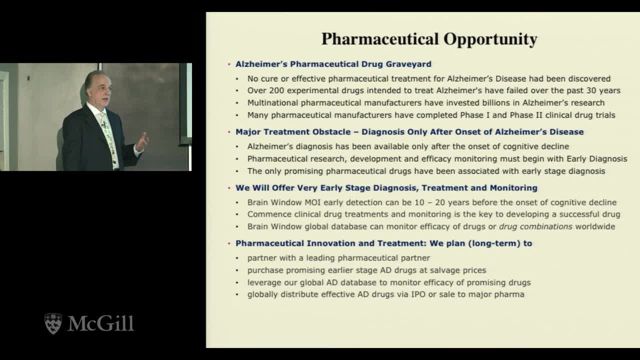 candidate drugs for Alzheimer's have failed. but in our opinion they have failed because they try to do something to late stage patients which really are beyond help, I think. So if you can do early detection, then you can probably do better. So the fact that there's an opportunity there, 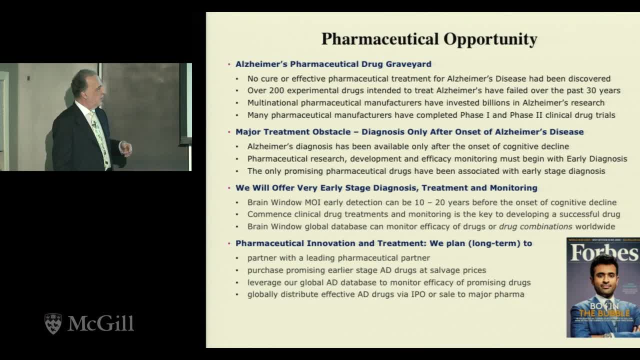 is pretty obvious and logical. but if you don't believe me, this gentleman, who's quite young- younger than my son, actually- he made it to the cover of Forbes by going to one of the pharmas and taking one of the failed drugs. 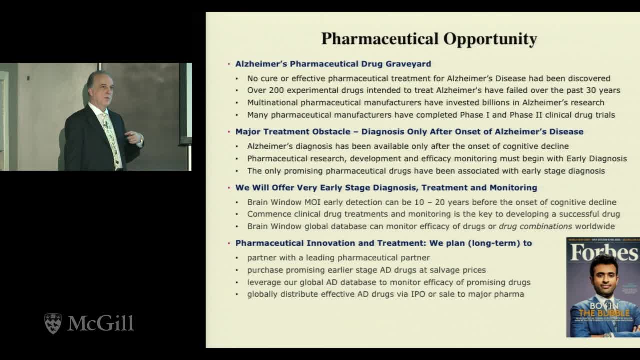 He bought it for $5 million and I think he IPO'd about less than a year later for about $5 billion, because there was hope that that one would actually be useful. Okay, I'm not going to talk about this. Optical coherence tomography is a beautiful method. 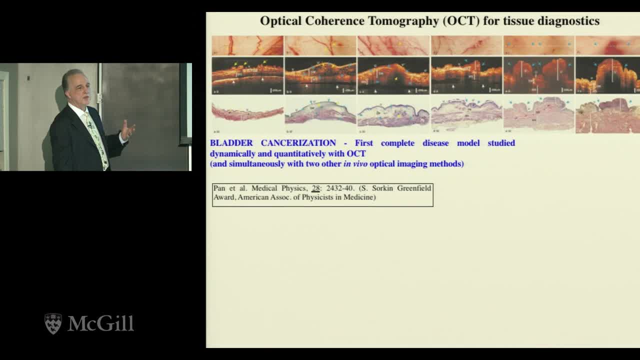 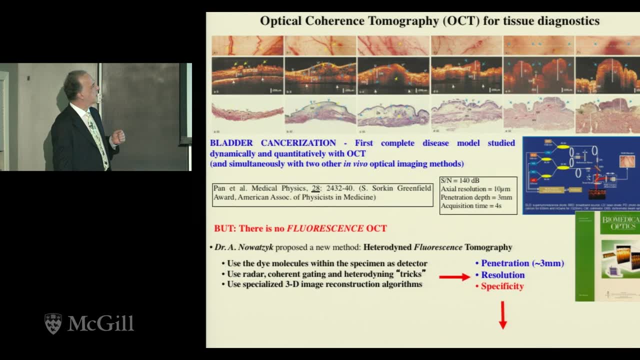 You would like to use it to look in the eye, but it doesn't have the specificity of fluorescence. So Dr Novacek, that I mentioned before, came up with a method of making fluorescent OCT, but I didn't bring the figures. This is the last slide of data. 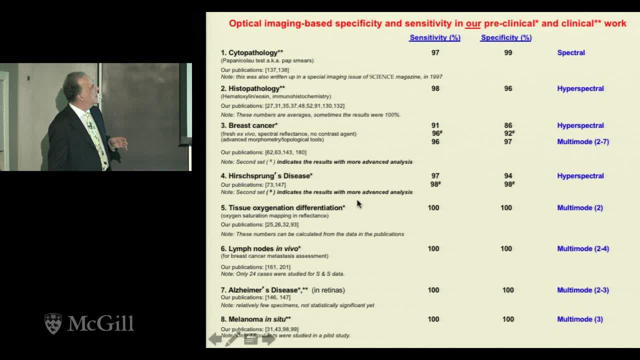 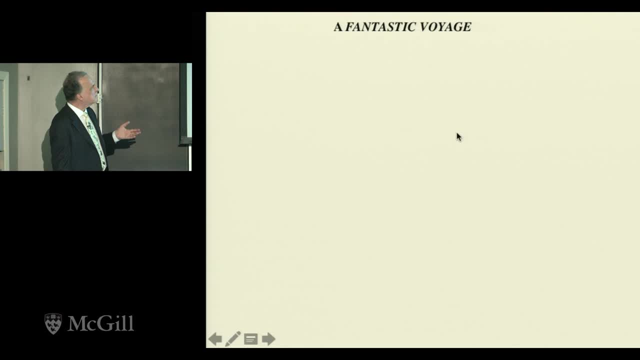 If you take the multi-mode approach that I was advocating, no matter what it is that you're looking at, you can do very well in sensitivity and specificity. So, to conclude, if the people of a certain age in the audience may remember this, 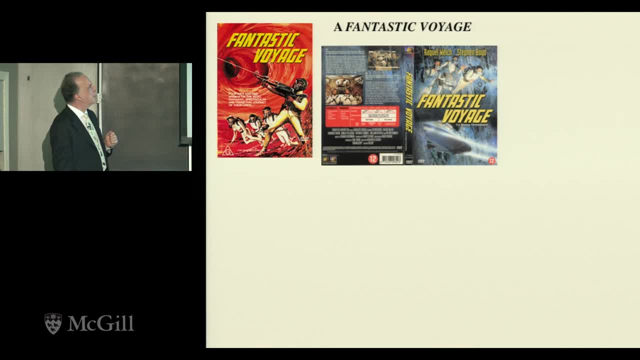 maybe the younger people don't. it was a very memorable science fiction movie in which an interdisciplinary team of scientists was miniaturized and injected into the bloodstream of a government scientist who had a major problem in his brain, And in a little submarine with lasers. 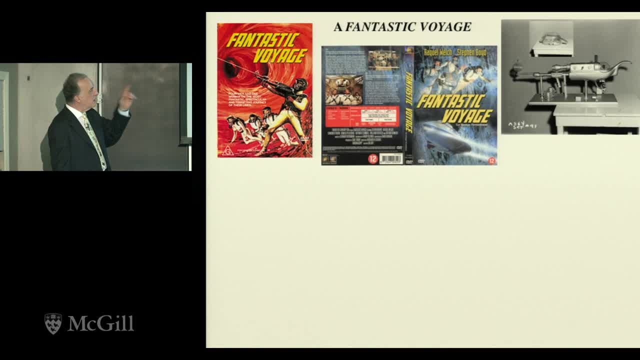 so at the time- this is the mid-60s, lasers were young. so I actually living in LA, I actually went and tracked down the prop that was the laser. Raquel Walsh was in it Looks like antiquated technology. 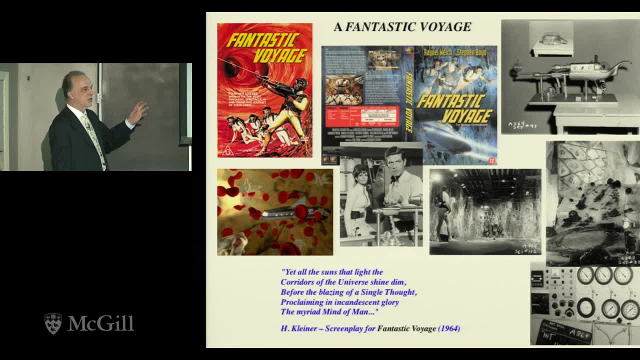 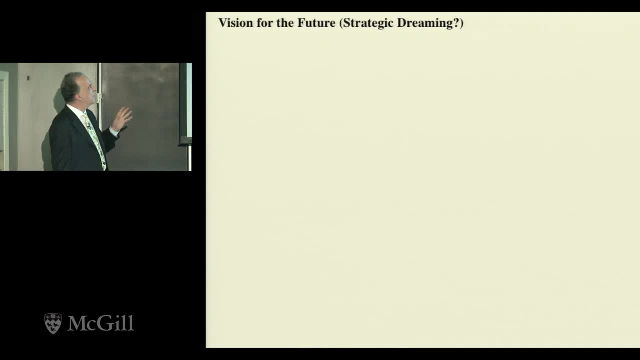 but the idea was very clear that you can do intervention with lasers and in a very kind of guided way. So for my concluding slide here, a vision for the future. The best way to predict the future is to create it. If you are a physicist. 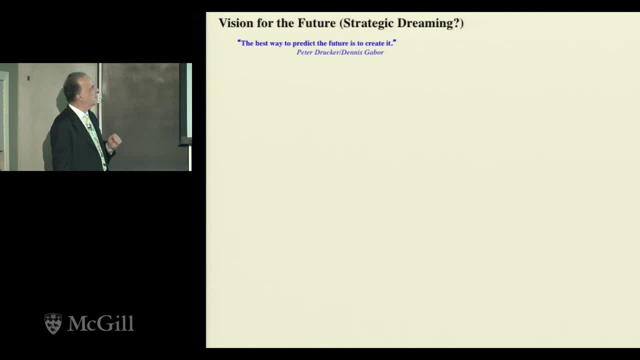 you think that Denis Gabor said this. If you are a business type, then you think that Peter Drucker said it. So here's Mr Bacon, that we mentioned technologically updated, and he told us that it would be madness and inconsistency to presume. 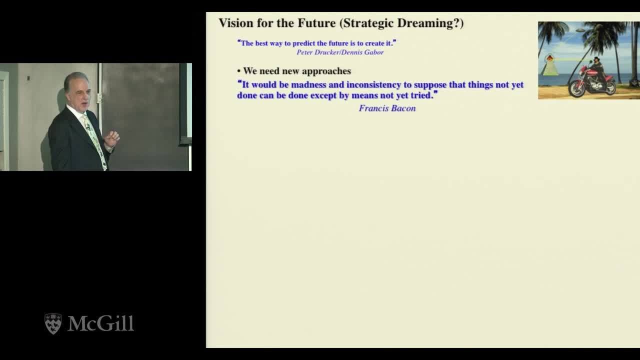 that things not yet done can be done except by means not yet tried, which sounds even more contorted in the original Latin, but is basically calling to arms to develop new technologies and new approaches. But, people, new tools are not everything, because men have become tools of their tools. 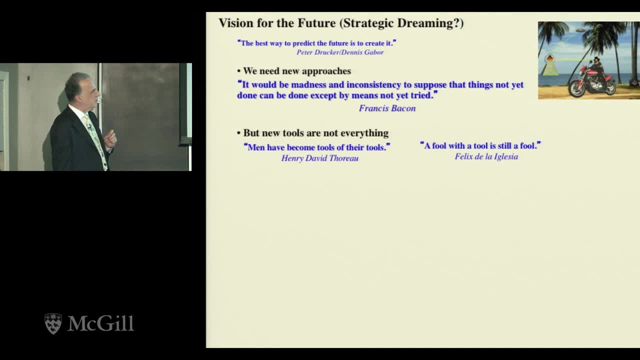 and my old friend Felix de la Iglesia is saying that a fool with a tool is still a fool. Yogi Berra the sage is telling us that if you come to a fork in the road, take it. So, in terms of methods of imaging, 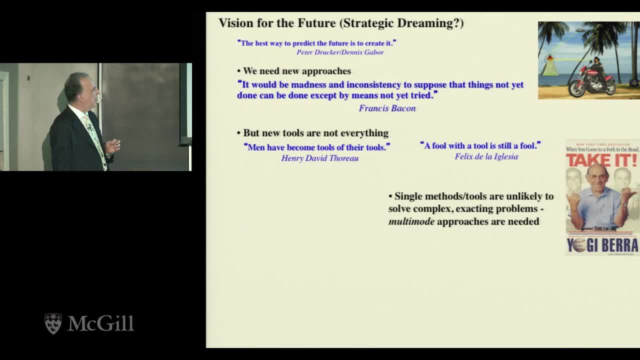 we are advocating multimode. Let's take that fork. And William Gibson, another science fiction writer, is telling us: the future is already here, but it's just not evenly distributed. And I would like to leave you with a quote from Christine Peterson. 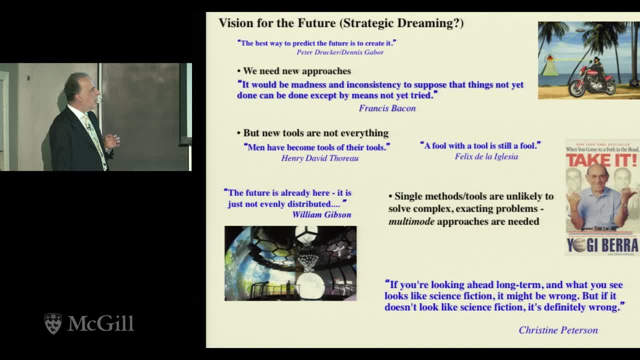 who is one of the founders of nanotechnology, And she said that if you're looking ahead long term and what you see looks like science fiction, it might be wrong, But if it doesn't look like science fiction then it's definitely wrong. 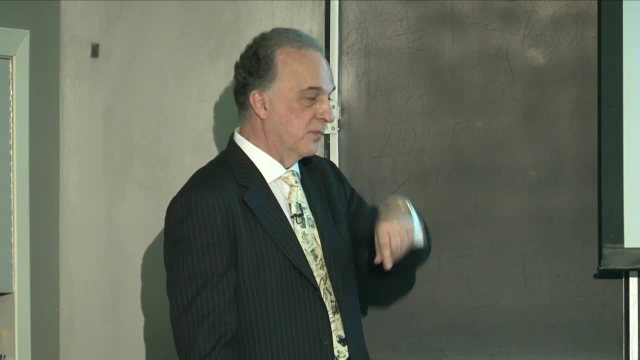 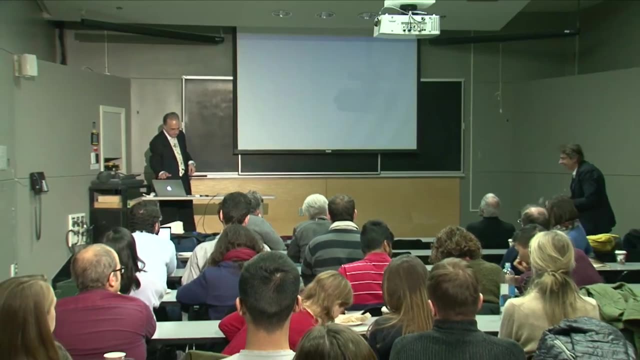 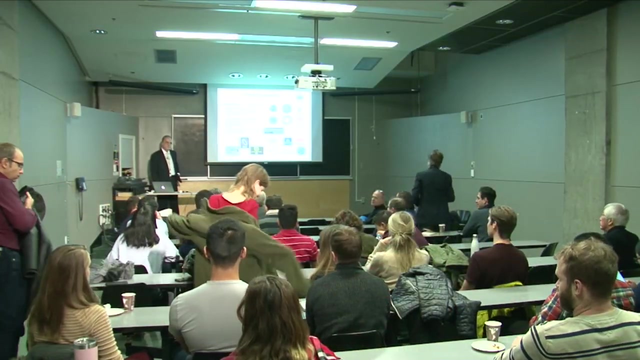 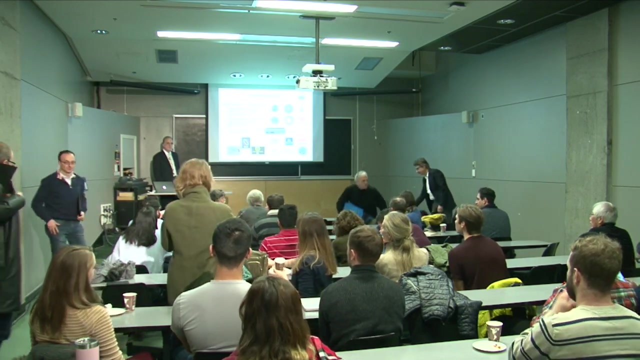 And additional acknowledgements. Sorry that I ran long, quite long. Thank you very much. Very interesting talk Questions. Thanks for the talk. Many possible questions, but there's one particular thing. You had a slide where you had breast cancer and comparing your spectral images. 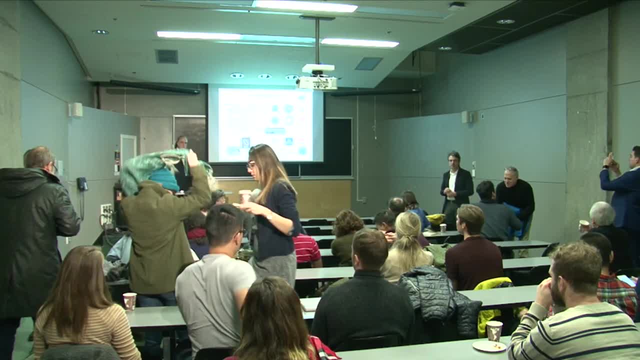 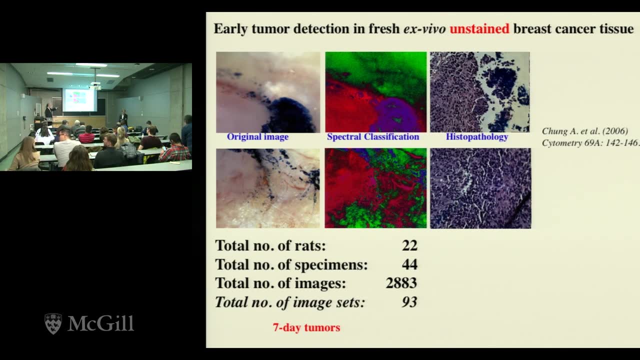 with histology, histopathology images, And I was just wondering if you can go back to it and explain what we're seeing. Sure, So we were marking with a marker the locus, because we were not really firm in what exactly we wanted to see. 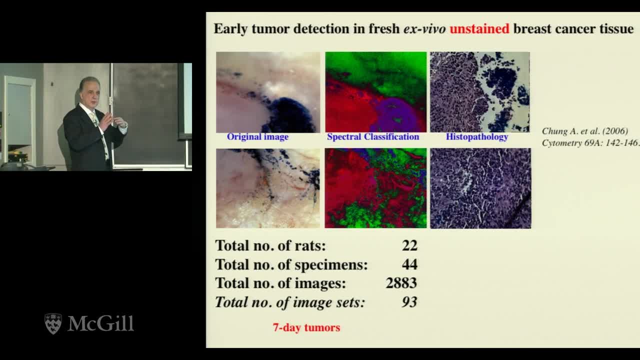 in order to preserve it in the same orientation with histopathology. So the dark blue stuff, that's just a marker. Okay, What we were characterizing by spectral imaging were pieces of tissue that looked the same to the naked eye and then take the histopathology of it. 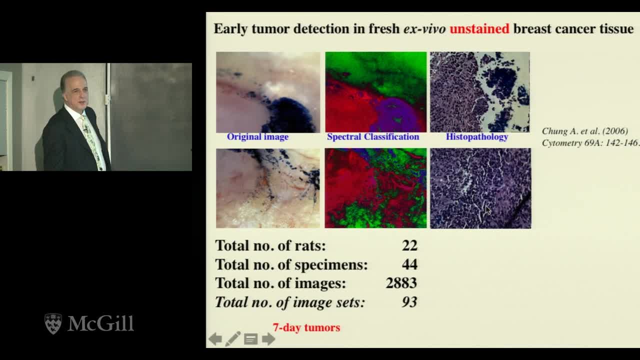 and actually I don't have the animation, but we had to zoom in on the histopathology. So just by pure spectral segmentation we were finding regions marked in red that were cancer versus normal, which did not look different to the naked eye And then confirmed by histopathology. 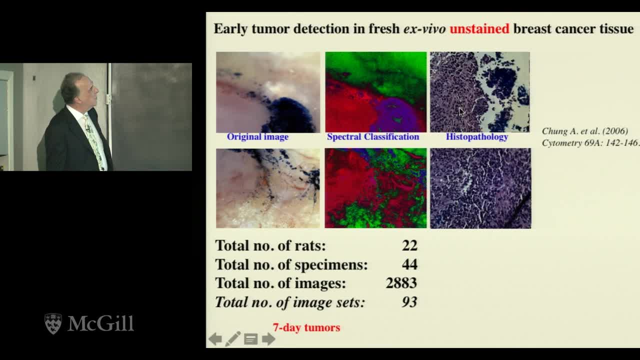 Okay, but histopathology images are not the same field. Well, as I said, I had an animation that it was actually the same field and this is a zoom in on the field. Okay, right, I didn't bring that animation. 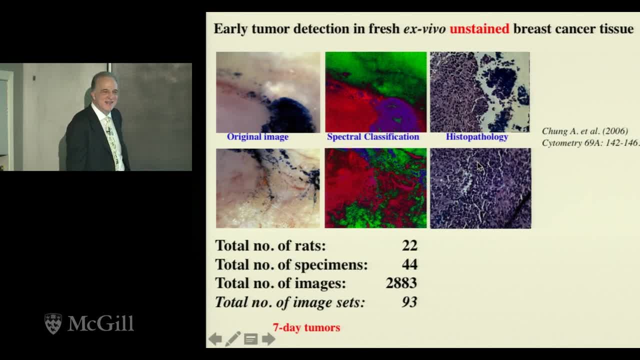 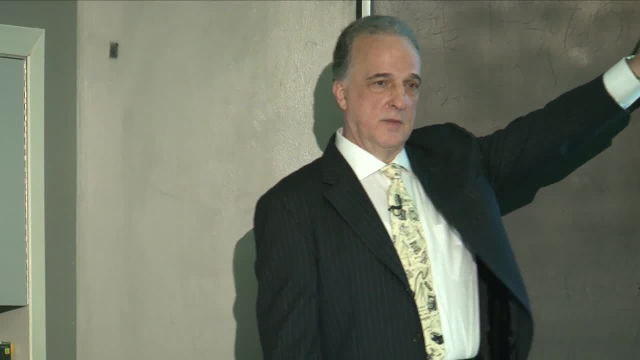 You know, animations usually don't work in the end. Yeah, sorry for that. But the other breast cancer one was a little bit more interesting because it was a breast cancer that was actually away from the field and it propagated through the ducts and it was very different. 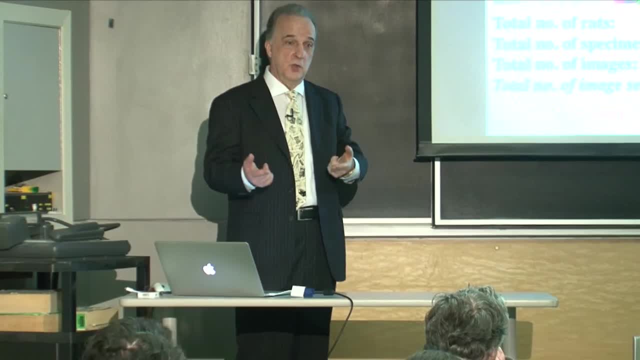 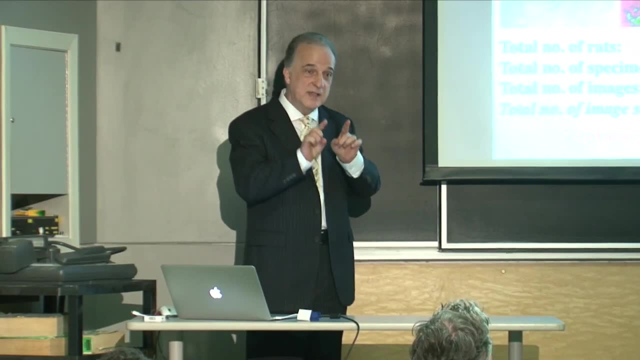 It was very difficult to find by regular histopathology and therefore they had to deploy immunohistochemistry. And we were able, on the regular histopathology on the H&E, just by spectral segmentation, to find exactly the same areas that immunohistochemistry found. 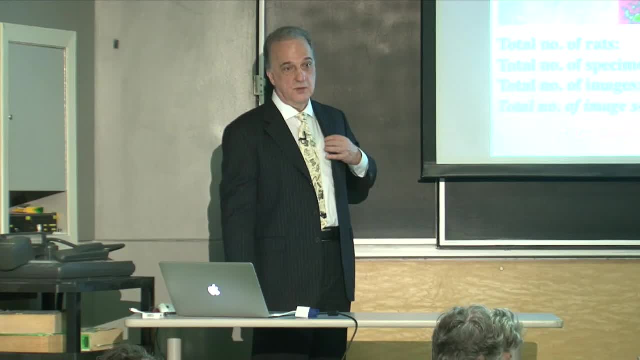 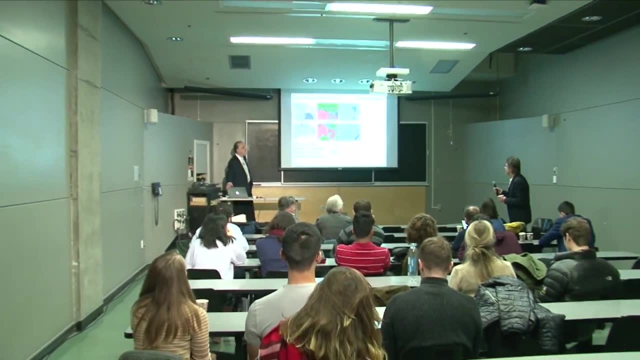 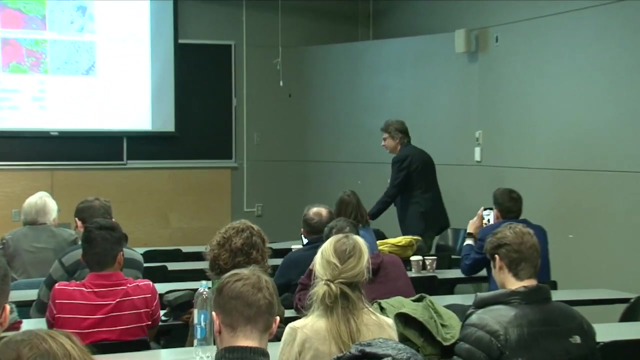 that obviously needs additional staining and time and so forth. Okay, any other questions? I have a quick question On the spectral ME scattering. Yes, You mentioned at some point that you need higher resolution. Yes, How high the resolution are you talking about? 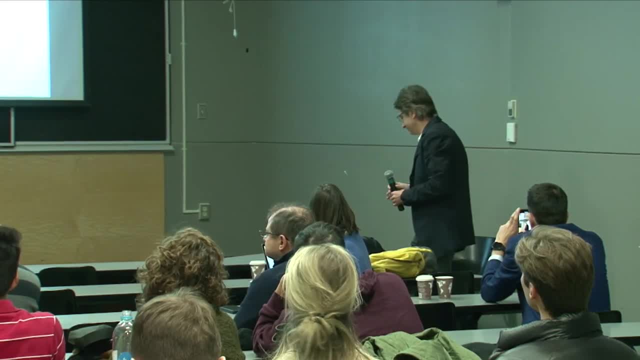 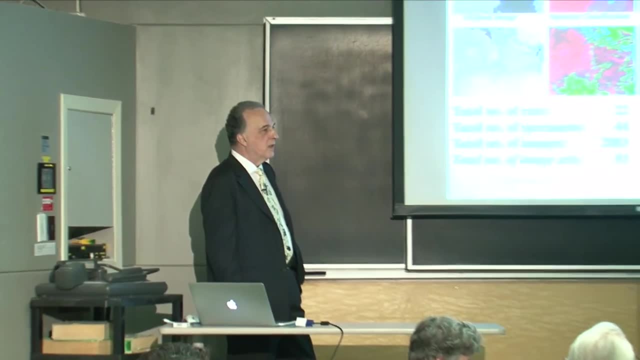 I mean, does this change in? We estimate that it has to be sub-nanometer, So not severely sub-nanometer, but In response to what sizes for the ME scatters? Yeah, based on the modeling if you do it in the visible. 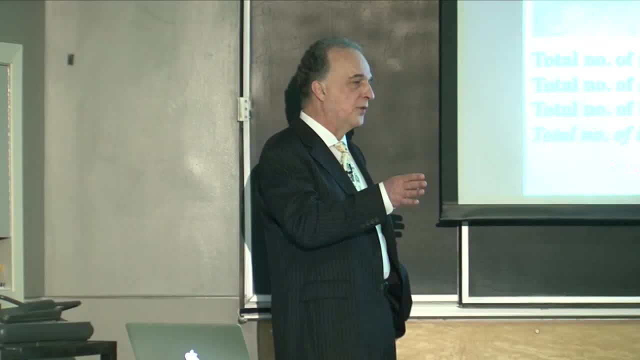 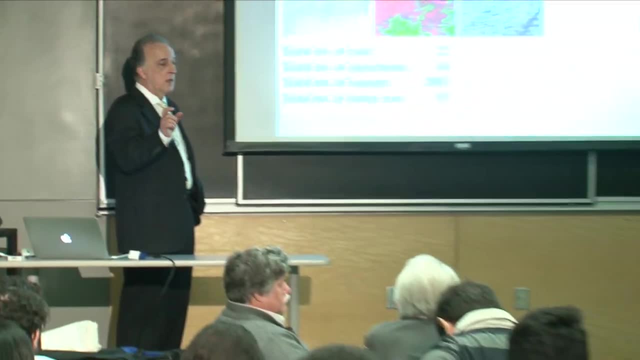 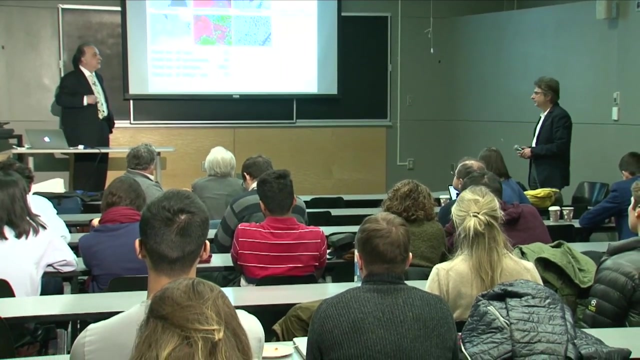 this is going from roughly 1 to 2 microns to 6 microns. That covers dysplasia and early cancer. If you go a little bit further out into the near infrared, the oscillations become more pronounced. So therefore, to pick up those oscillations, 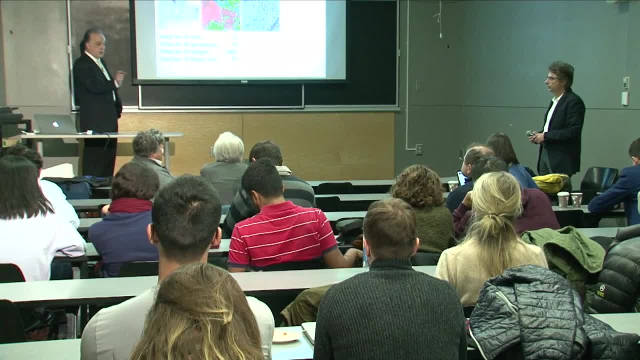 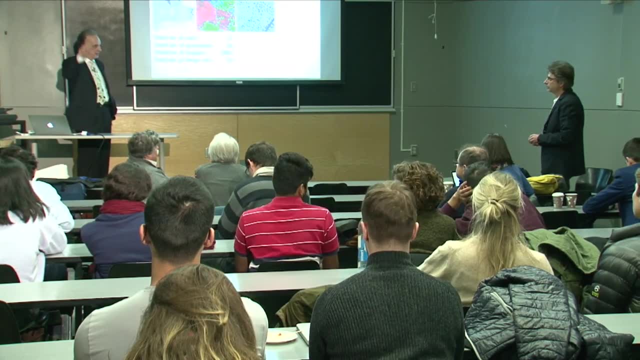 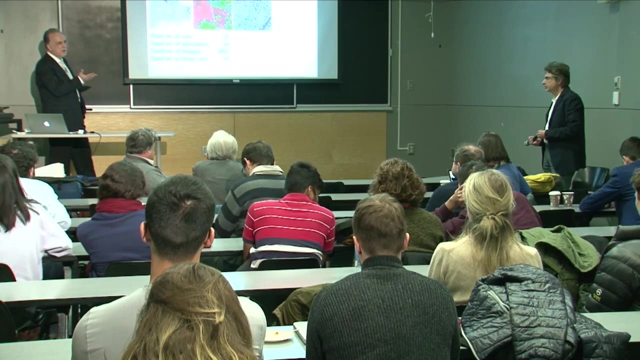 you really can benefit from the, But you can use a smaller spectral range because the oscillations, instead of being like this, they start being like that, And so we modeled that, but we also have seen that. So this particular system had about 0.1 nanometer resolution. 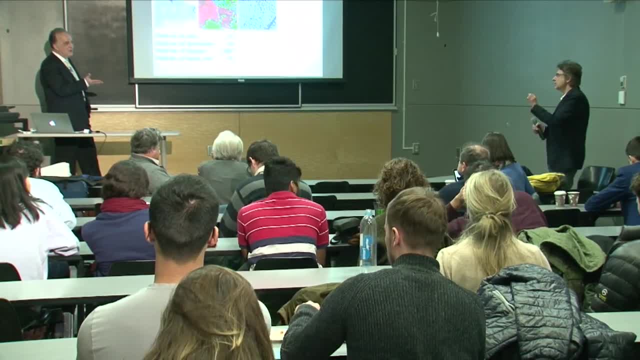 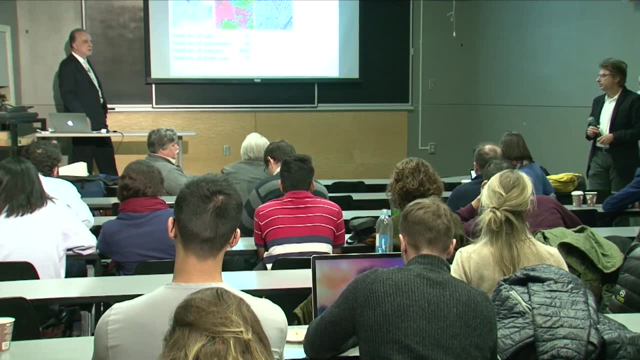 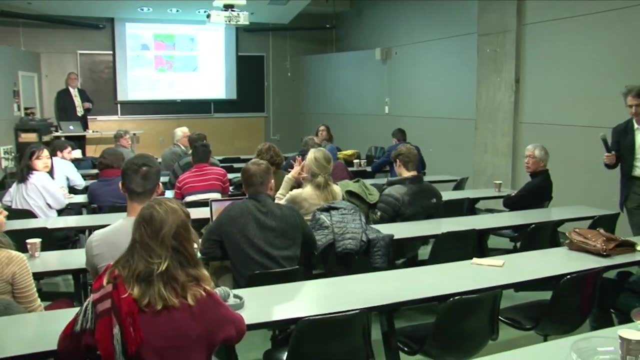 but obviously starved for light in that case. So also to see sizes of 1 to 3 microns, give or take. 1 to 4 microns, Yeah, Okay, Other questions? Yeah, Hi, thanks for the talk. 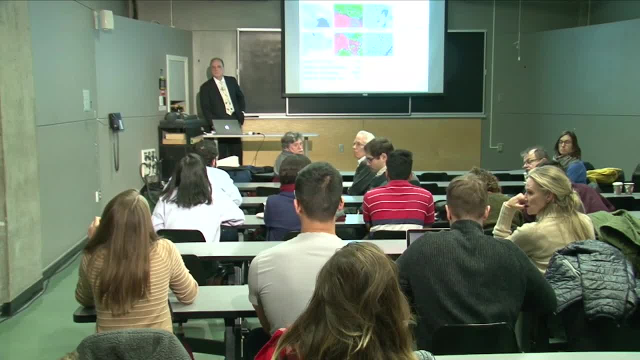 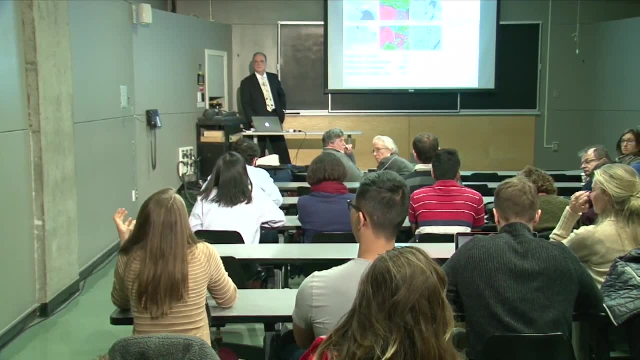 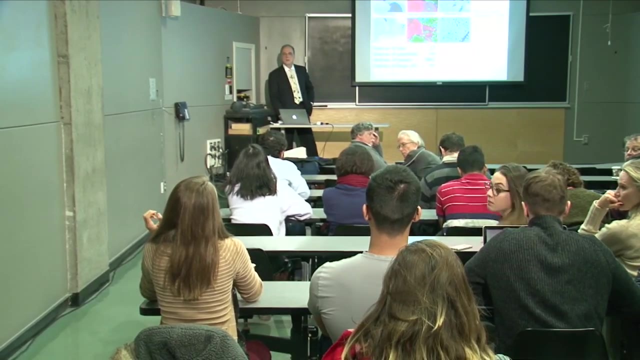 I actually had a question about your work that you do with Hirschsprung's disease. So the transition period is basically defined as basically the presence of these nerve cells within the muscle layer of the gut And the reason why it's so difficult. 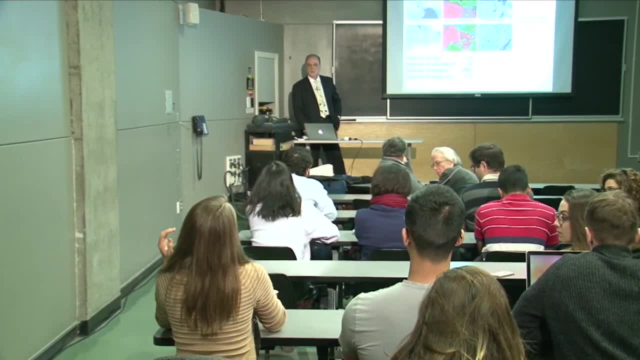 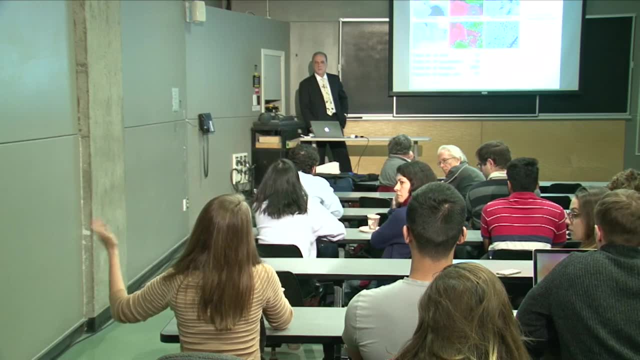 to determine where to cut is because we want to know what, I guess the threshold or the magic number is for the presence of these nerve cells that will basically facilitate gut motility. So my question is: with the spectroscopy that you do, 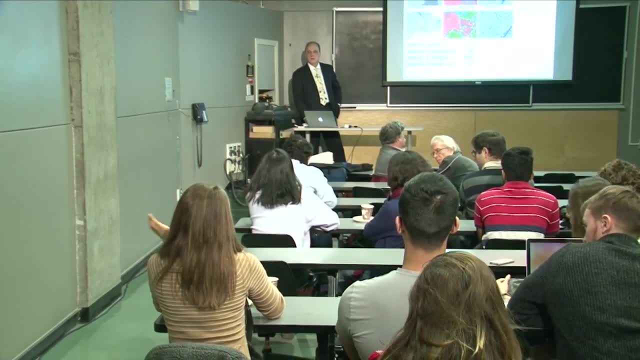 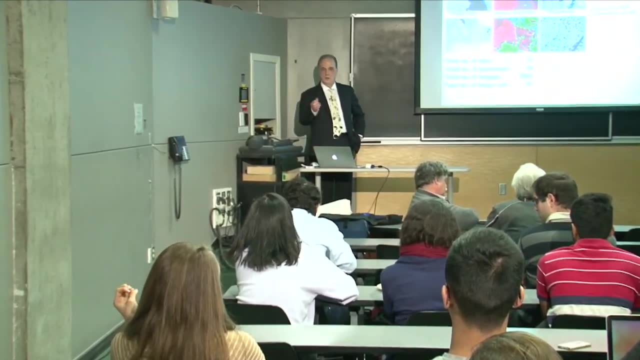 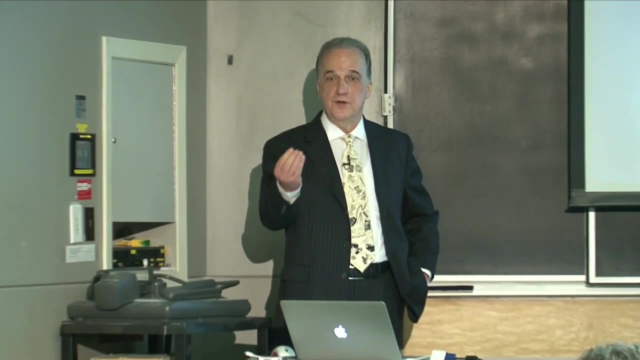 I'm assuming that you are looking at the waveform of these nerve cells and if you found this threshold. Well, actually we did not look mechanistically for those specific nerve cells. What we looked for is the tissue in its spectral signature being different from normal. 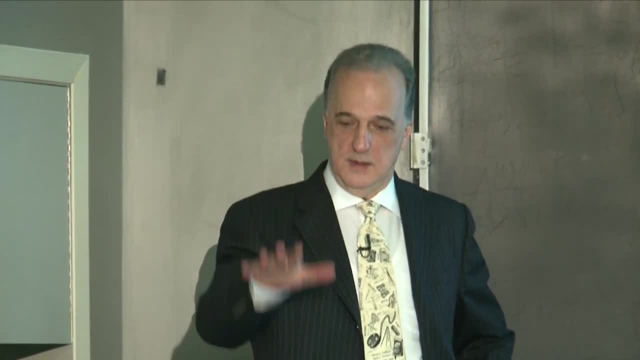 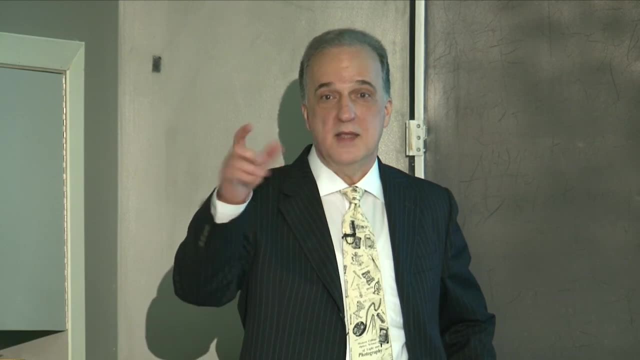 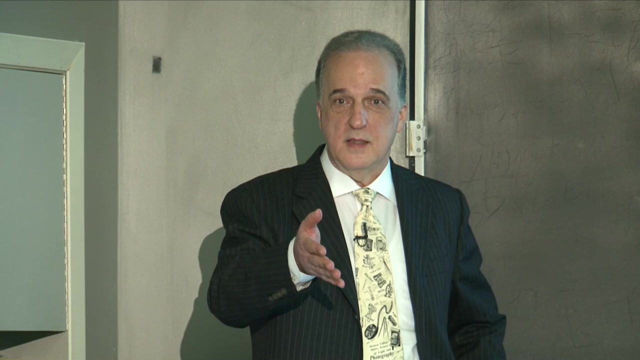 And, as you could see, there's a region where it's quite visibly- I mean not visibly- quite reliably- different from normal. But then, as in all things in nature, there's a transition where some of the tissue is aganglionic and some of it has ganglia. 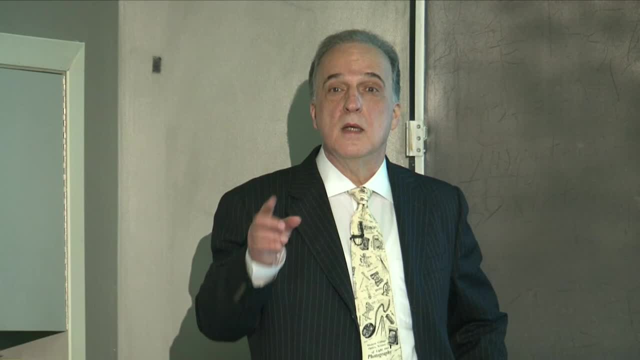 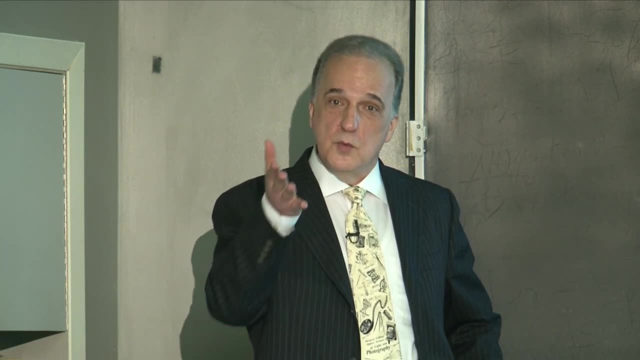 And I think that, at least in my guess, that region probably changes even within a couple of days until the intervention is done. So what you would really want is to be able to do the characterization, which in certain ways it's almost agnostic. 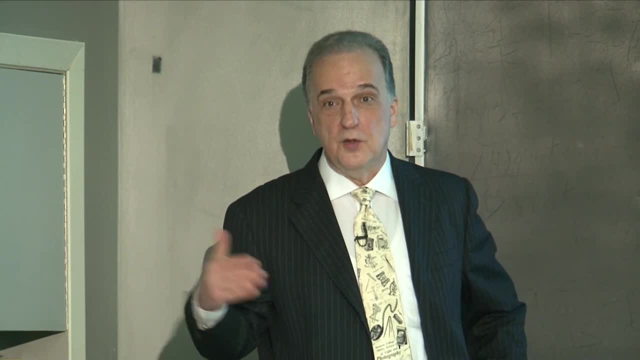 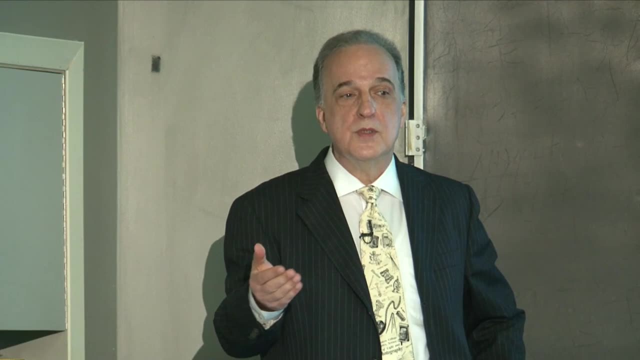 as to what the reason is for the discernibility of the difference. So we are not drilling down to the level of neurons firing and you know the ganglia working and so forth. It was just requested by the surgeon that is presented with this. 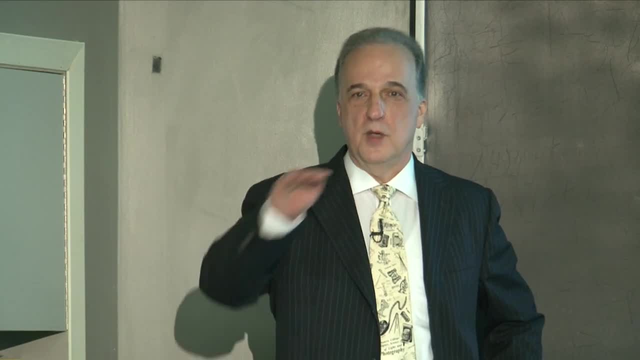 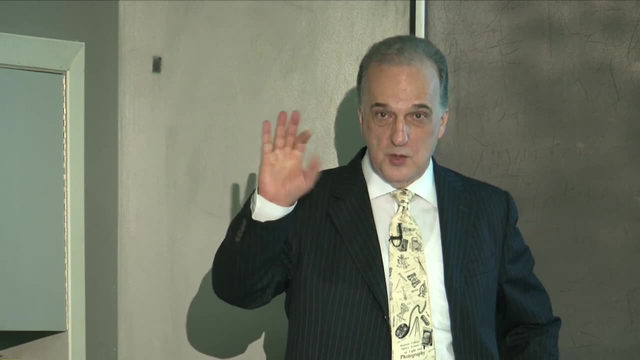 on a daily basis. Can I be a little bit more confident about where it is that I'm cutting? So you're not going to cut below the transition region. You're going to cut probably above the transition region to make sure that what remains is all healthy.